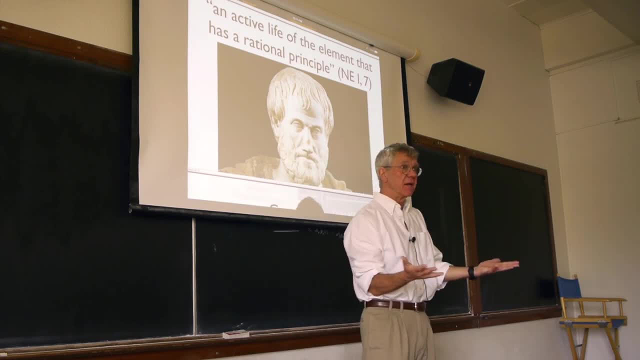 that differentiates us from lower forms of animal life. I think dogs, cats, raccoons, etc. actually have some degree of rationality. After all, they can solve problems, They can figure out things, They know when it's time to be fed. 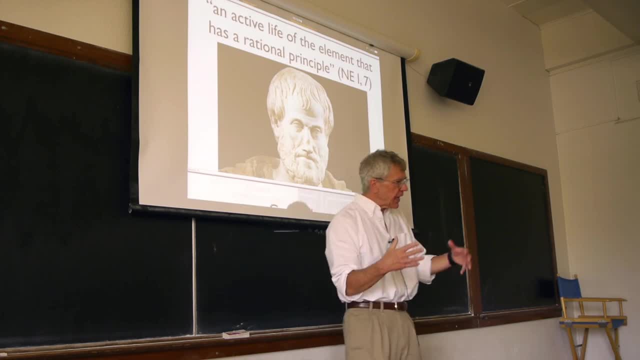 On the other hand, it seems to me that there is something that is distinctive about human beings: We're capable of constructing rational plans. If I say what's your plan for the next four years, you can maybe give me an answer. maybe not, But at least you can consider. 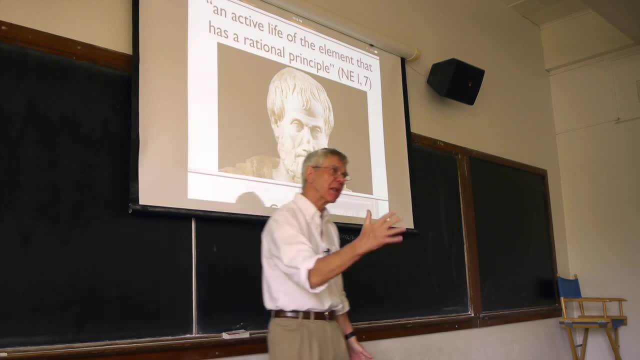 the question right? You can't do that with a dog. Well, what's your plan for the next four…. I mean, the dog doesn't know what his plan is for the next hour, let alone for is for the next several years. 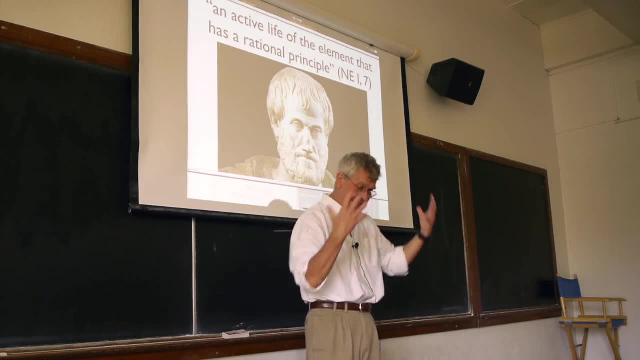 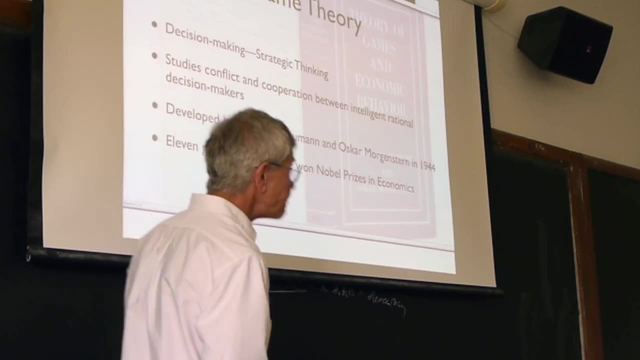 So the complexity of human planning, of human activity, is far greater. Now, what is involved in all of that? Well, at the very least, decision making, And so game theory is, from one point of view, the theory of decision making. 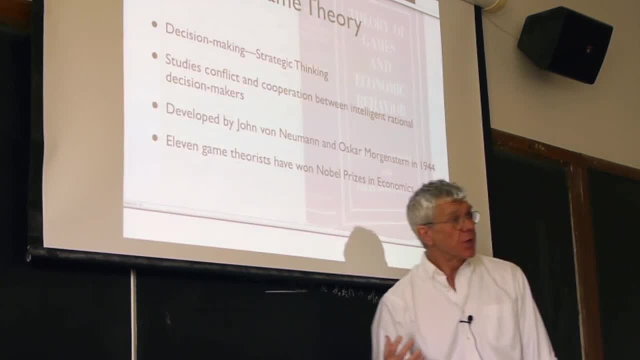 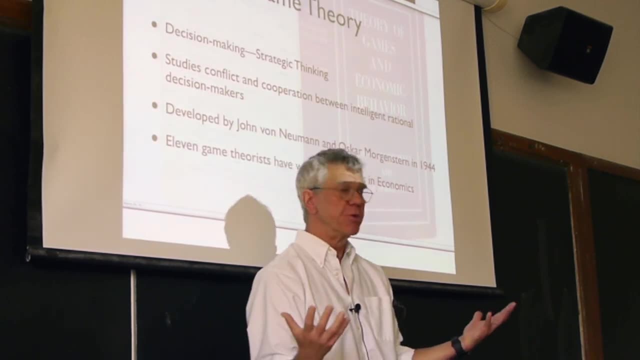 How do we make decisions, How do we formulate strategies? So it's really all about strategic thinking. Now, it's unusual to put this in an ethics course, because you might think: wait strategy? Well, there's an obvious connection, right. 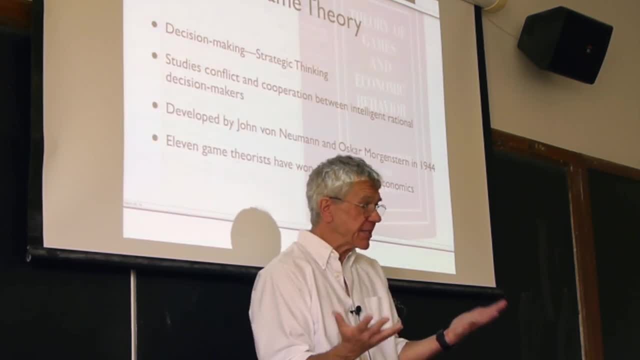 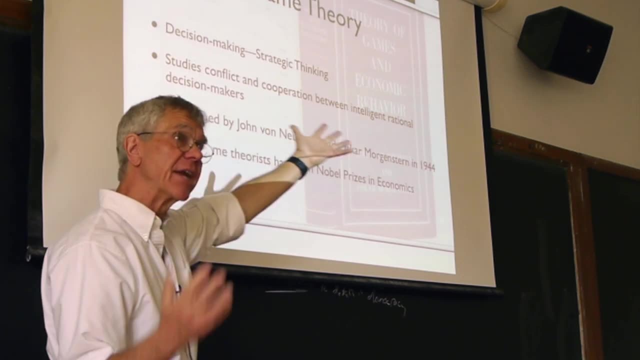 Strategy is how you should go about addressing a problem. Ethics is about what you ought to do, how you ought to make decisions. So there's an obvious overlap here. There's a connection between strategy and ethics in a way that I think people often ignore. 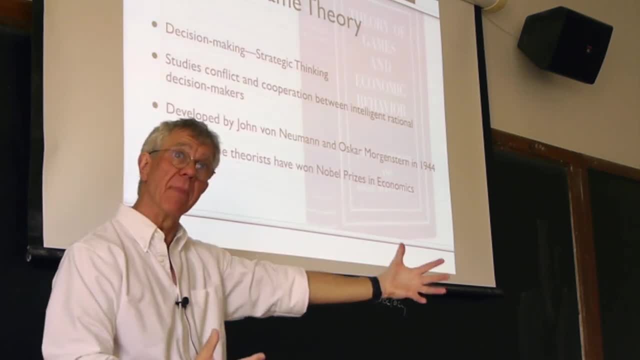 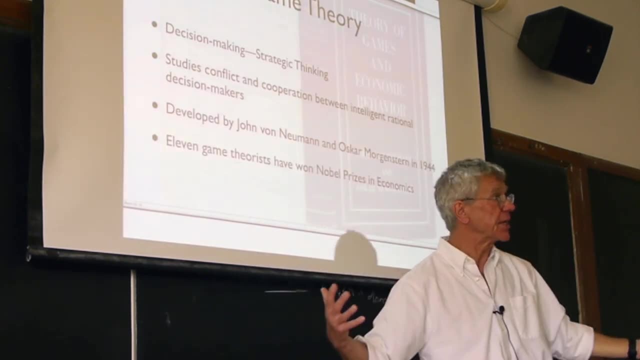 We always are deciding upon actions with a purpose, a goal in mind And, in short, we're formulating a strategy, And so ethics is, in part, about how to address the problem, These kinds of strategic problems. Anyway, game theory focuses on that. 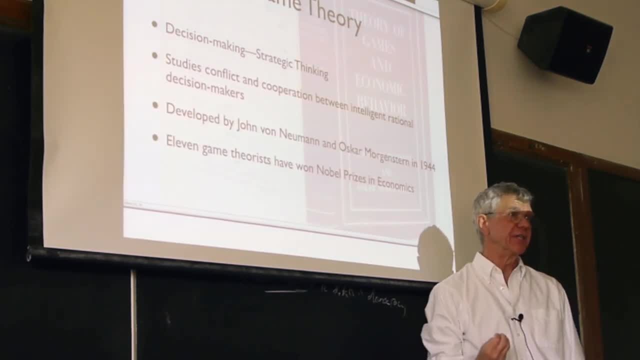 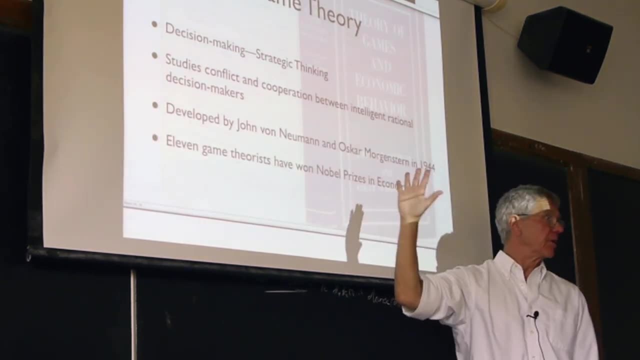 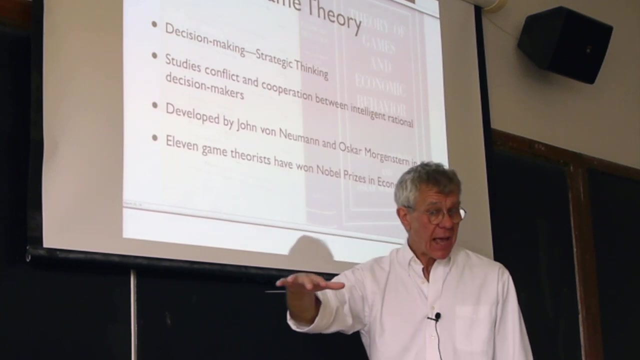 And it focuses on studying conflict as well as cooperation, trying to understand how people in groups address problems. So one thing that's distinctive about it is we don't just think about one agent- how you should act, for example. We think, OK, you're interacting with other people. 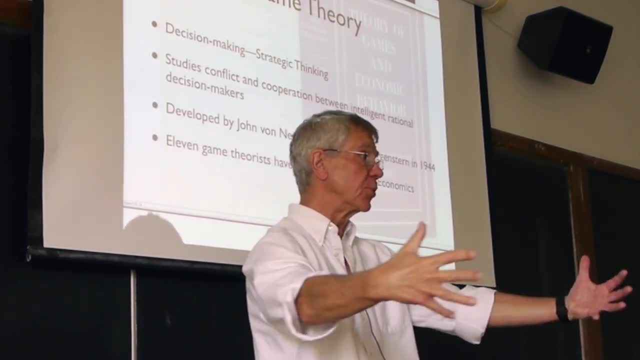 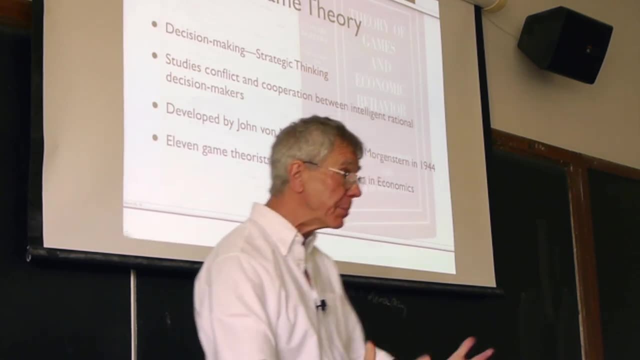 Game theory is about social behavior, about the way in which we interact with others who are also decision makers, And since at least a huge amount of ethics has to do with how we get along with other people, there's a connection there too. 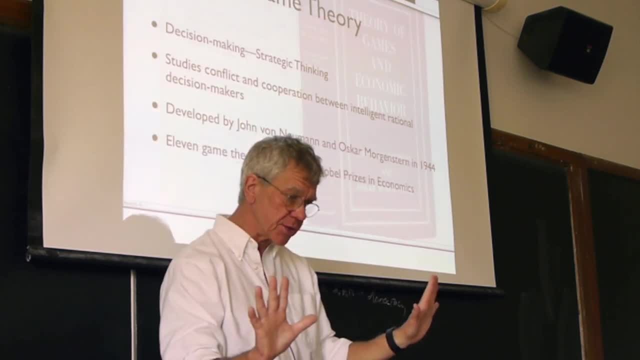 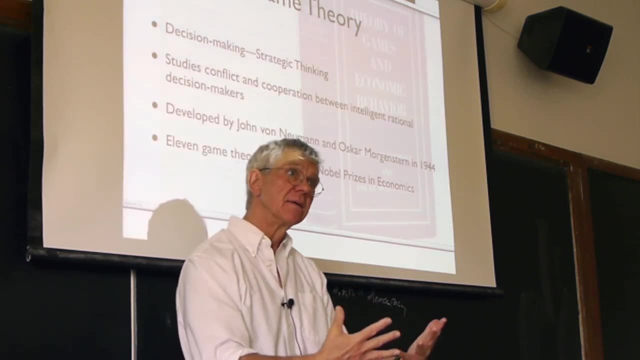 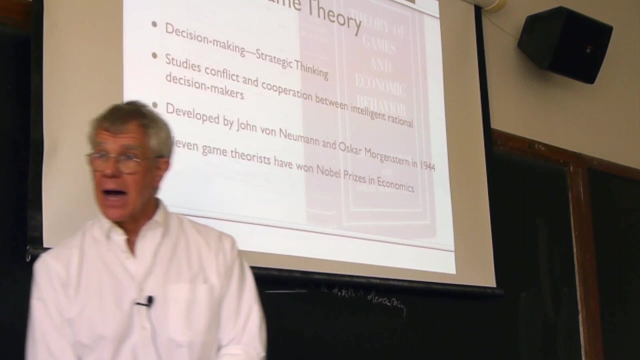 We think. suppose we have multiple intelligent decision makers who are trying to behave rationally. Well, how does their interaction matter? That's something that game theory focuses on. It was originally developed by John von Neumann and Oscar Morgenstern. 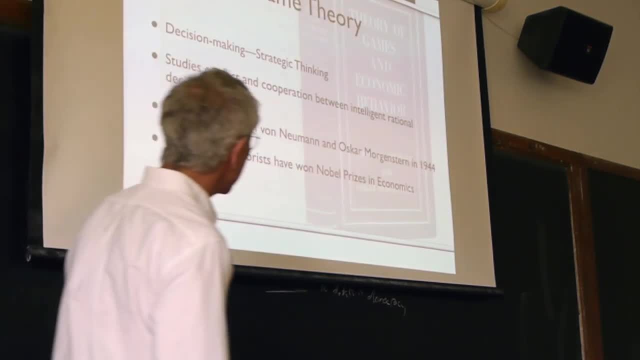 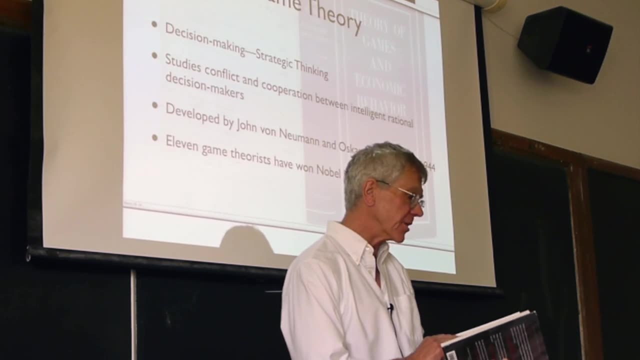 The big book on it is The Theory of Games and Economic Behavior, the first edition. The first edition is shown there. Here's the edition I have. As you can see, it's pretty thick And it's very mathematical. It started with von Neumann's attempt to understand poker. 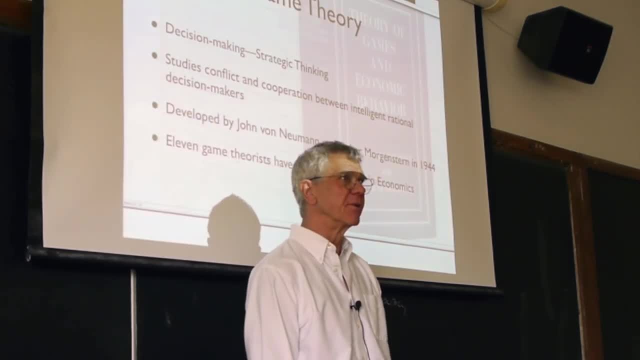 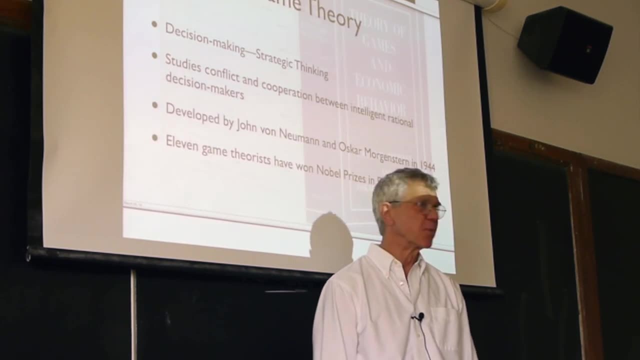 and become a better poker player. Actually, it's pretty useless for poker. Poker is too complicated, And so my son-in-law is a very good poker player. He competes in the World Series of Poker and things like that. I have nothing to contribute to him by knowing game theory. 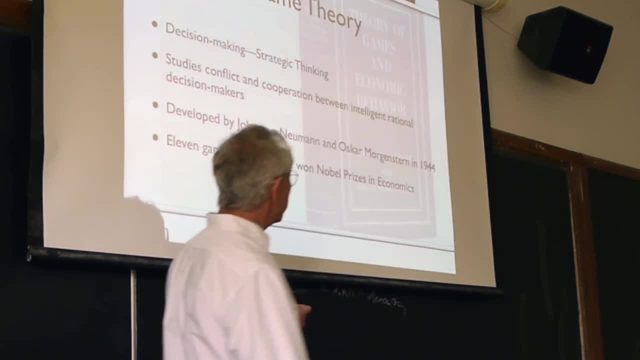 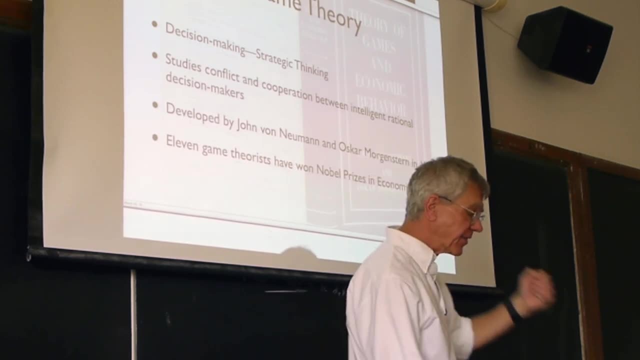 I'm afraid OK. So if that's your hope, yeah, it's going to be frustrated, But it is useful for all sorts of other things And in fact it began to attract a lot of attention in the 40s and in the context of the Cold War. 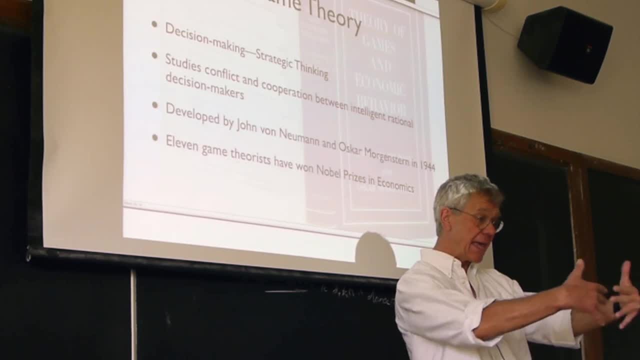 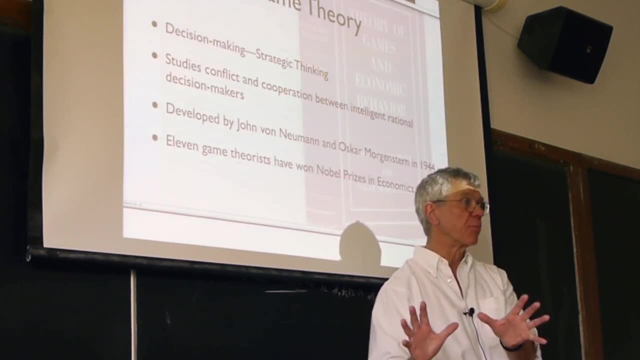 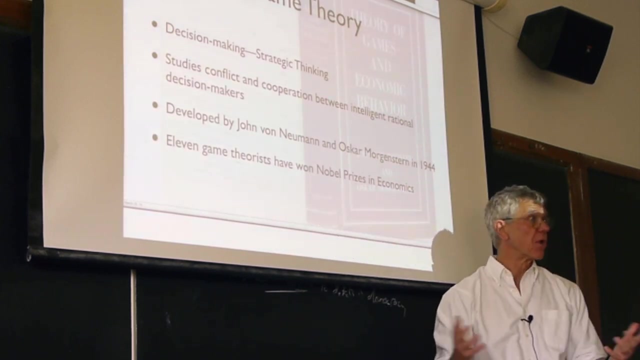 People immediately started thinking: wait, this allows us to game scenarios for nuclear conflict and other kinds of conflict, And so it's something that was studied heavily at the Rand Corporation and by the military in the years after the Second World War. 11 game theorists have won Nobel Prizes in economics. 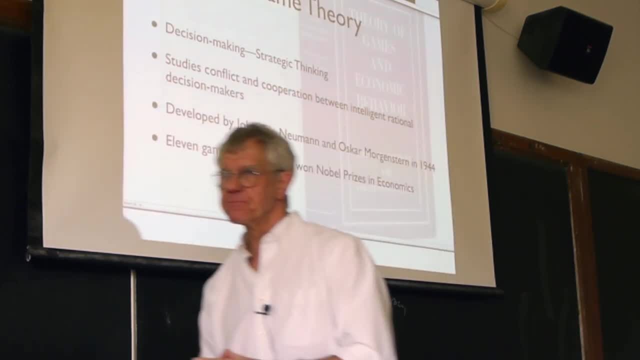 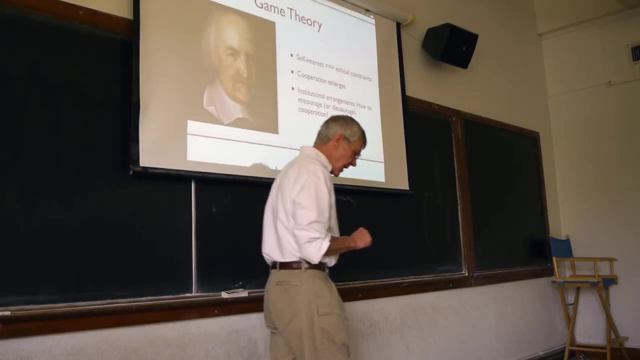 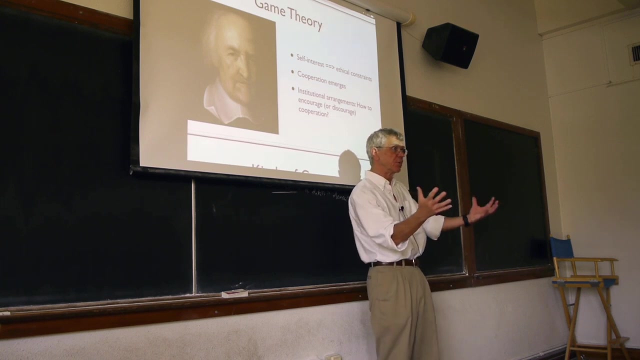 So it's also something that is at the forefront of economic thinking. Now here's one way of thinking how it connects to ethics: The picture there is of Thomas Hobbes, who in a sense had the same kind of attitude about the connection. 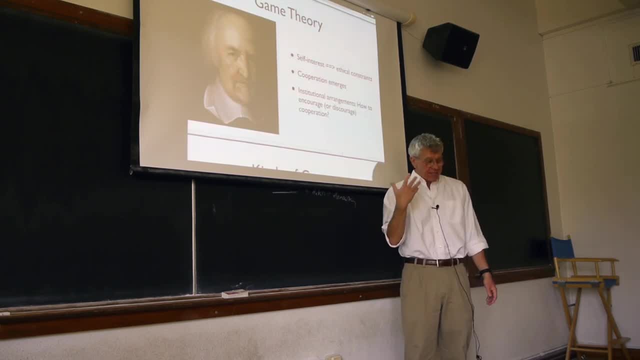 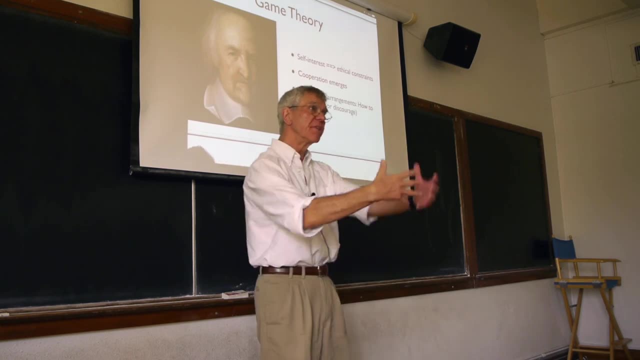 between ethics and strategy. The whole idea is this: Self-interest. rational pursuit of self-interest can actually give rise to ethical norms. We often think of self-interest and ethics as competing, as going at things at loggerheads, And sometimes they are. 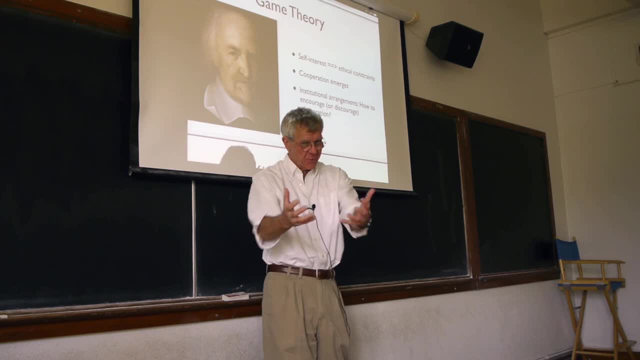 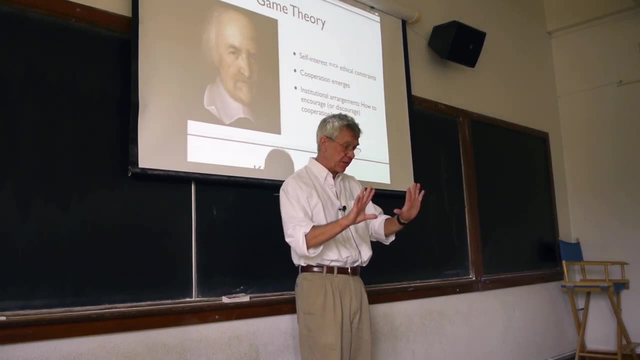 We're trying to do what's right, but we have this real desire to do what's wrong. There are cases where self-interest can conflict with ethics, But on the other hand, if you think about the larger framework of our interaction with other people, 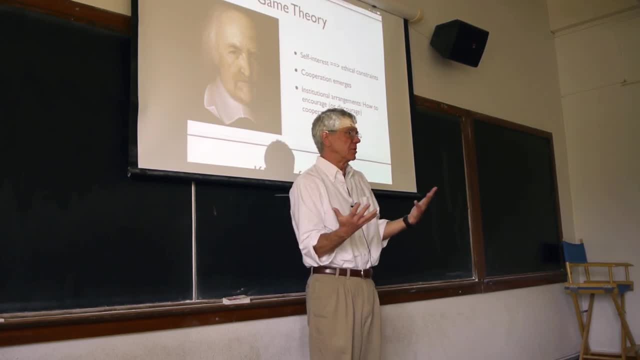 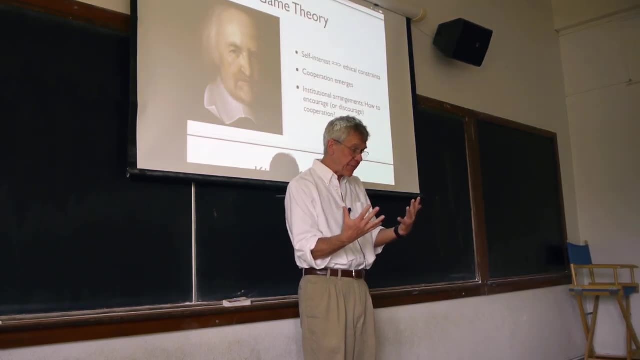 you can start to think: well, wait a minute. Actually, it's pretty rational to be in a system governed by ethical norms. Go back to Hobbes's question. Would you rather be in a state of nature? He's thinking primarily about a state. 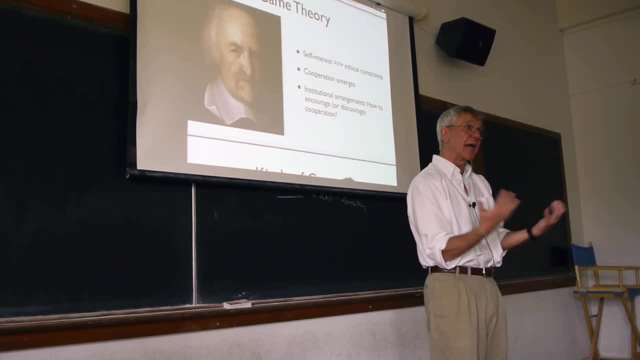 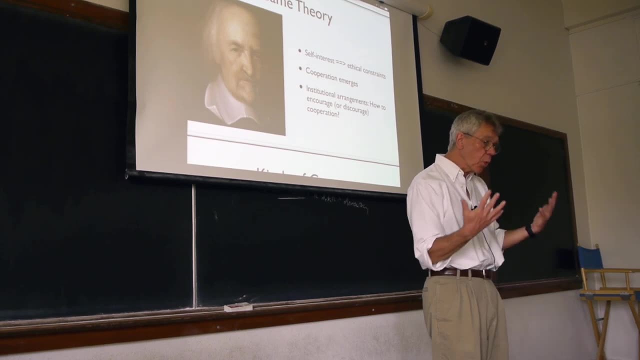 without any political authority at all? But suppose you ask it about ethics. Would you rather be in a society where nobody had any ethics in relating to other people, Or would your rational pursuit of self-interest and other people's rational pursuit of their self-interest 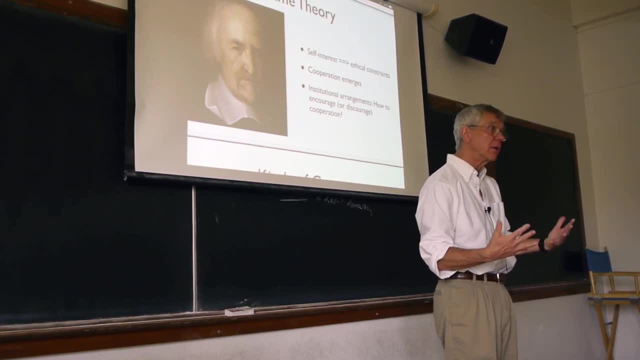 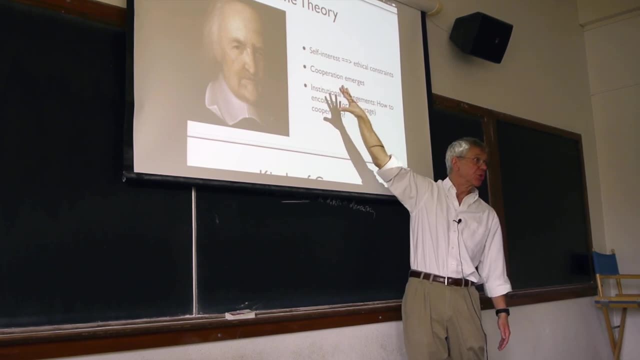 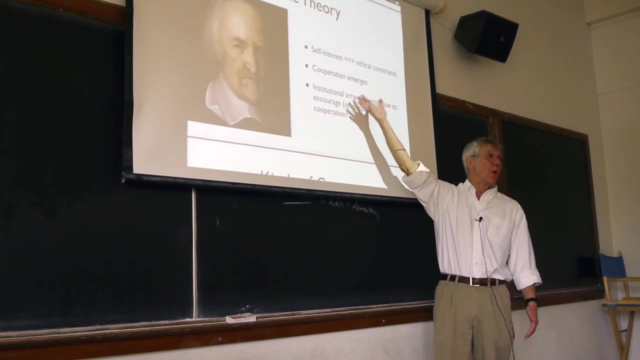 lead to us all agreeing to observe certain norms to get along better. Well, the idea is it would be rational to actually adopt these norms of behavior And, in fact, cooperation would emerge in not only setting up those rules of behavior but enforcing them and finding ways of cooperating. 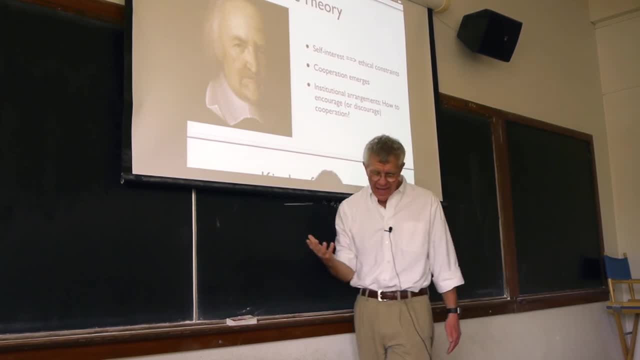 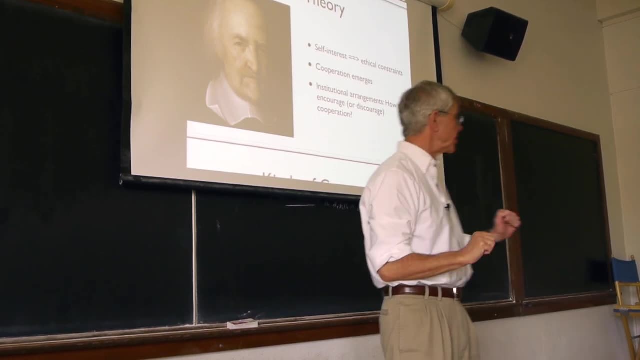 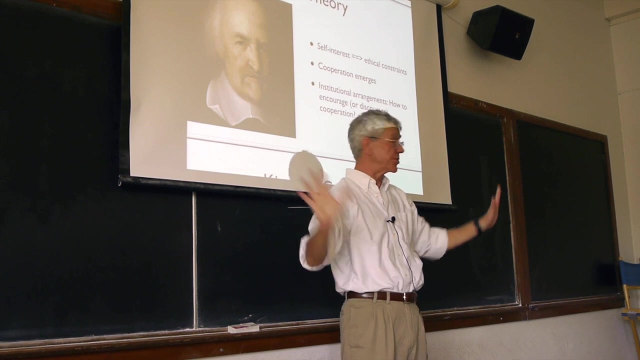 within those rules. So you can think about the sense in which ethics arises out of self-interest. You can also think about institutional arrangements. What kind of institutions do we want? How do we want to structure an organization, for example, or, for that matter, a whole society, in such a way? 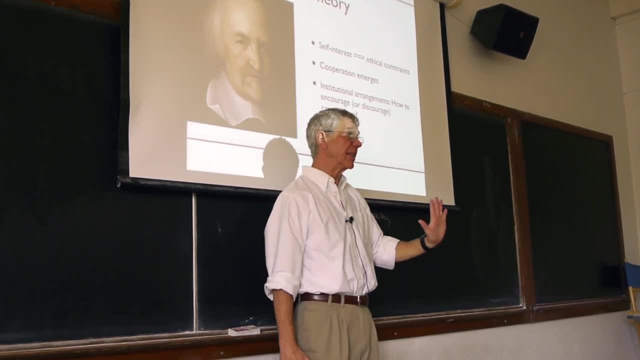 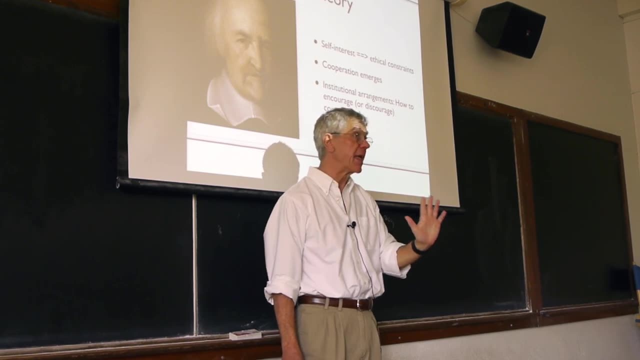 as to encourage cooperation or discourage it. I mean there are good things And bad things about cooperation. Sometimes cooperation is very good, Sometimes it's bad, And it's important to keep that in mind. I mean it's easy to think of examples of cooperation. 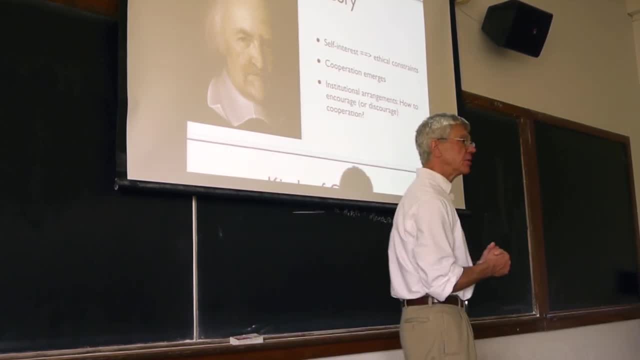 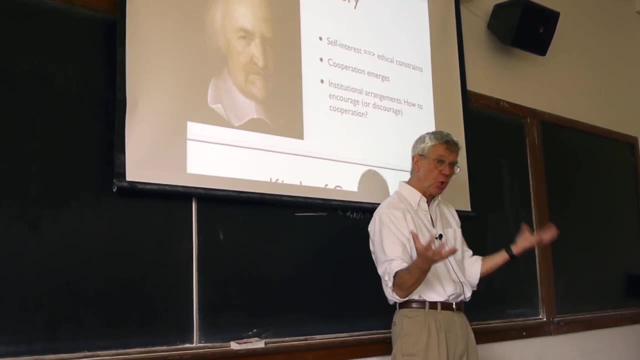 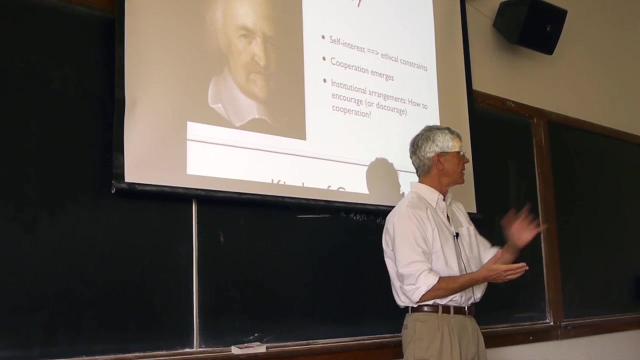 that are good. right, Give me some examples of good cooperation. Marriage, Marriage, OK good, You have to cooperate with the other person, And cooperation is a good thing within any kind of relationship. Other examples: Good cooperation, Yeah. 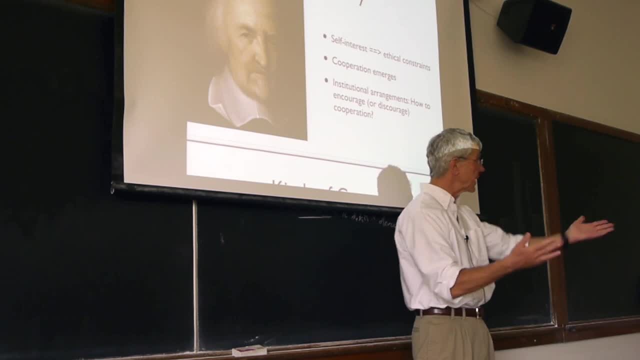 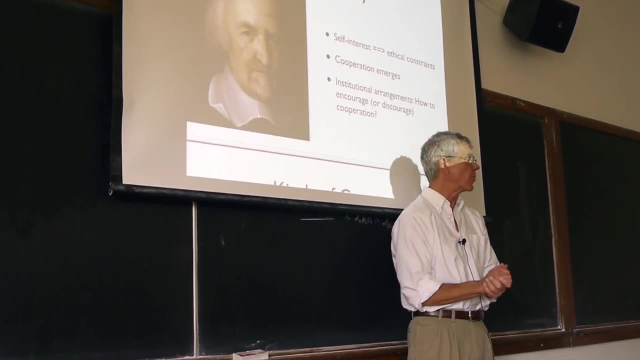 Good, You've got a team project. You split up the work, You all cooperate and do your share, And that's a very good thing. But are there bad instances of cooperation? Yeah, When you have lots of very, very lazy people on the group. 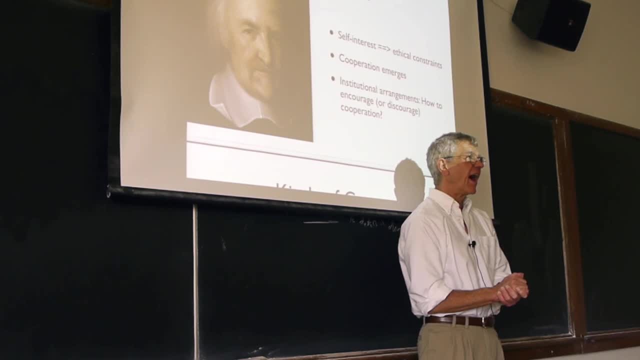 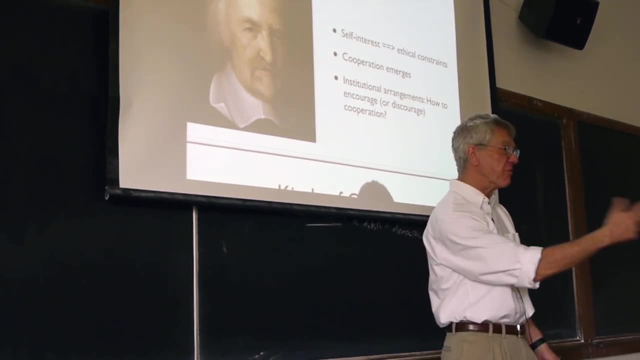 project and two people end up doing all the work. Oh, it's like: hey, you know, those two are hard workers, They'll do all the work. Let's all goof off right, That would be people cooperating to push those people. 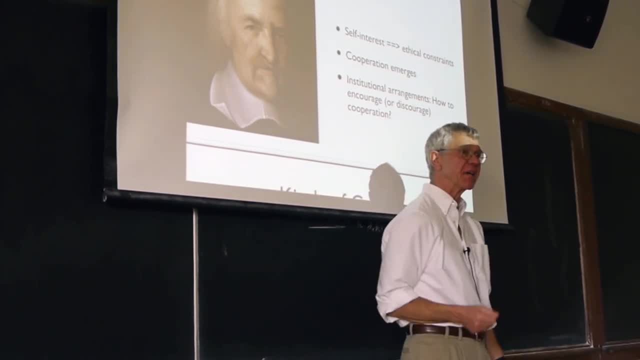 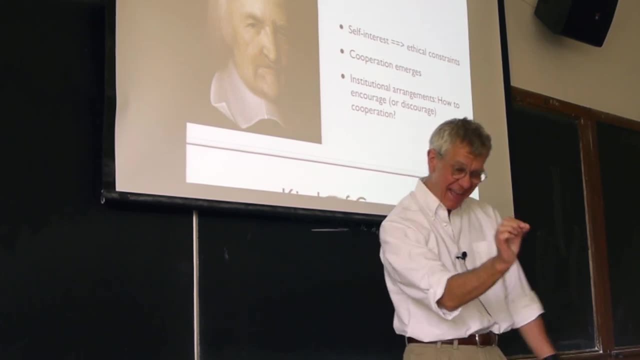 into doing all the work. That would be a bad sort of cooperation. Other examples: Would you like bank robbers? Good Bank robbers, Like: hey, we work together. man, You all right, your job is to kill the guard. 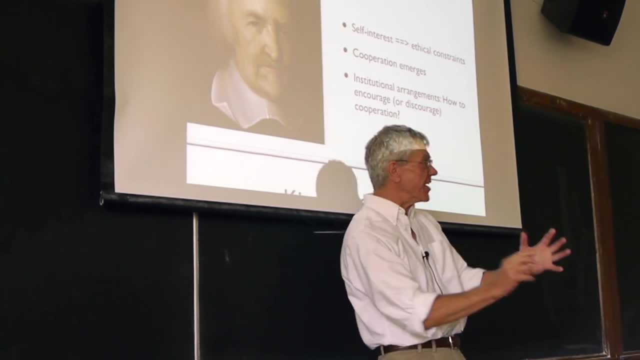 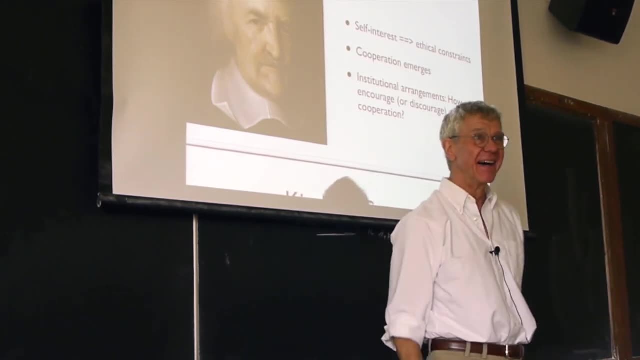 My job is to drive the getaway car. You're going to set the explosive, You're going to go in and get the loot out of the safe, Then all of that would be an example of bad cooperation. Yeah, And tragedy of the commons problems. 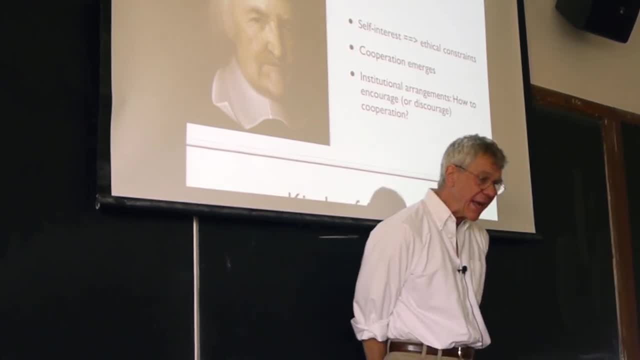 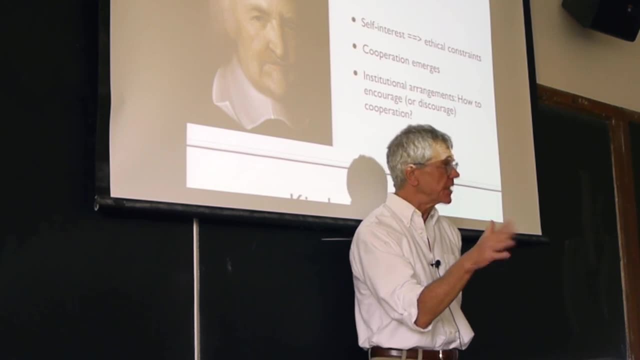 Ooh, tragedy of the commons problems. Yeah, So think about ways in which I mean Sometimes that arises because people don't cooperate, And we'll talk about those problems a lot next time- But sometimes they can arise out of cooperation. Suppose we are a bunch of business people who agree to fix prices. for example, It's like: hey, you know, you've been selling your airline tickets for less than we're putting on our website. Why don't we all agree to raise our prices? 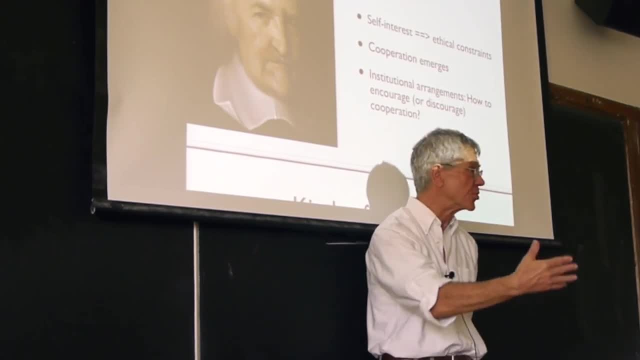 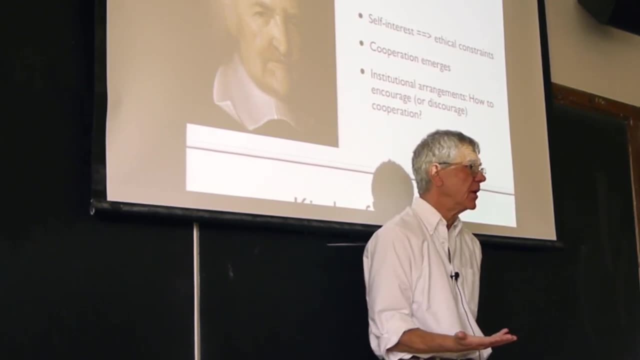 We'll all make more money. That would be an example of a bad sort of thing. price fixing Cartels can be like this: right A cartel is often. It's often a bad form of cooperation. The mafia is a bad form of cooperation. 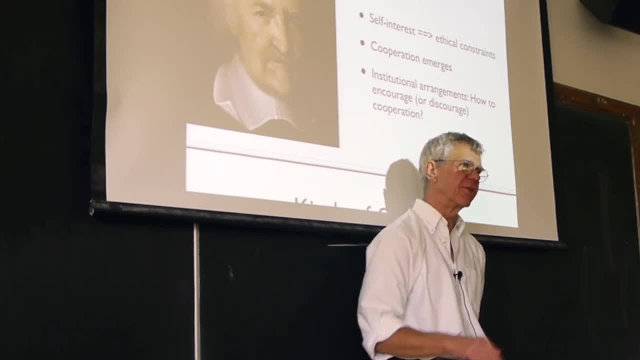 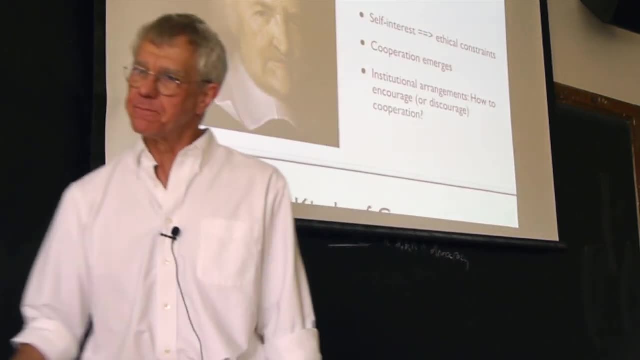 Hey, you don't whack me, I don't whack you, But we'll whack those guys together, OK. OK, that's bad, That's a bad form of cooperation Now. so, in short, we want to encourage the good kinds. 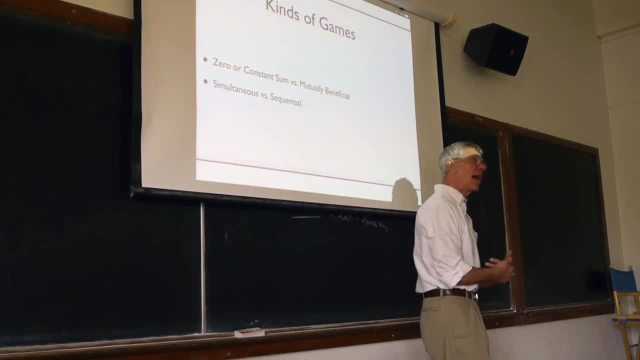 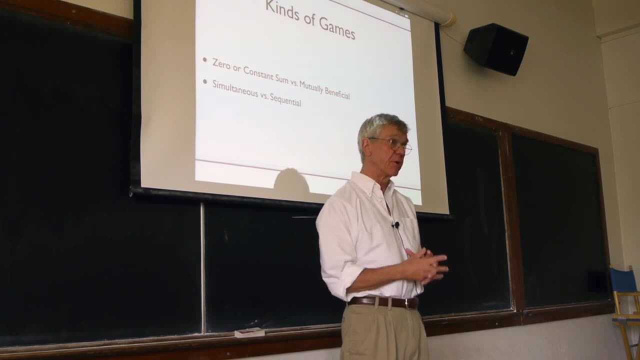 discourage the bad kinds. There are different kinds of games, And one of the things you have to do at the very outset of analyzing a problem in these terms is understand What kind of game you're playing. So today I want to talk about two distinctions. 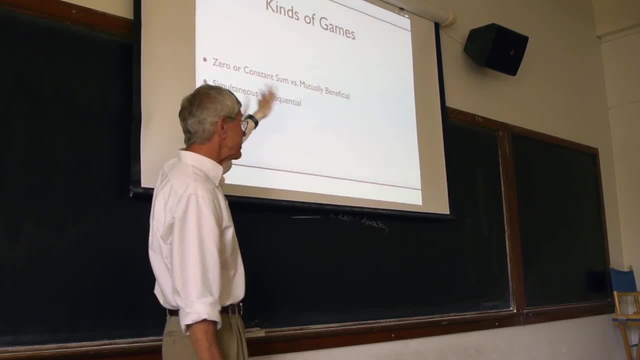 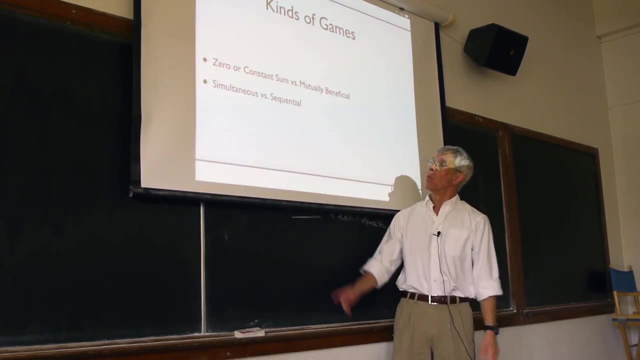 The first between a zero or a constant sum game, and really mathematically they're equivalent. And then mutually beneficial or, for that matter, mutually harmful games, But ones where, in short, if one person wins, it comes at somebody else's expense. 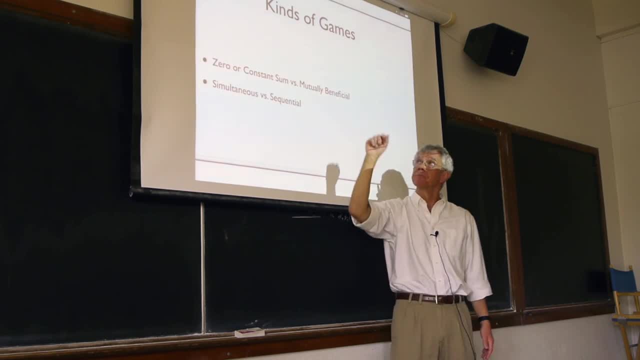 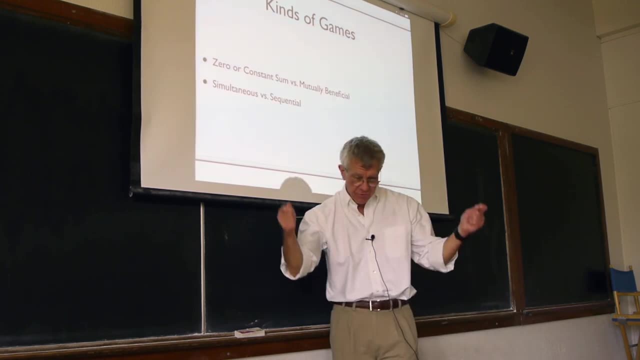 as opposed to games where both people can benefit or both people can lose. And then we want to talk about the distinction between simultaneous and sequential games. Sometimes You and I have to play at the same time without knowing what the other person is doing. 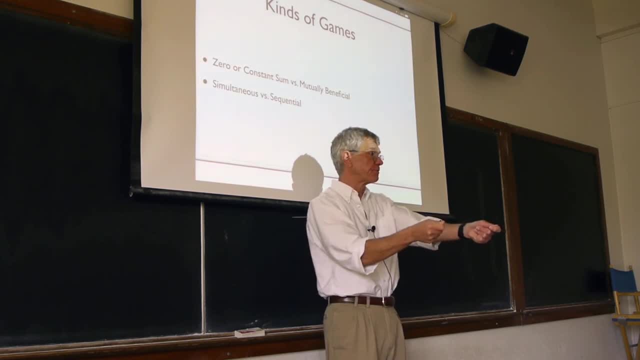 At other times you move first, then I move, And that makes a fundamental difference. Do I know what you are doing, Right? In the one case, I don't. You and I let's say we're, I don't know, we're well. 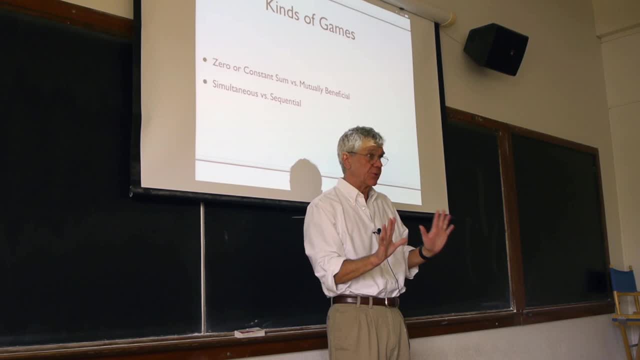 we're going to talk about examples in a moment, But a simple thing as we'll talk about is a game of two-finger mora, where we have to hold up one or two fingers and then one of us is odds and one of us is evens. 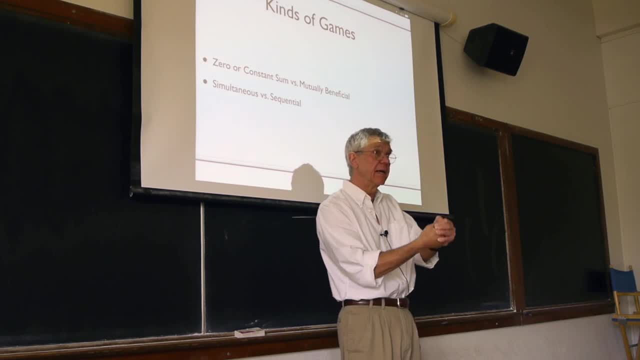 And I don't know whether you're going to hold up one or two fingers when I make my play, And so that's a case of a simultaneous game. We have to do it together. It's not very fair if we say, OK, yeah, I'm evens. 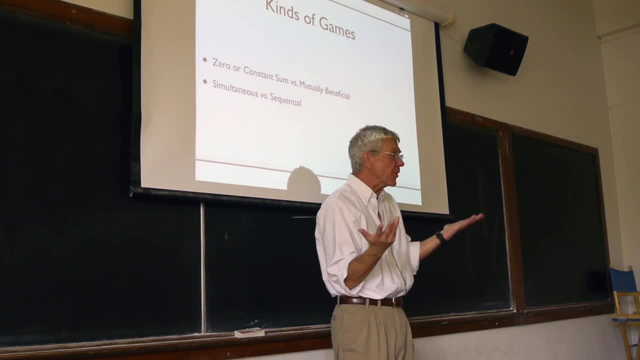 Yeah, now you go Right, Then you know exactly what to do. Other games are sequential. In chess it's not like we both move at the same time without seeing what the other person's doing. I'm white-moved, Then black moves, and so on. 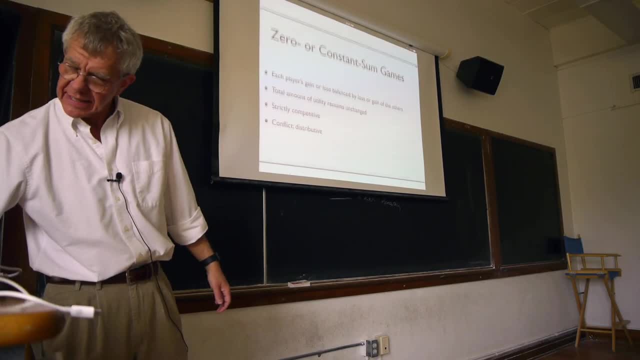 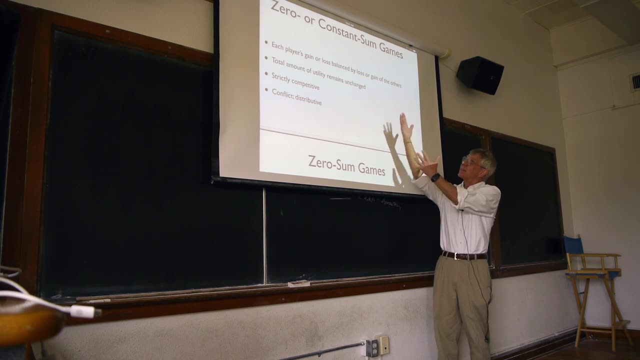 So it's sequential. So, anyway, we'll talk about each of these in more detail. A zero-sum game is a game where, well, there's a constant amount being allocated among the players And each player's gain or loss is balanced by a loss. 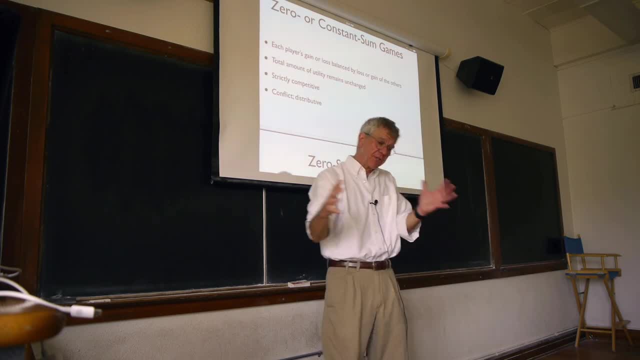 or gain from other players. OK, So the total sum remains the same. Now it might be that it's just zero: I win, you lose, And the average of that is just sort of the same as it was before. But it might be that, let's say, we're carving up a pie. 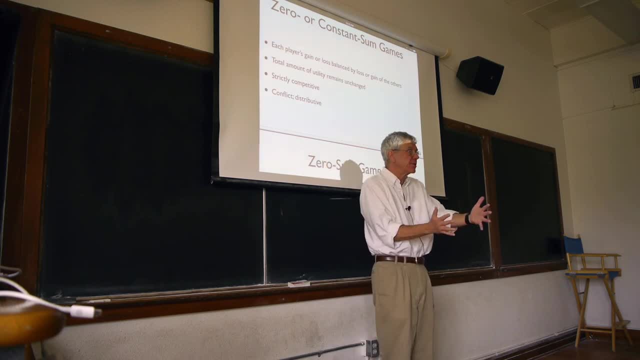 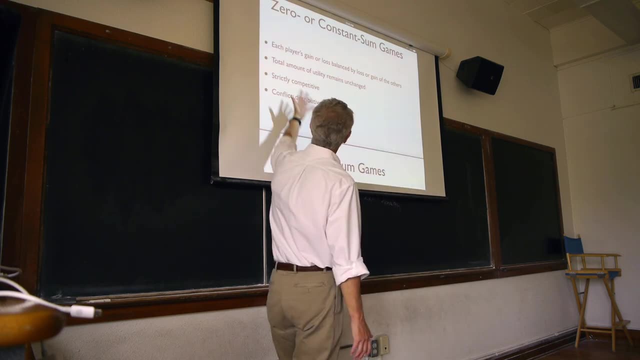 And it's the same amount of pie. If I get a bigger piece, you get a smaller piece And it's like the pie doesn't grow or shrink as a result of what we do in cutting it. So those are cases where you might. 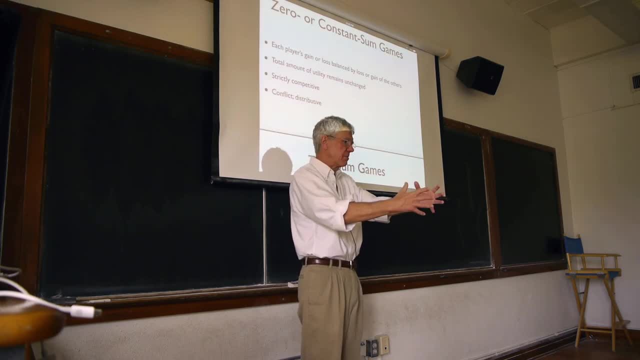 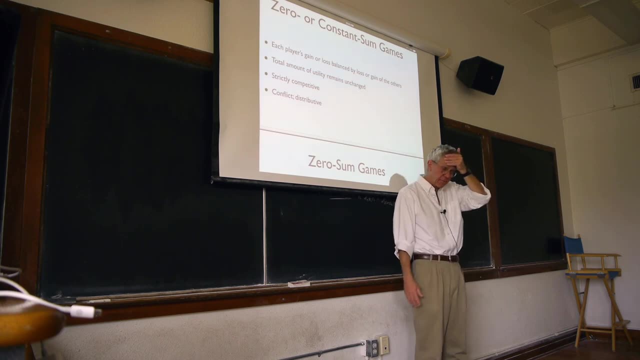 say, the total amount of utility, whether it's zero or some other sum, is left unchanged. It might be a positive thing or it might be a negative thing, Like: ah, we have this debt, Where are we going to get the money from? 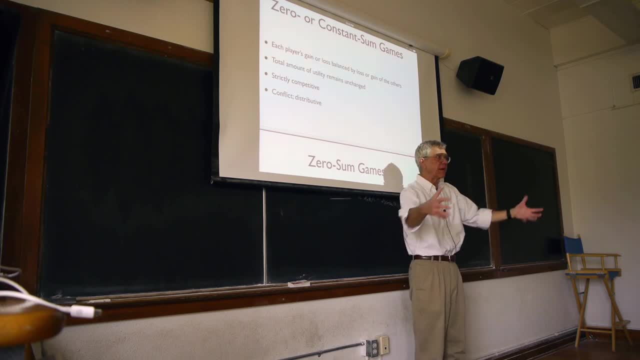 We take it from other parts of the budget And it's the same amount we have to take. It's just a question of where we allocate the losses. So all of those would be examples of zero sum games. Now, these games are strictly competitive. 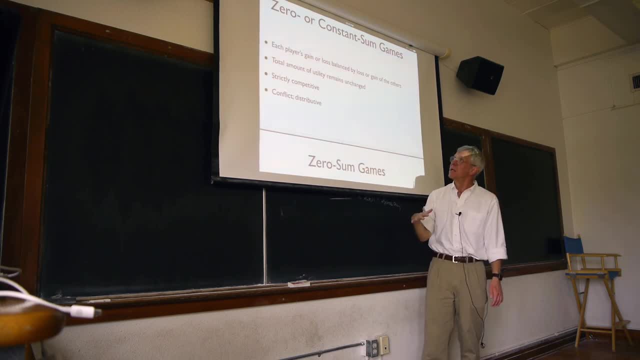 One person's benefit comes at the expense of other people, And in that way they're good for modeling conflict or the question of distribution of a fixed pie: SPEAKER 1.. SPEAKER 2. Ah, a fixed amount of something. 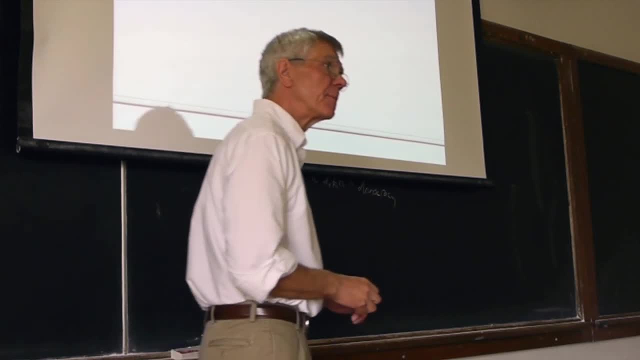 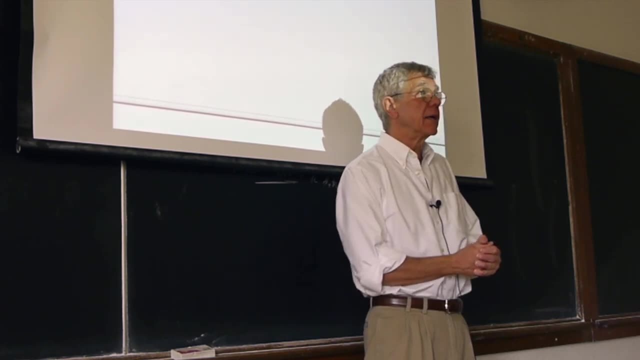 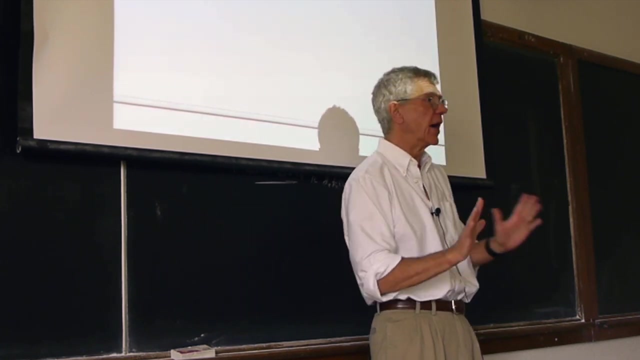 So what are some examples of zero sum games or constant sum games in practice? SPEAKER 3. SPEAKER 1. Ah, is war a zero sum game? OK, Some people are shaking their heads. no, Why not? SPEAKER 3.. 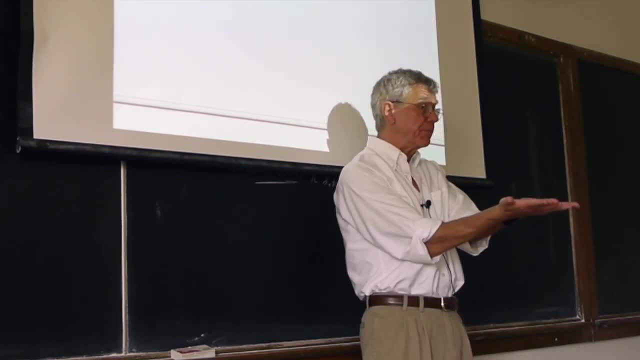 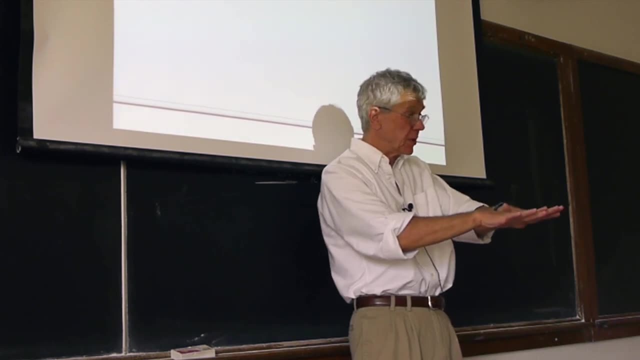 Ah, OK, good, There could be ways in which it might be mutual. There might be mutually beneficial solutions to conflict like a treaty. There might be mutually damaging ways of going And the amounts of damage might change a lot, right. I mean something that escalates to a nuclear war would presumably be a lot more negative than a war fought by conventional means, other things being equal. And then that might be more damaging than a limited conflict by proxies in some remote region of the world and so on. 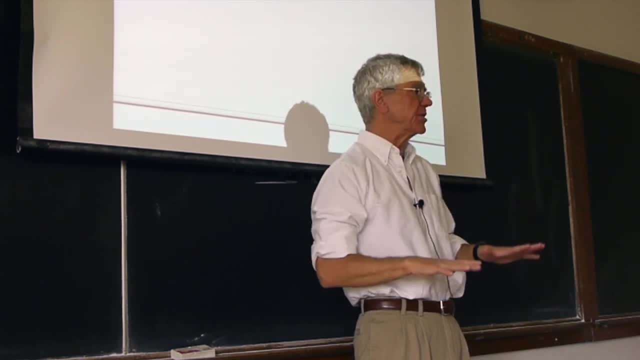 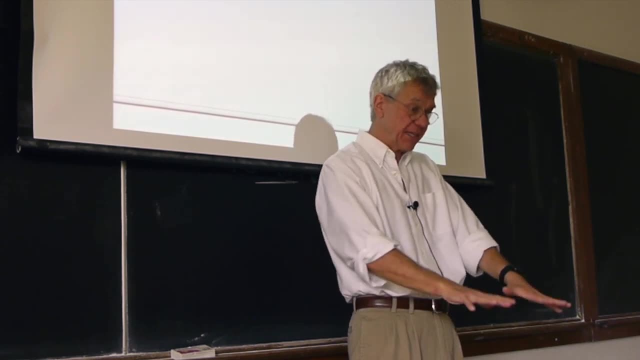 So there are lots of degrees of loss, degrees of harm, And if you're doing a war game it's not simply like, ooh, we win, you lose. It can be: look, we both suffer horrendously, We both kind of benefit. 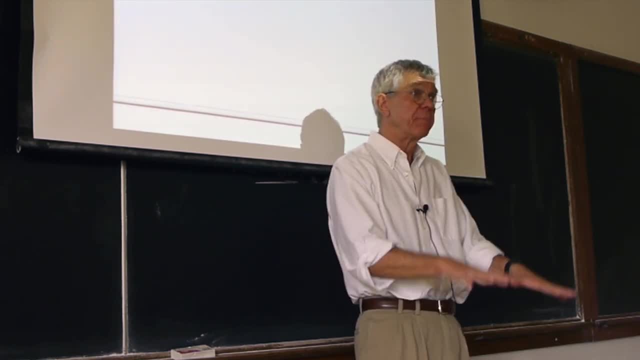 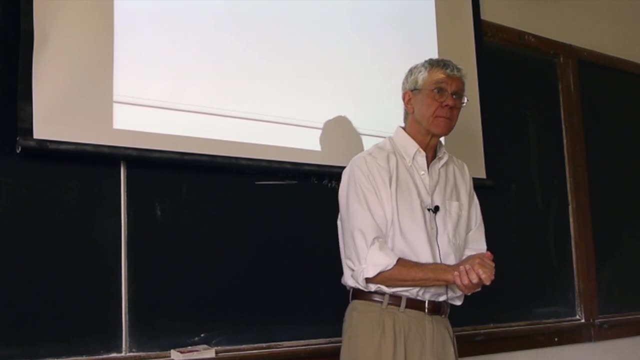 We both suffer a little, So that's not a constant sum, But what would be an example of a zero sum game? Yeah, SPEAKER 4.. Is an ultimatum game a zero sum game? SPEAKER 3. Tell us more about what that is. 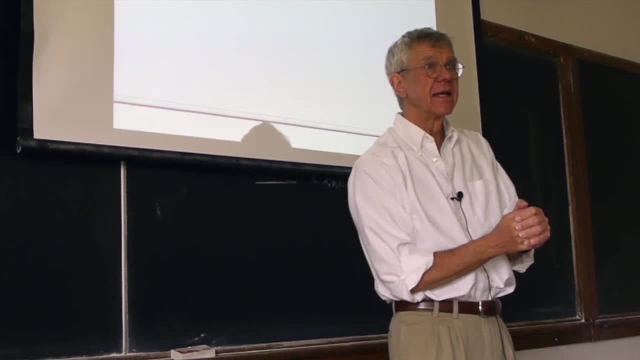 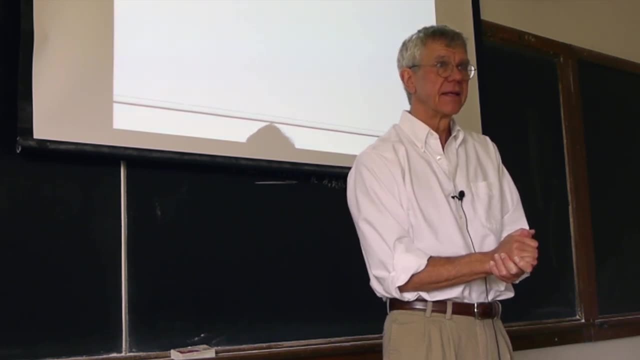 What's the ultimatum game? SPEAKER 4.. SPEAKER 5.. It's basically like you have two players. One player is guaranteed to get $100. And he's allowed to distribute that to the other person however he wants. 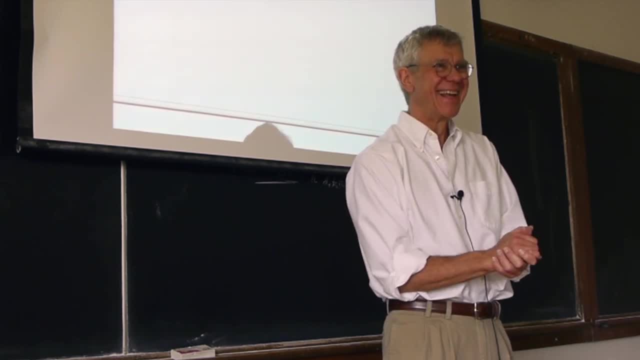 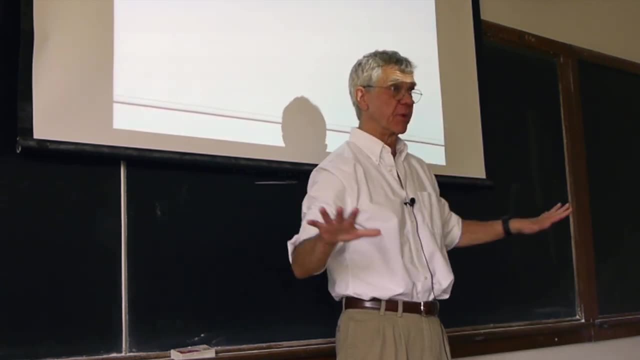 But the other person has to agree with the other person to vote And the other person does not agree with the other person. SPEAKER 4.. Good, good, good. Yes, So they actually do this experiment, often with undergraduates. 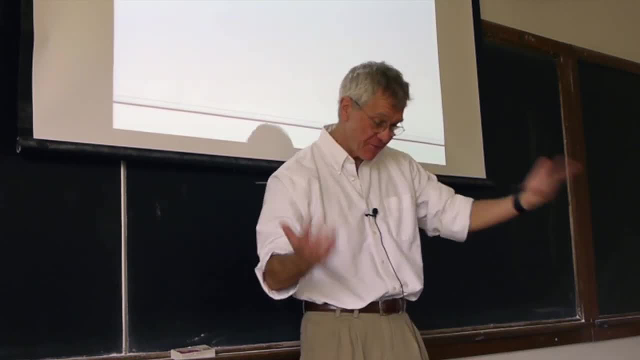 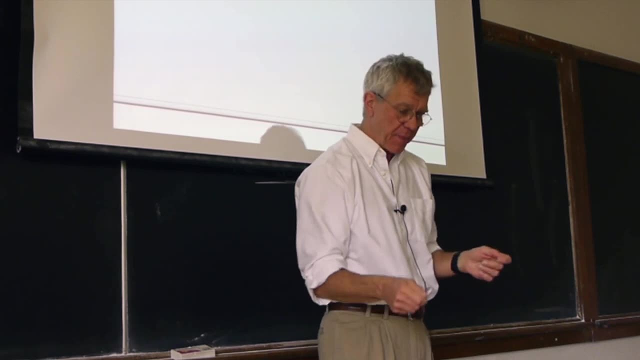 You guys are the guinea pigs of the psychology world, the behavioral economics world, But they do this kind of thing. They bring you in and there are two people- Let's say you two- And the experimenter gives you $10 and says: 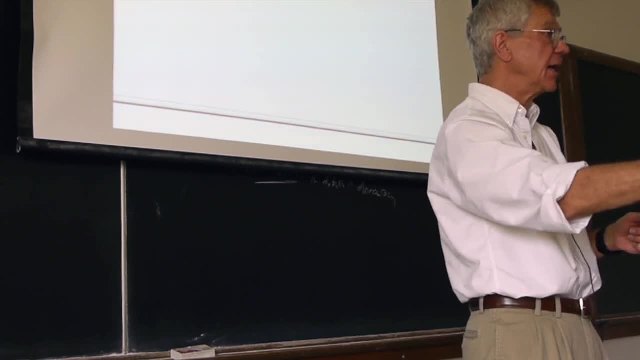 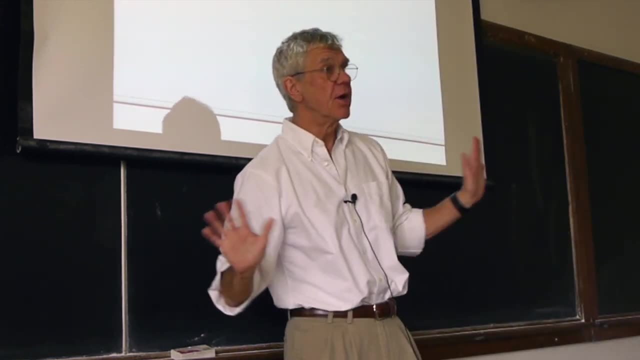 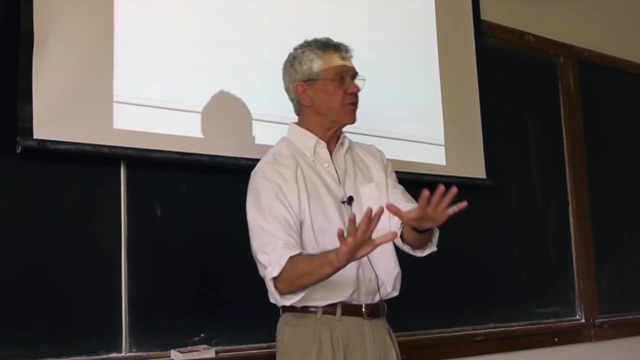 now you can give him any portion of that $10 you want, And you both get to keep the money, provided that he agrees. But if he says no deal, then neither of you gets the money. So what do you do Now? from one point of view, you could say: well, OK. 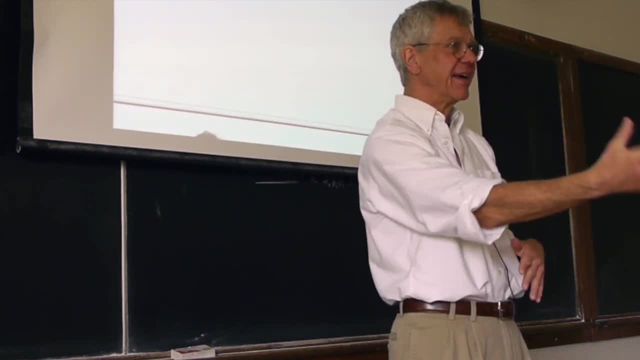 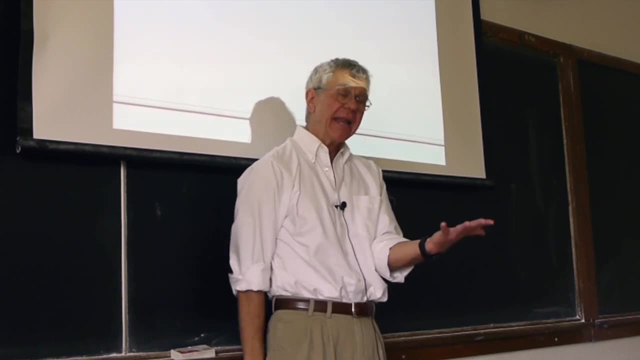 if he keeps the $10 and says, ha ha, I got it. you get nothing, Presumably he's going to say, Well, screw you, You don't get the money, So he's going to say no deal. 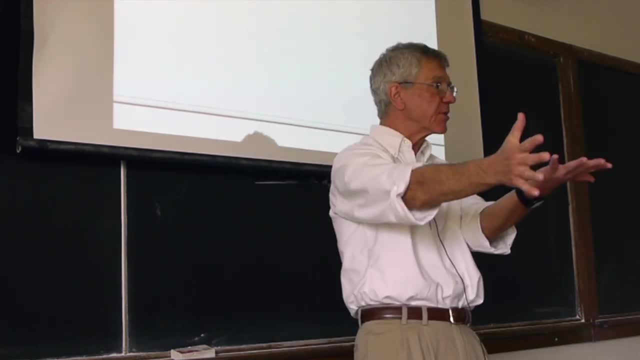 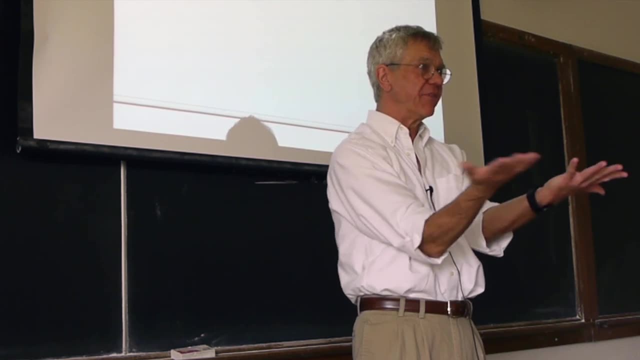 Now suppose you offer him $1. It looks like, rationally speaking, well, he's better off by $1, right? And so wouldn't that be reasonable, Shouldn't he agree? If he doesn't agree, he has no money. 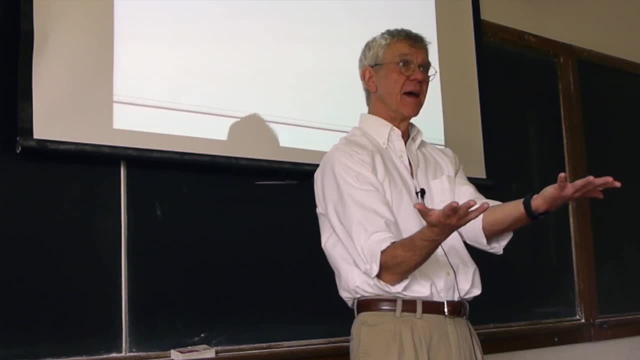 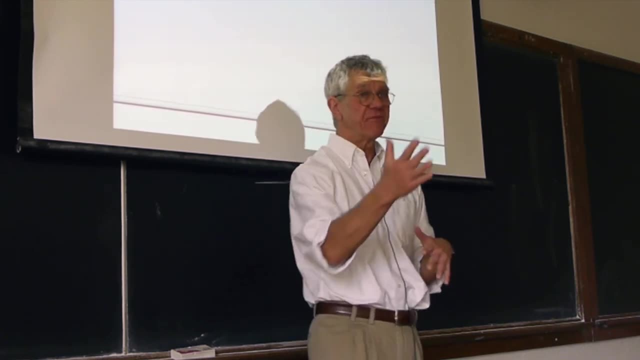 If he does agree, he has $1 at least, But lots and lots of, and some people think that way, But a lot of people will say no, no deal. I want my share Now if you offer him $5.. 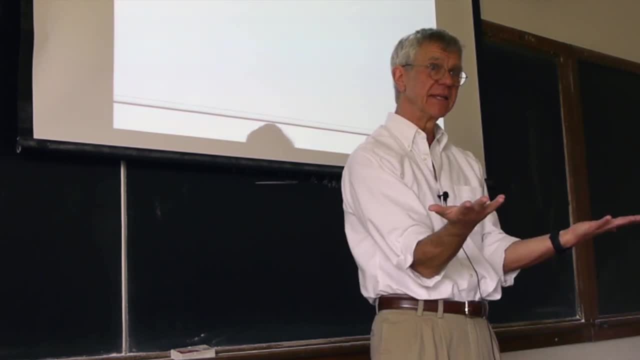 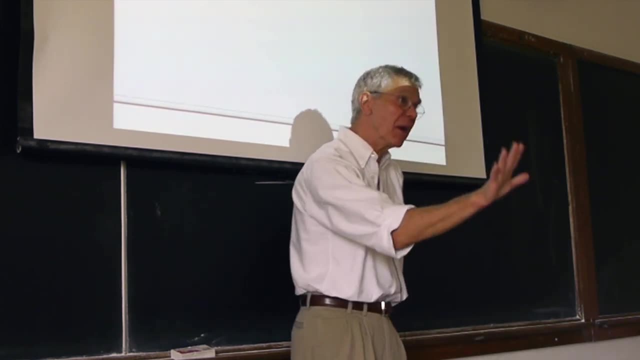 $5,. almost certainly he'll agree. You're splitting it evenly, right? Seems fair, Unless he's really, you know he might be saying: no, I get the $9.. You get the $1,. right, But most people will go along with an even split. 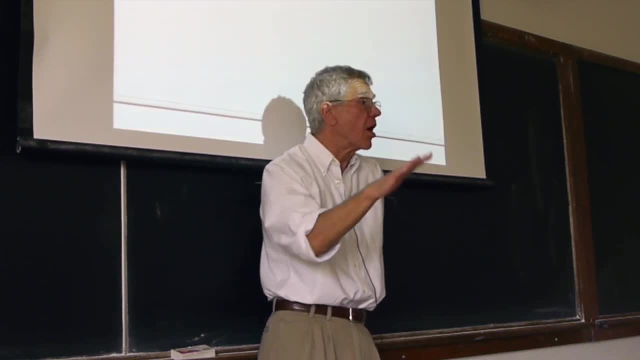 But how far does it go right? And so behavioral economists study this kind of thing to find out how much inequality people will tolerate in that situation. And it's sort of interesting. As long as the other person gets $3,, most people will agree to the deal. 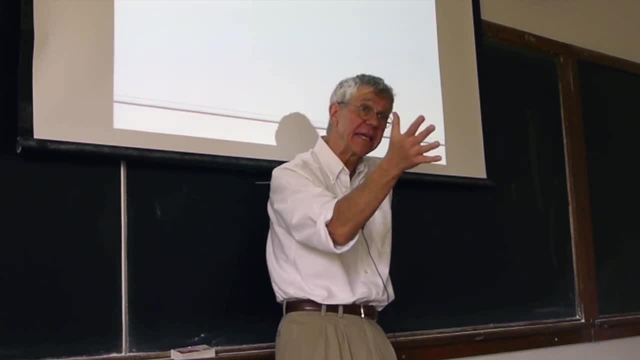 But there's a sliding scale here. Anyway, it's an interesting game, But- notice, it is a zero-sum game. There's a fixed amount, in the sense that it's $10.. However, that's given that you actually divide it up in some way. 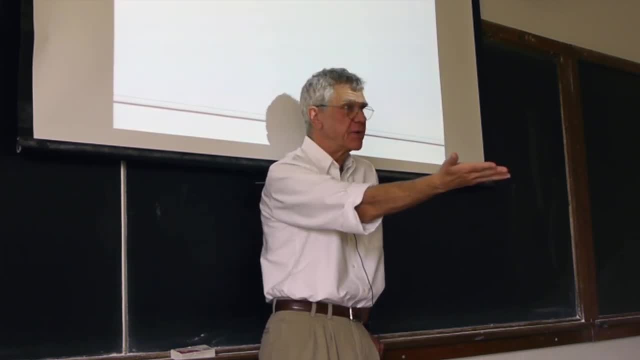 I suppose if we include the experimenter, if he says no deal and you get nothing, when I view it as you two, aha, it's not zero-sum anymore. You lost the $10 amount. On the other hand, if I include the experimenter, 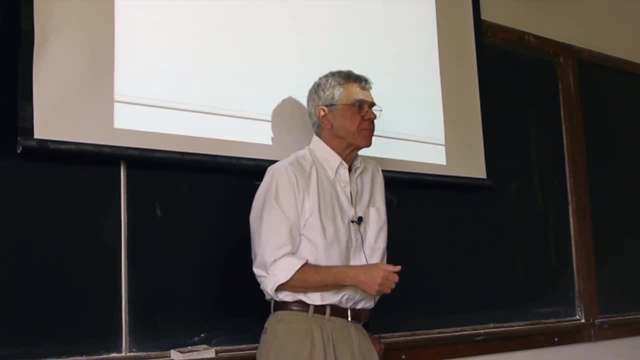 then it looks zero-sum Because he at least gets the money back. So other examples of something that would be a zero-sum game: Yeah, Cutting the cake and sharing the slices- Good. cutting a cake at a birthday party: You're cutting the birthday cake. 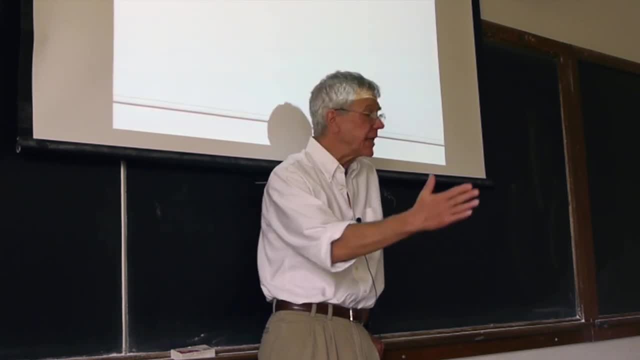 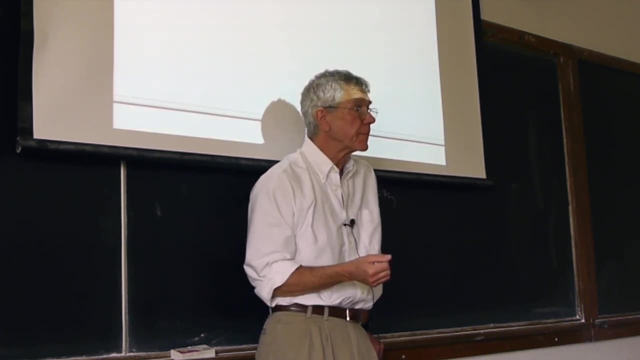 There's a fixed amount of cake And you are allocating it among the people. If you get a bigger slice, somebody else is getting a smaller slice. Yeah, If people throw their money together and sit down and play cards to see who gets the money. 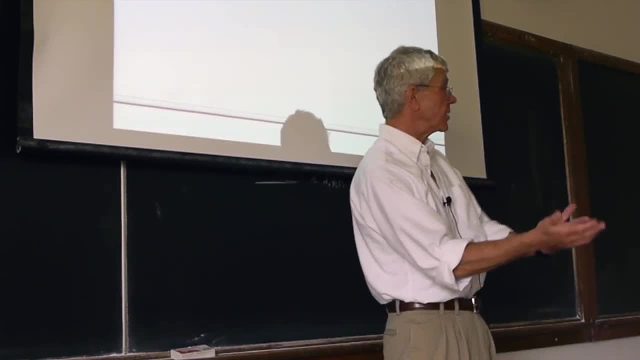 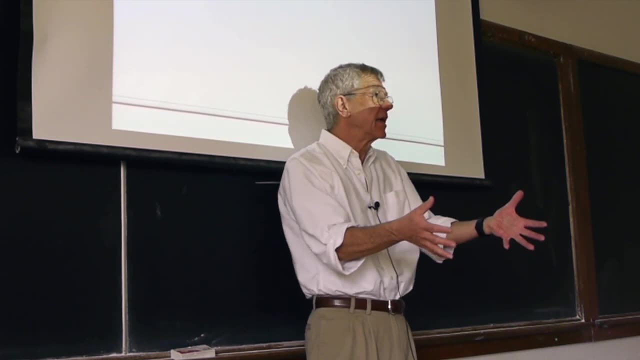 Oh good, You put your money in a pocket, You put it in a pile and you play cards to do this. You have, in effect, a little tournament And you find out, And the winner takes all. let's say: 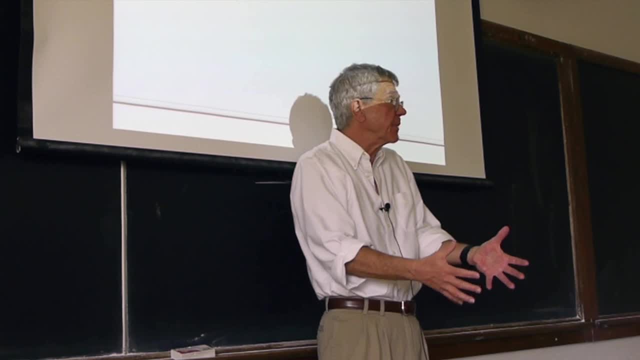 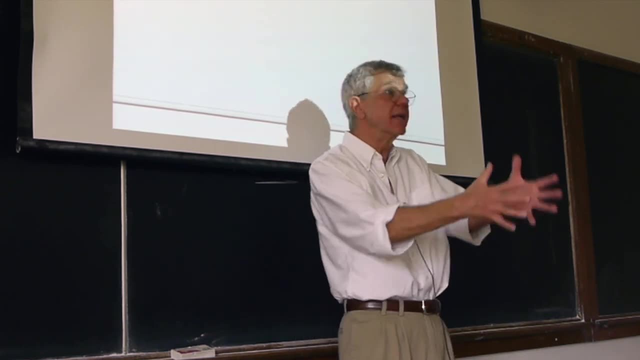 That would be a case of a fixed amount. It's not as if playing makes that amount that's in the pot grow or shrink. It's something that is fixed and then it's just a question of how it gets allocated and who it gets allocated to. 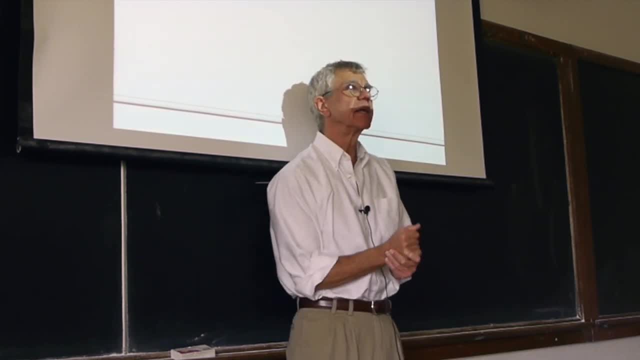 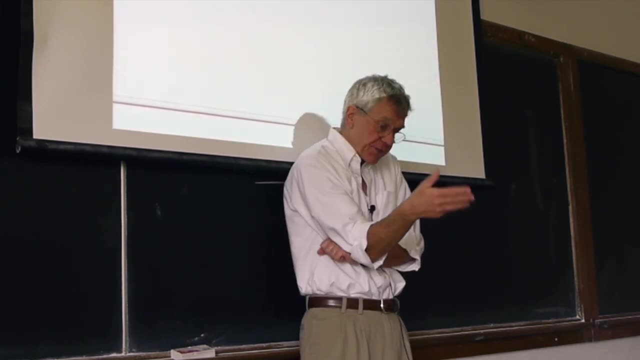 Yeah, Elections, Elections. Ah, Is an election a zero-sum game There? Yeah, One way to look at it is to say there are only a certain number of votes, And if this candidate gets more votes, the other person gets less. But of course more or fewer people might vote. So really to have it be zero-sum, we'd have to have a situation where the number of votes cast is the same. If people just sit at home and don't vote, then one candidate might get more votes just. 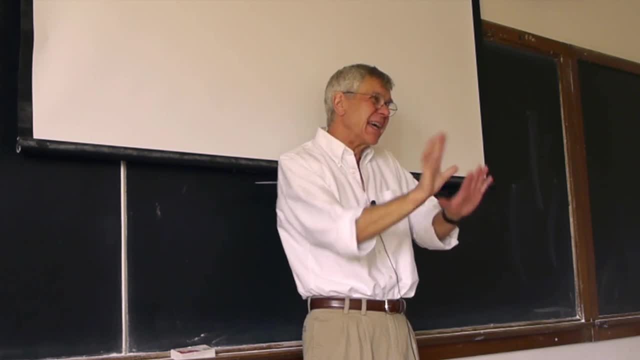 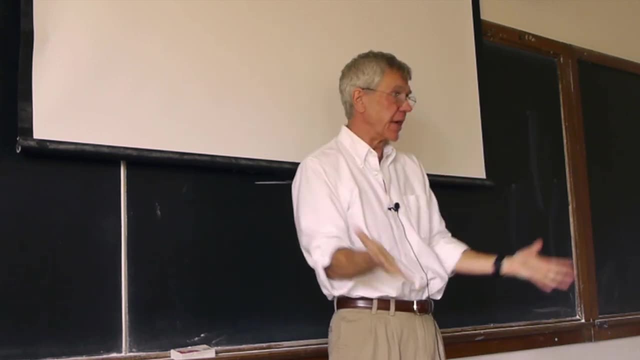 by attracting the people who otherwise wouldn't vote at all. So if you think of percentages of the vote that you get, it looks zero-sum because the percentages by definition have to add up to 100% If we're thinking of the actual total number of votes. 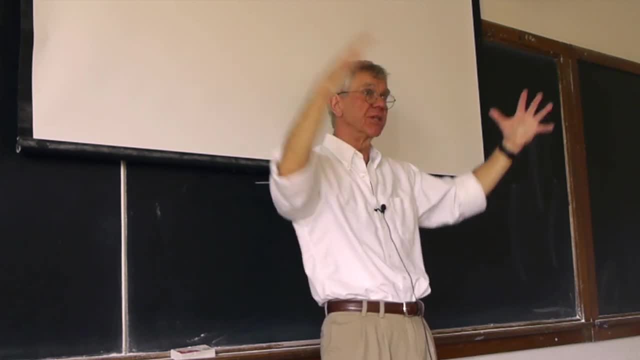 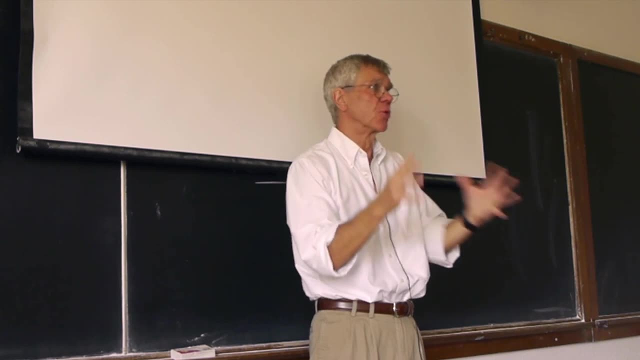 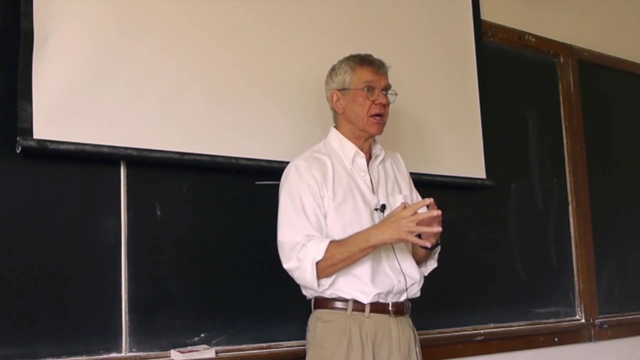 that might be a number that increases or decreases depending on the public's interest in the election. By the way, that itself can be gamed. The Austin City Council is extremely good at gaming elections. in that respect, Here's a proposition that has to go before the voters. Do we want it to face a large number of voters or a small number of voters? Yeah, We could have a special election in the middle of May so that hardly anybody votes. We could actually allocate it for the main primary or the main election in November, when lots of people 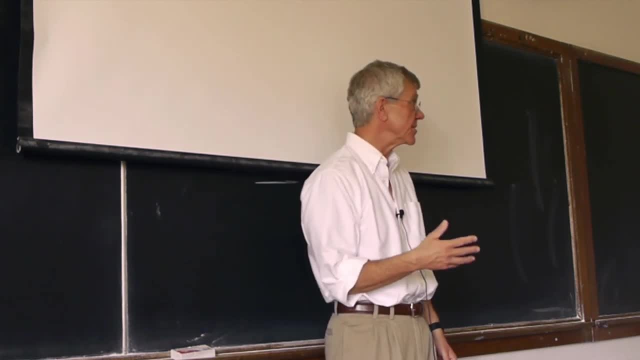 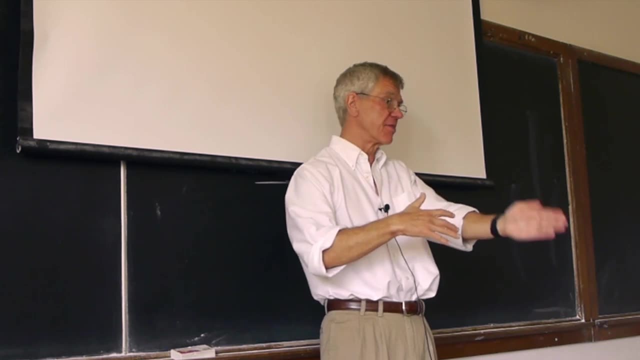 will vote on it, And they often make that decision on the basis of how they want it to come out. So that's a good illustration. A lot fewer people are going to vote in the third week of May than will vote on the first Tuesday in November. 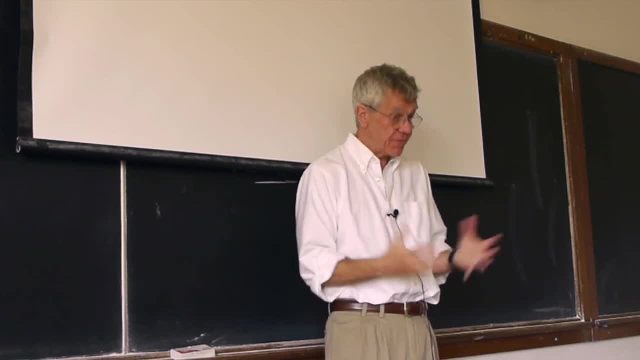 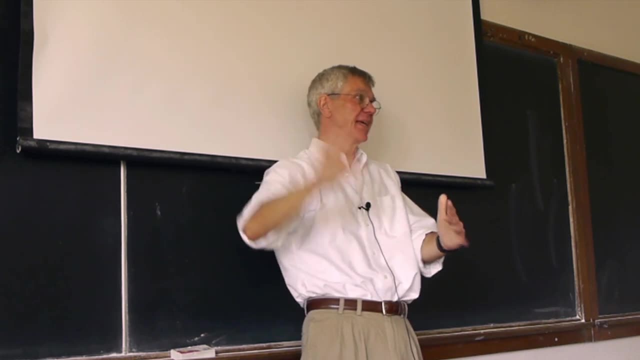 And you can use that to game the thing. figure out. we've got a dedicated group of people who are going to show up, no matter what. They'll be overwhelmed in November, but they can dominate in May, So it can make a big difference. 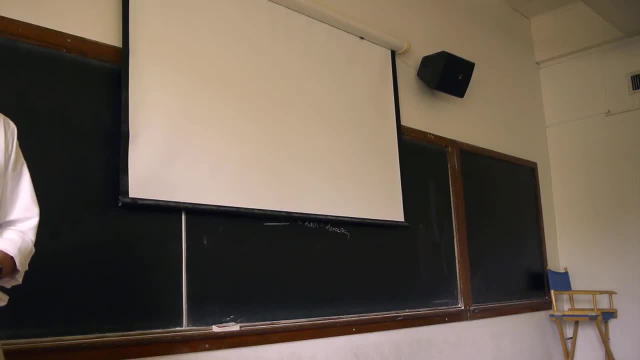 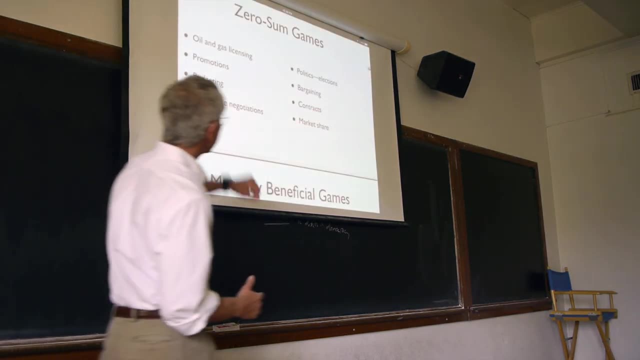 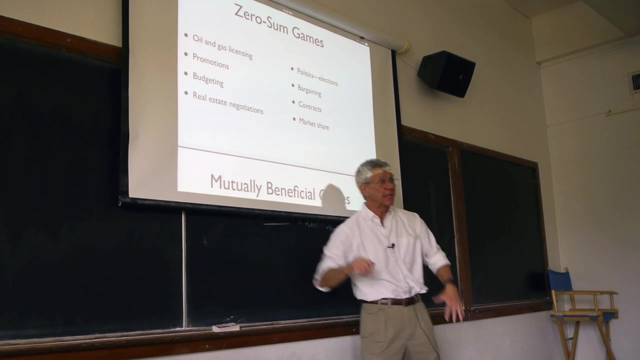 OK, well, those are examples of things that are zero-sum games. They're actually a little less now. everybody in the world knows mine. Here are some other examples: Oil and gas licenses. You might have a certain territory. You divide up the licenses among different oil and gas. 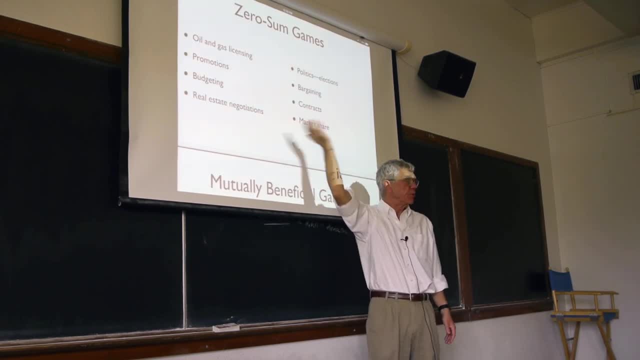 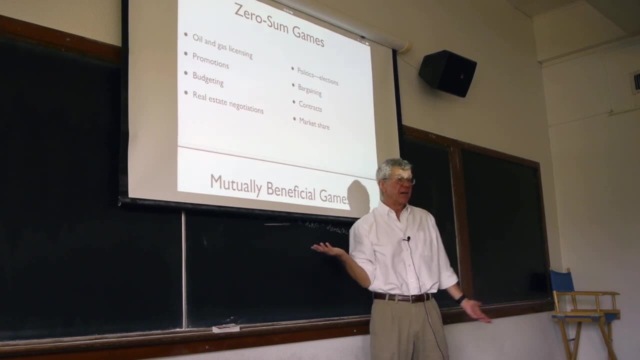 companies for exploration. That's something that's a zero-sum game. You can't create more land as a result of the way you do it. Promotions are like that: You have a certain position open. One person in the company is going to get promoted into that position. Their promotion means other people aren't going to be promoted into that position. Budgets are like this: You have a set amount of the budget and then it's a question of the different groups within the organization fighting for their share of the budget. 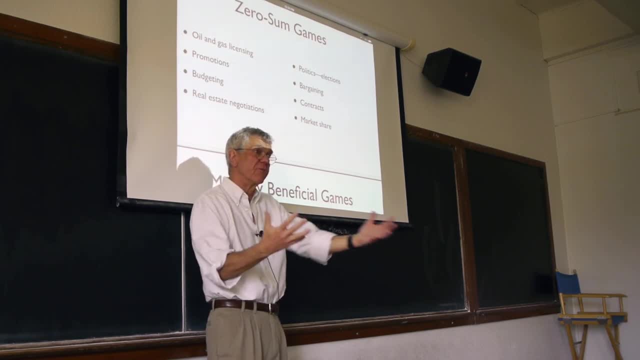 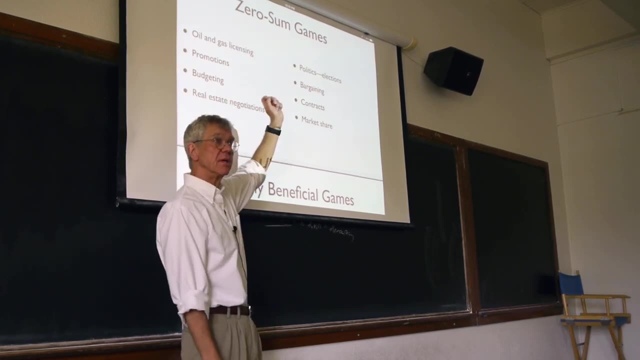 And you might say the amount of dollars remains fixed. It's just a question. It's a question of who gets what in the budgeting. That's how things more or less work at the university. Departments compete within their colleges, Colleges compete within the university. 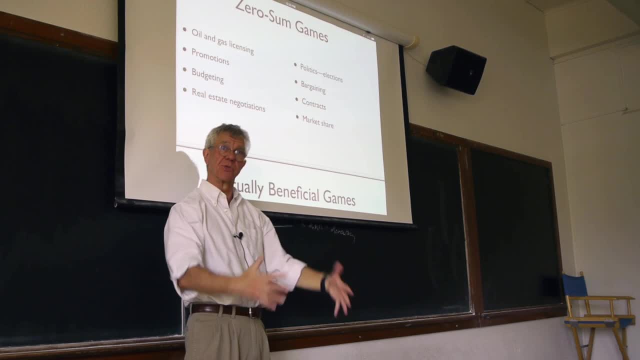 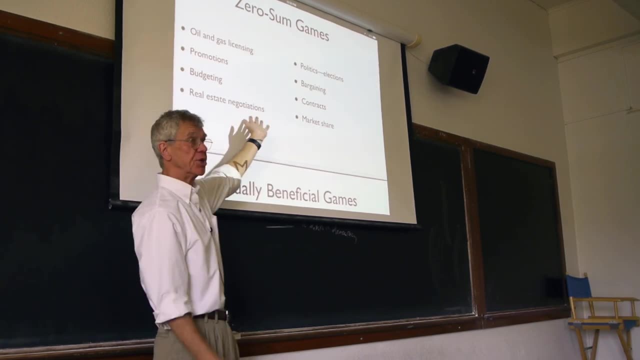 And it's really more or less a fixed sum that is coming in through tuition and legislative appropriations and other things, And then it's a question of where that money goes. Real estate negotiations are often like that: If I pay more for the house, you get more. Right. You can't get more for the house unless the buyer actually pays more. Elections are like that. if we think about percentages of the vote or, for that matter, if we think about seats in Congress, One party can only gain seats if other parties lose seats. 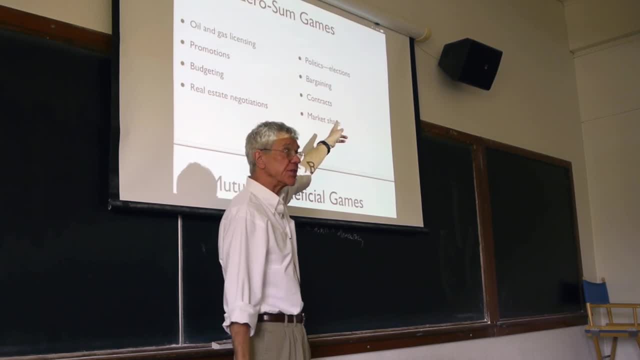 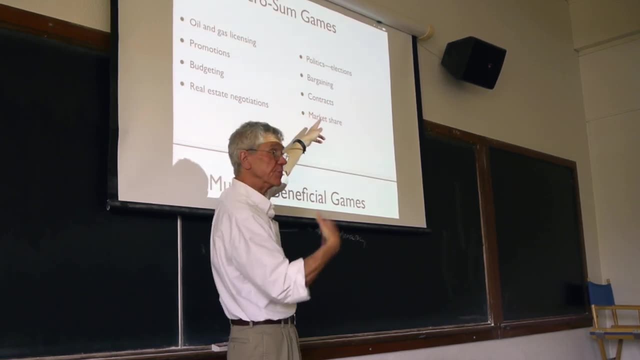 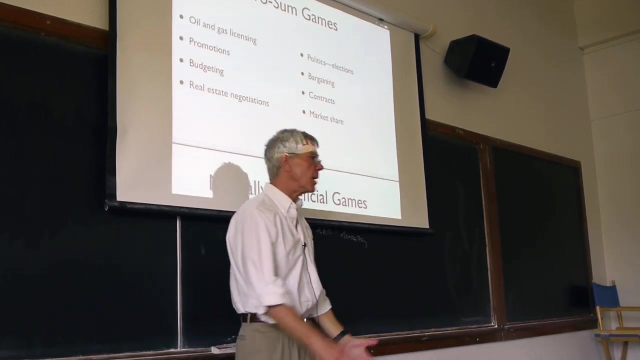 Bargaining is often like that. Say, we're bargaining over salaries, If you pay me more, then you have less Right. The salary amount I'm receiving comes out of someplace. Contracts are often like this. Market share is like this: 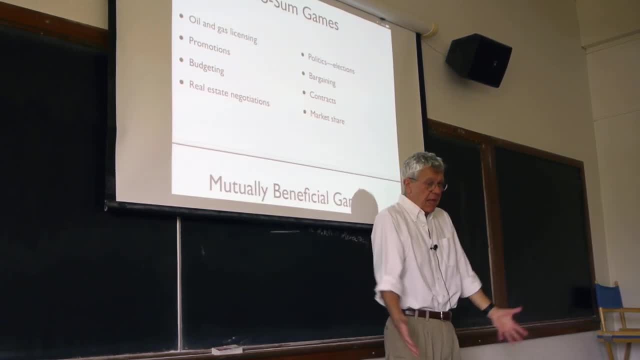 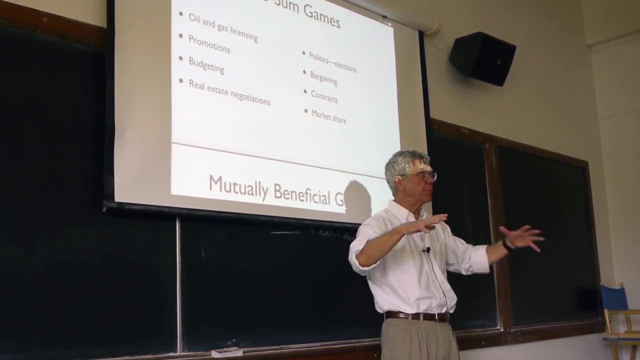 Companies are competing for market share. There's only a certain I mean. you might have more viewers on TV, say, or fewer viewers, So that pie can expand and contract. But if we're thinking of shares, well, if you increase your market share, 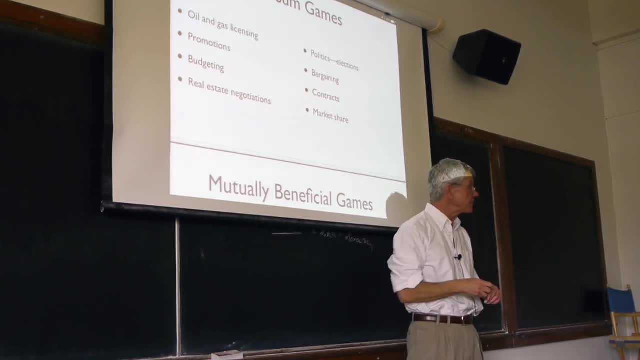 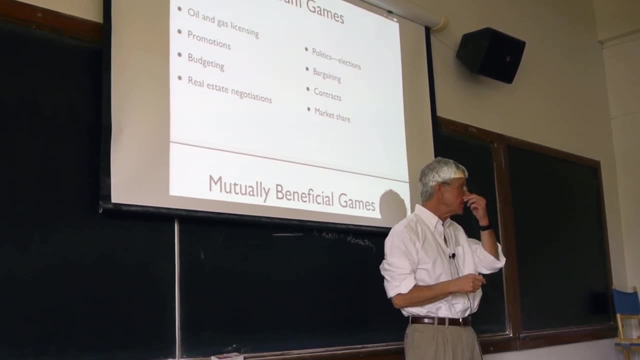 that means somebody else is decreasing their share. Yeah, It seems like a lot of these are really focused on economic side, like on money Right, For example, like the salaries. Maybe it's in a not in the money way, but in a beneficial. 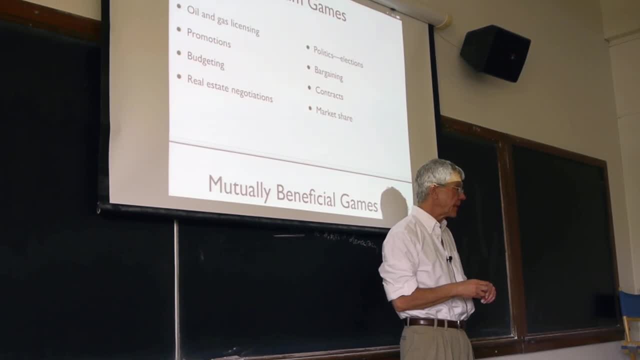 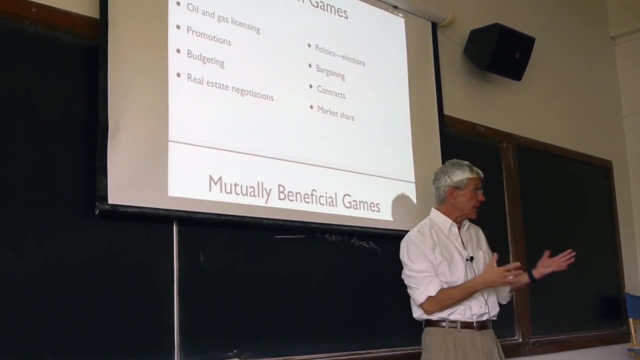 for both parties in a different way, like increasing productivity, perhaps, Right. So it seems like there's a lot of factors too Well, right? I mean, it's easiest to think of examples like this in economic terms. I absolutely agree. 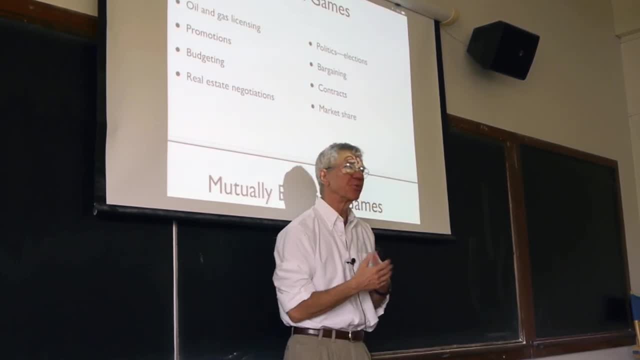 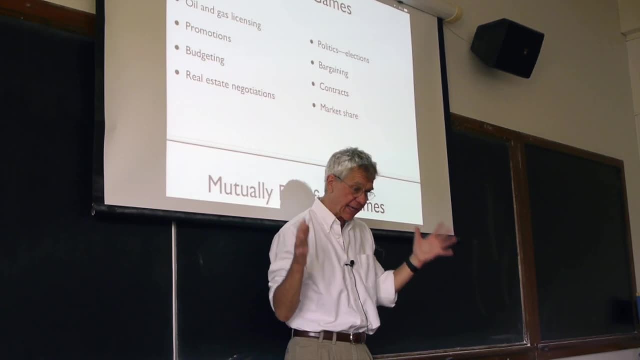 But think about: we don't tend to do this in liberal arts because we're nice, OK, But in some departments at this university, grades are allocated on a bell curve. Yeah, And then I might say, hey, 10% of the students. 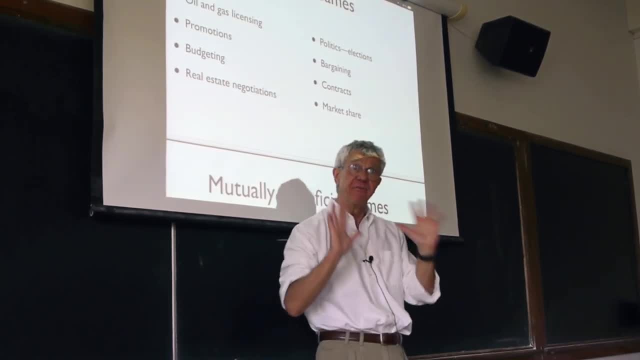 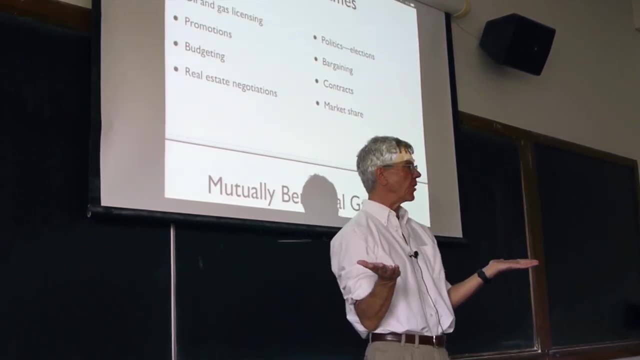 or 15% or whatever it is, are going to get A's. Actually, the toughest grader in liberal arts used to have this policy. He'd say: look, I'll give you an exam and it'll be entirely determined by how you do. 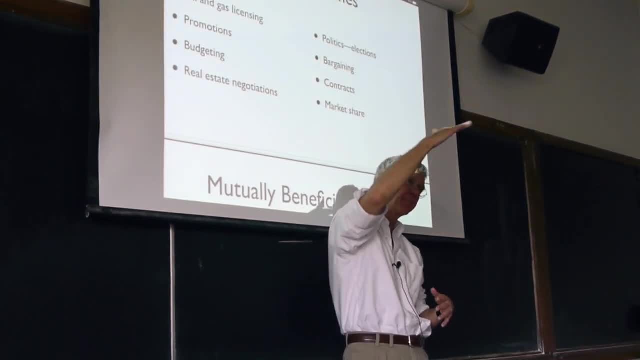 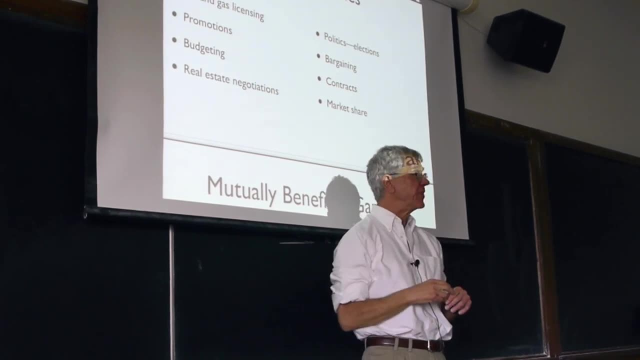 The person who does best on the exam, anybody who does within 10% of that gets an A, Anybody who does within 20% of that gets a B, et cetera. That turns out to be incredibly, incredibly stern. 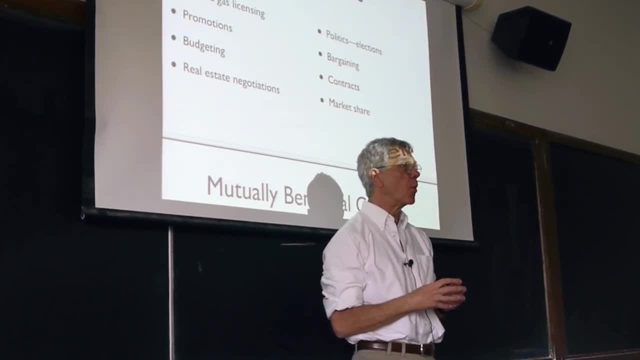 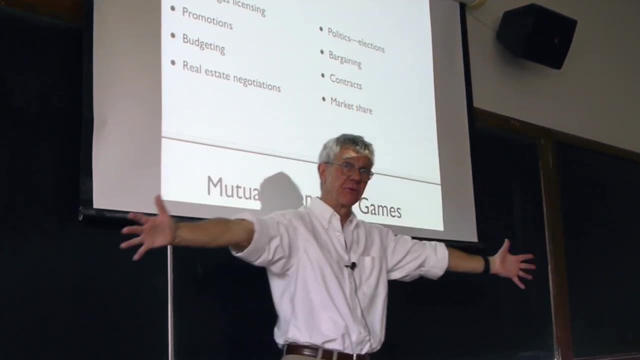 More than half of his students would fail. Now why is that so stern? Well, think about the way a bell curve goes Often in a large class, and he would teach classes of 500 people in intro psych- the very best student. 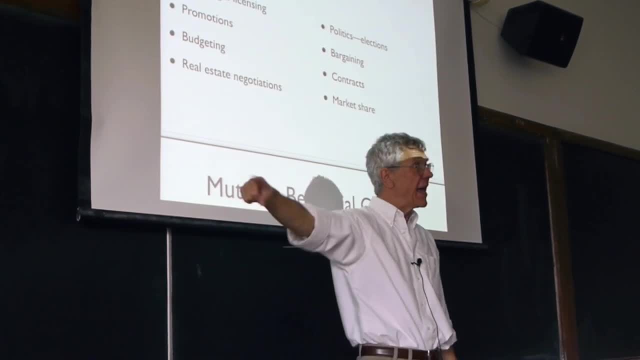 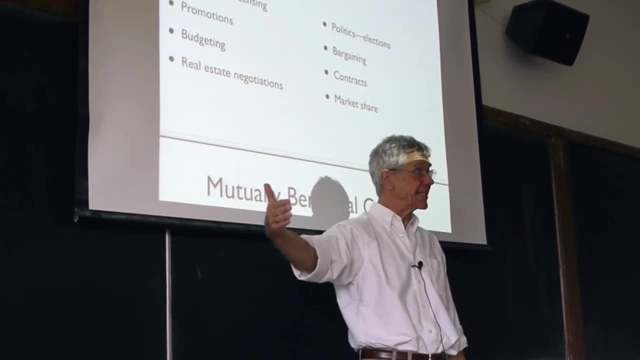 is often extremely good, right, And they're way out on the tail of the bell curve, Well within 10% of that score. Now, he wasn't saying 10% of the class, He was saying 10% of the score, right. 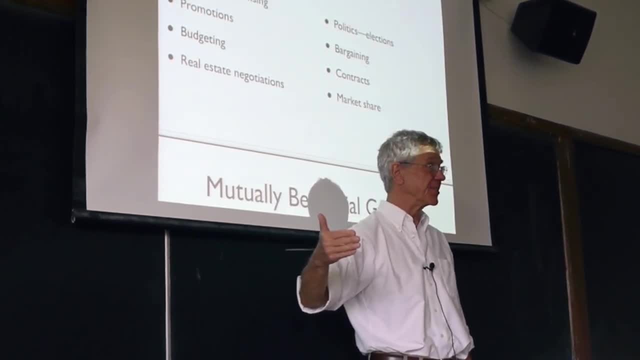 And it might be that only 2% or 3% of the students would fail, And then he would say: look, maybe 2% or 3% other people are within 10% of that highest score, which means only the people on the extreme tail of the bell curve. 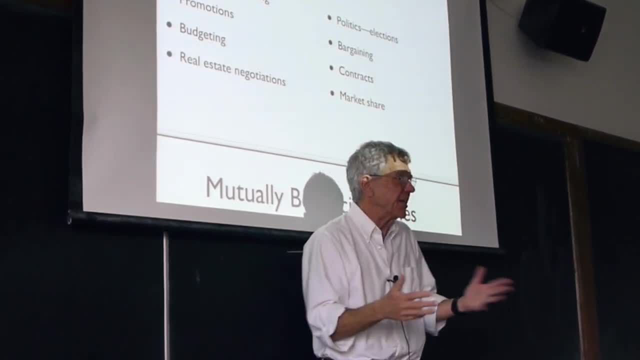 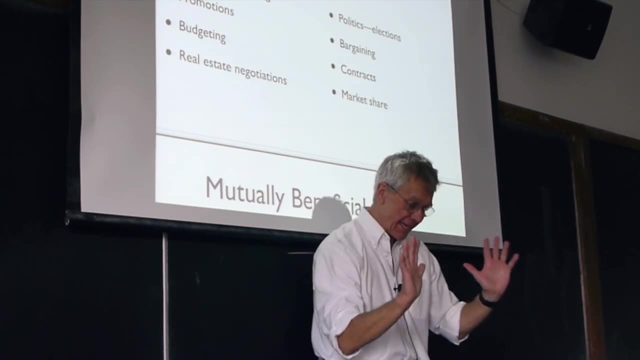 are getting an A, So, but anyway, that wasn't exactly a fixed thing. In a sense you could take the smartest person in the class and pay them off like make a few mistakes just for the rest of us. But in any event, suppose we don't do it that way. 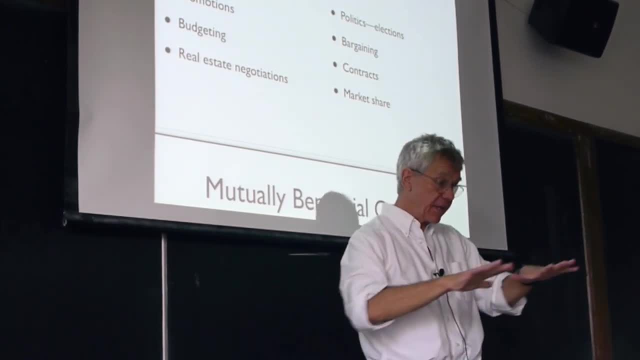 Suppose we say, yeah, 10% of the students will get A's Or for a while in liberal arts. actually the dean- a former dean- would say: I'm going to yell at you if you give more than 50% A's and B's. 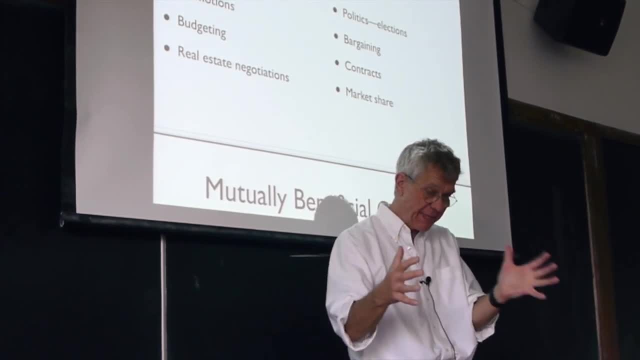 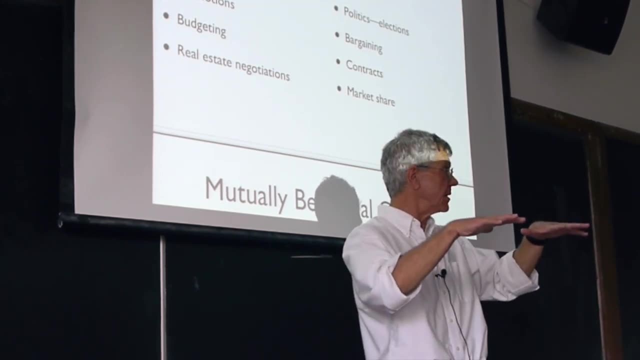 And in that case you might say: there's a fixed sum of A's and B's together that I can give out, And then it's a question of who gets them. But even if everybody in the class does better, it doesn't matter. 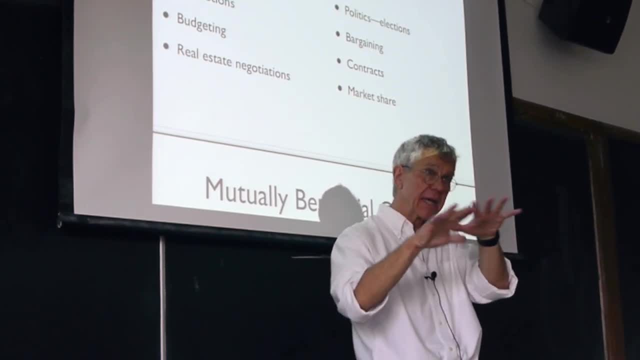 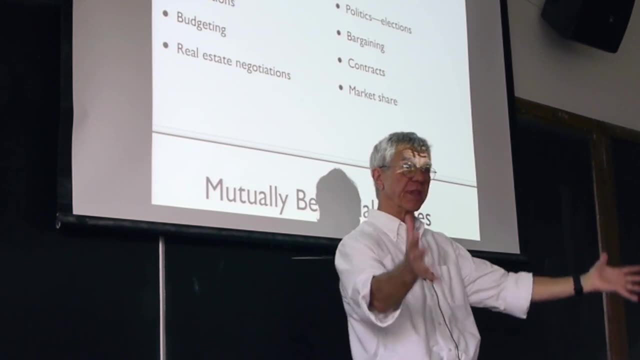 Only half the students can get those grades. So that would be a kind of treating of grades as a zero-sum game. Now, I don't do that. I mean there are classes like this one where the students are very good and lots of people. 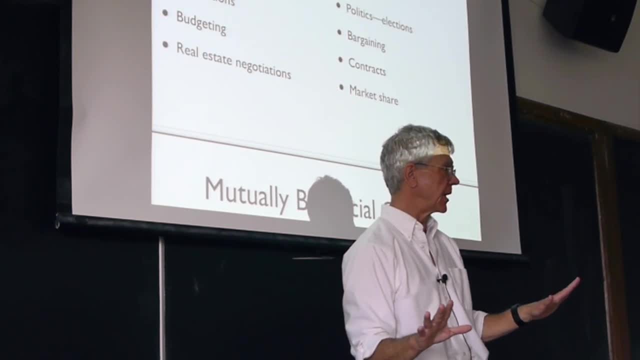 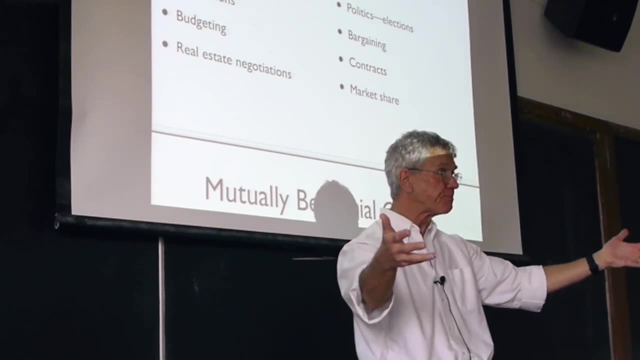 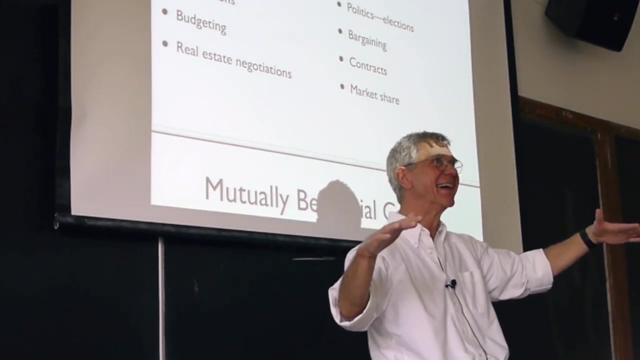 get very high grades. There are classes where people are terrible. In fact, talk about an instance of bad cooperation versus good cooperation. We have this program called FIGS, First Year Interest Groups. The advisors refer to the people in them as figlets. by the way, 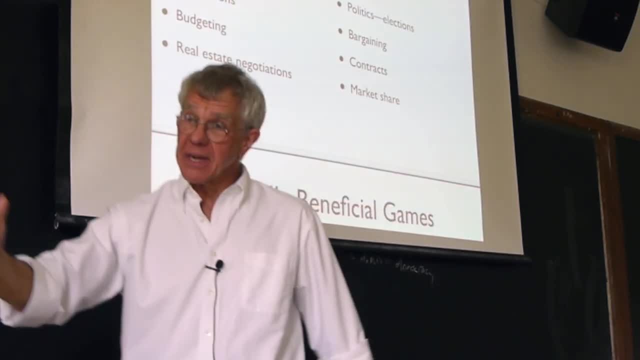 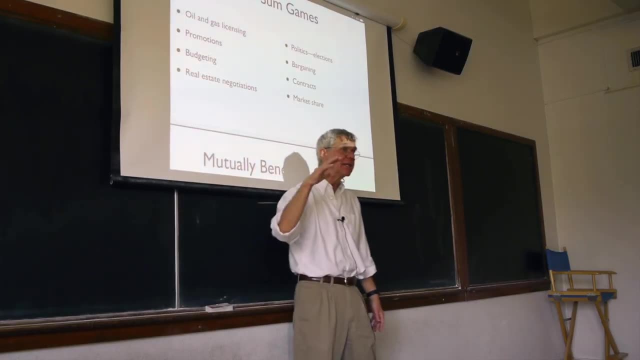 It is kind of cute. Anyway, the figlets. normally within those groups cooperation is very good And people in those perform better. But in the time I've been here I did have one of these where it was bad cooperation. 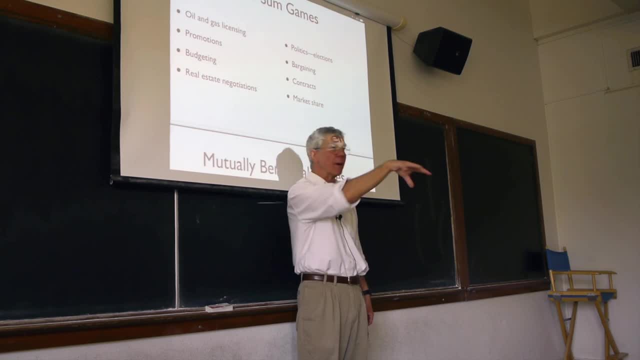 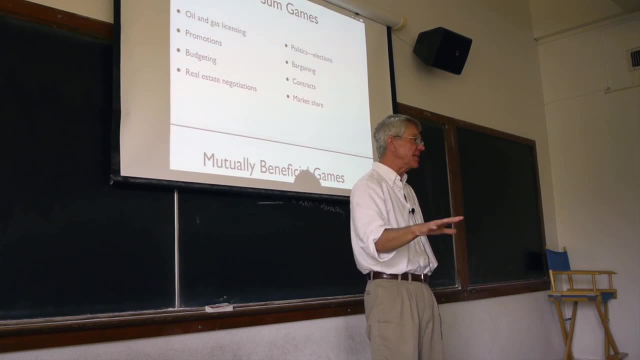 There were several people in there who were just terrible students and they corrupted the others. They all co-opted, So I think one person in that entire fig group got a C, All the others got Ds and Fs, And I don't think it's at the first. 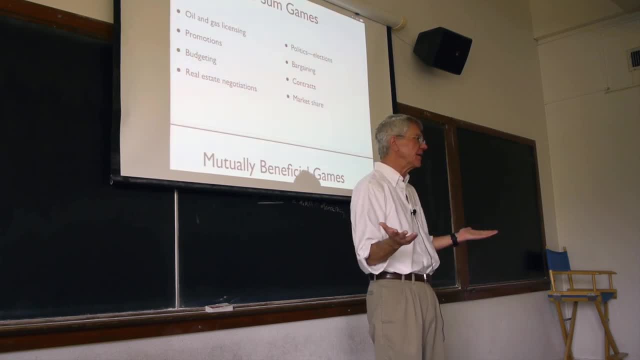 they didn't look like they were all terrible students, But it turned out the few really bad apples just spoiled the whole bunch and encouraged them all to have terrible work habits. So that kind of thing can happen. In any event, normally grading isn't like that, but it could. 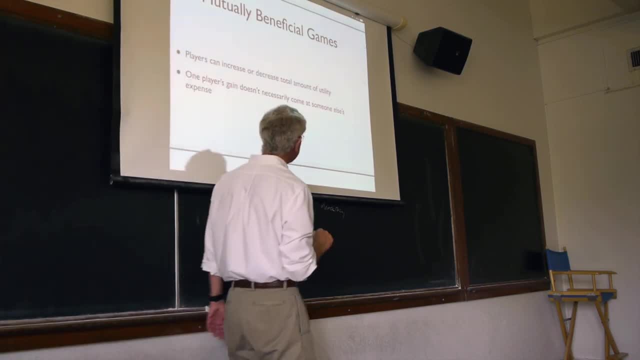 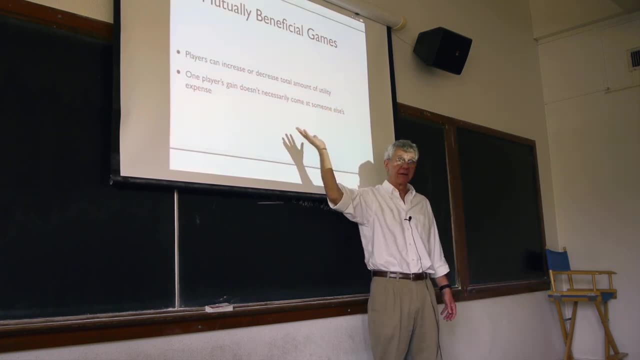 be, So it doesn't have to be economic. Now, lots of games are mutually beneficial in the sense that the players can increase or decrease the total amount of utility. So normally we would think war is like that. Wars can be fought more or less destructively. 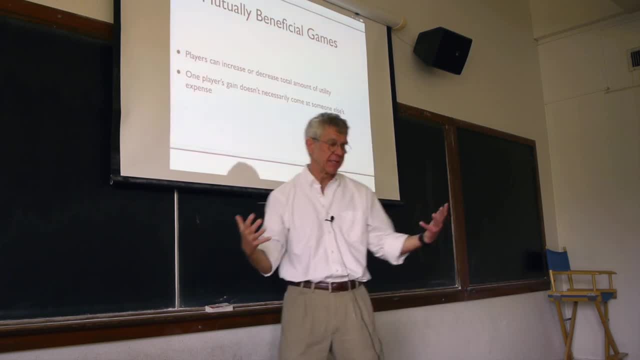 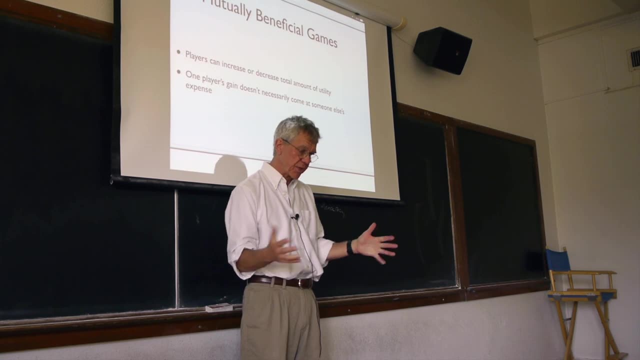 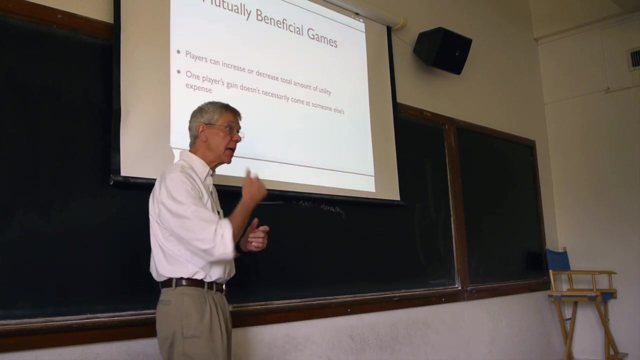 And in fact one of the hard questions in looking at 20th century military history is: why were 20th century conflicts so unbelievably destructive? The First World War, the Second World War, the loss of life, the destruction of property and so on just dwarfs earlier wars. Partly that's just because people had more technology to do more efficient killing. but it wasn't just that. And so you have to think, yeah, why were they such terrible wars? That was a case of people really decreasing utility radically. 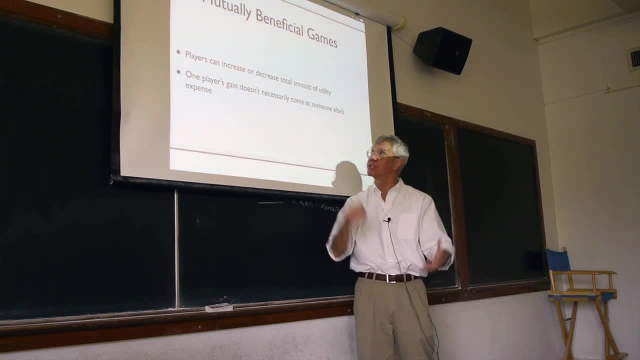 But also there are ways of people actually getting together and cooperating and increasing utility. Well, in this case, one player's game doesn't necessarily come at somebody else's expense. It might be, in fact, that I gain by causing you to gain. 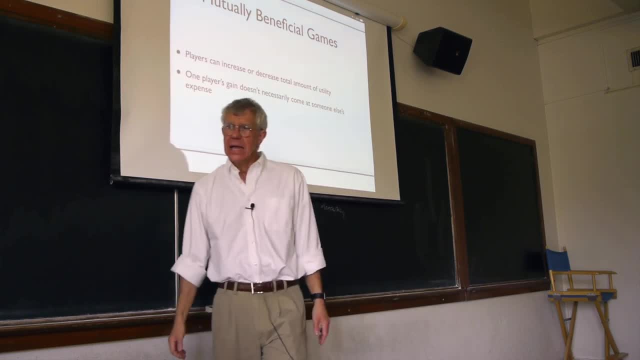 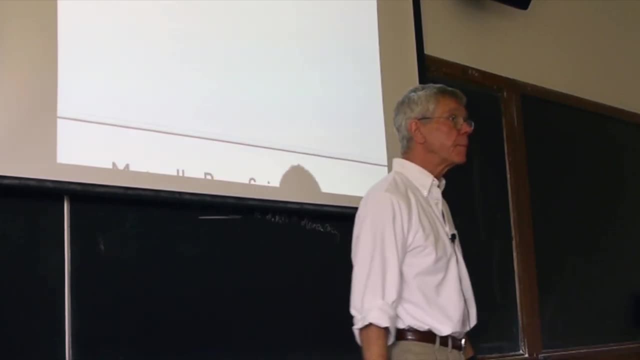 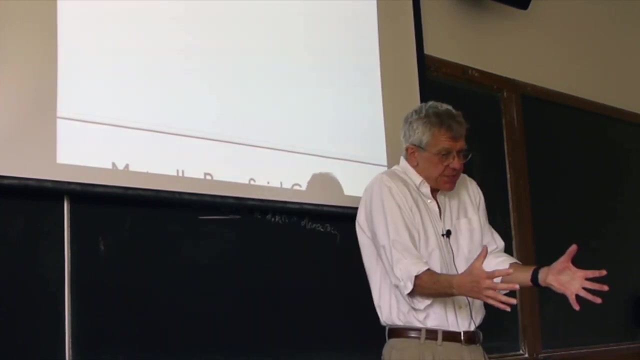 And so we actually have useful cooperation. So what are some examples of mutually beneficial gains? Economic competition, Good economic competition, You might think. well, if we're thinking market share, my getting more market share means you have less, But on the other hand, it might be: 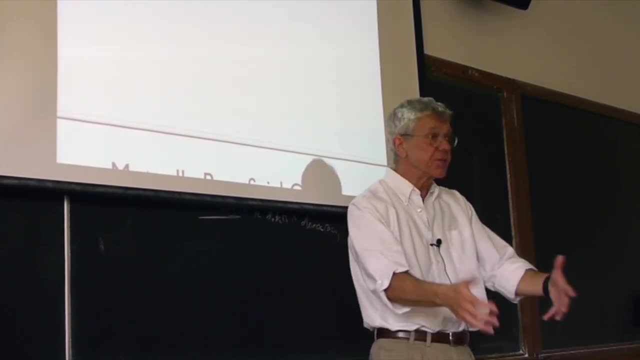 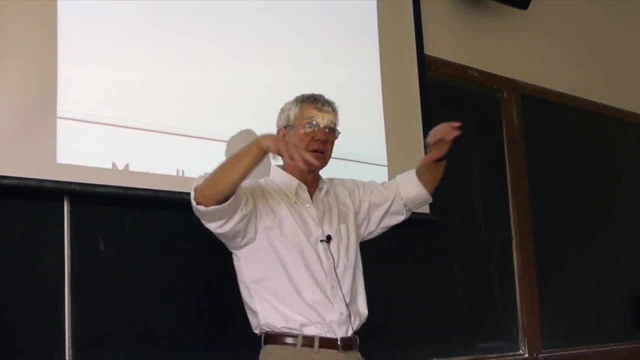 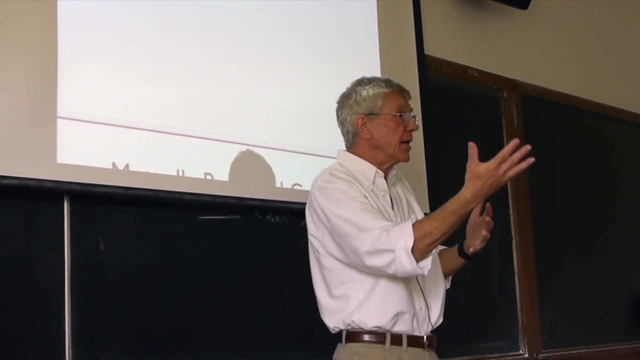 that actually, by introducing new products and competing, we're actually increasing people's interest in all of this, And so we're growing the market at the same time. So maybe the competition is actually improving all of our situations, And similarly, I sell you some product and you like it. 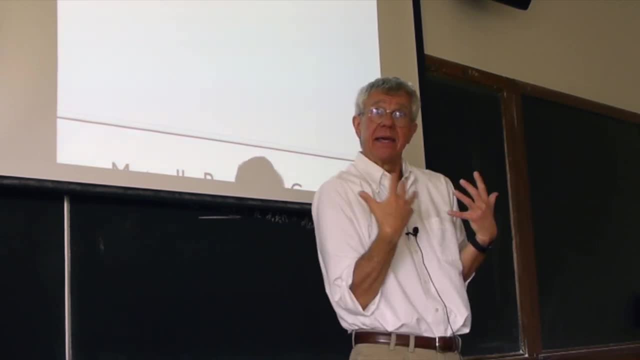 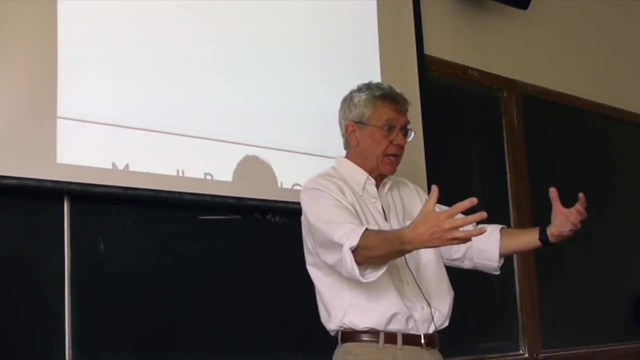 It makes your life better. I'm improving your utility. Meanwhile, you're paying me, so I'm getting a benefit out of that, And so we're both benefiting. In fact, typically in an economic exchange, that's how it goes. 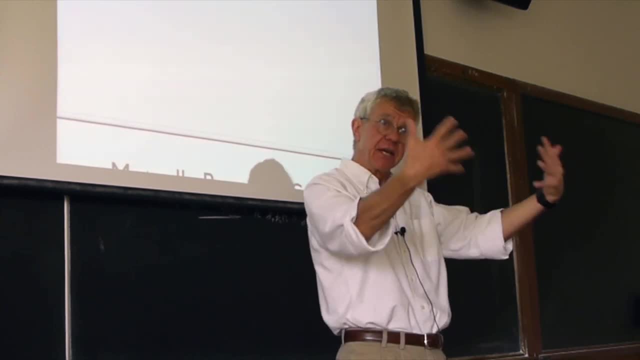 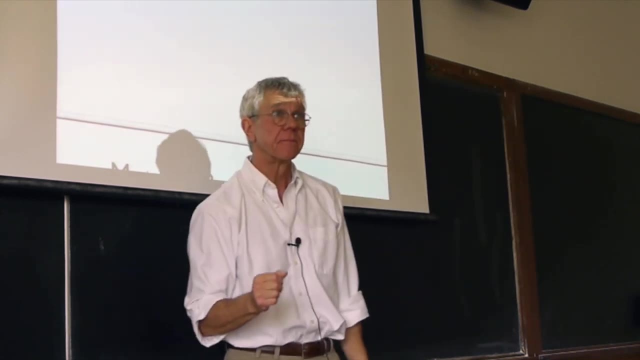 You agree to it because you're better off, And this person agrees because they're better off, And so the exchange actually makes both parties better off. Other examples: Yeah, Education, Education, good Education is something that generally makes people better off. 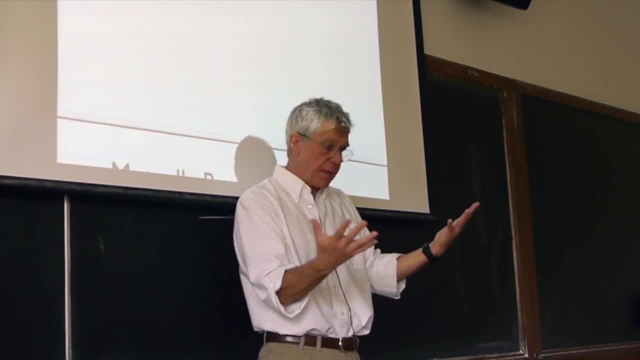 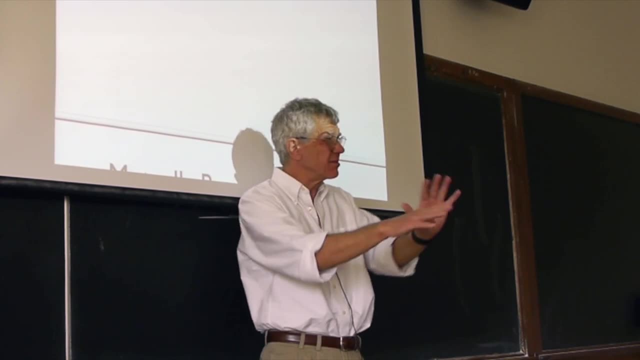 And so you might say: when a professor does the job well, the professor is better off, but also the students are better off. A teacher who does a terrible job, the students don't learn anything. the professor, I assume, doesn't feel good about it. 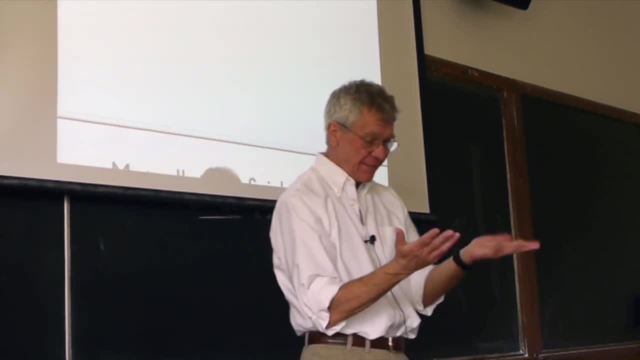 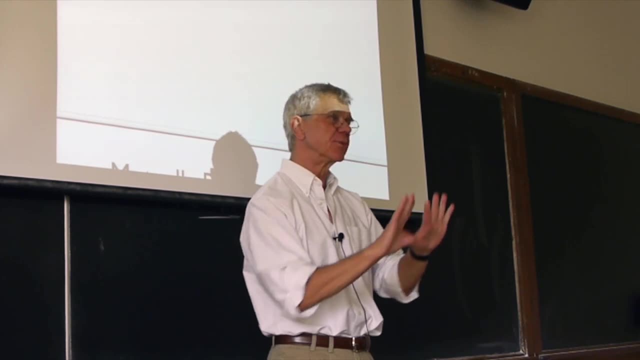 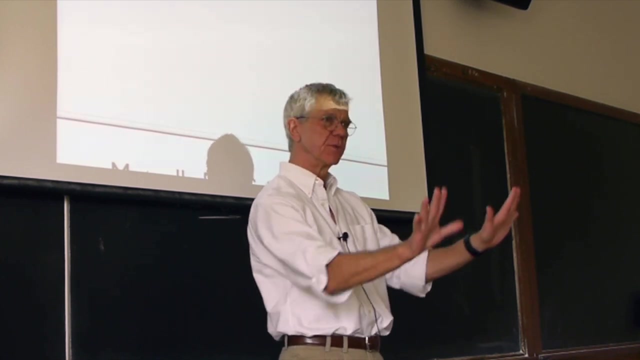 I wouldn't know, of course. Well, yeah, Think about the worst teacher you've ever had And don't tell me if it's me, But think about the ways in which that can be worse for the students, but also for the professor. 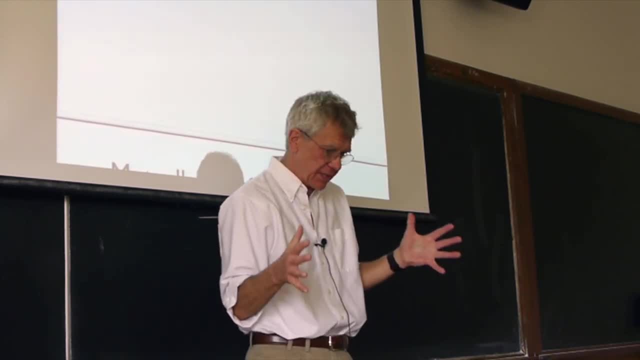 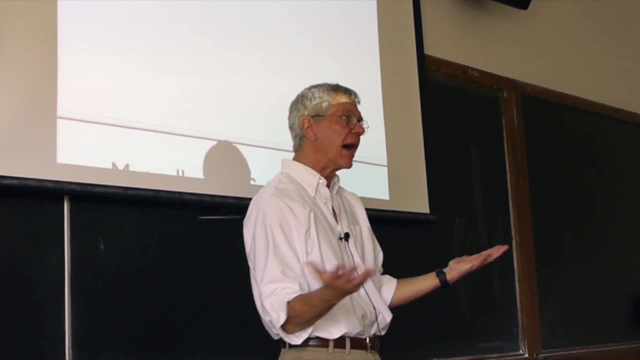 Even within a class, holding the professor constant, as it were. sometimes the group of students in a class add to each other's learning a lot, and other times they don't. I've taught ideas of the 20th century, sometimes with really good students who make comments that are terrific. 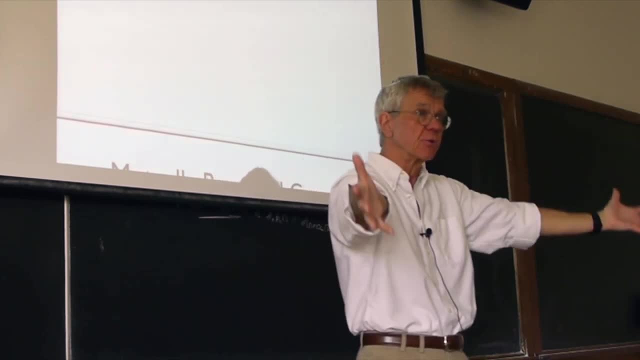 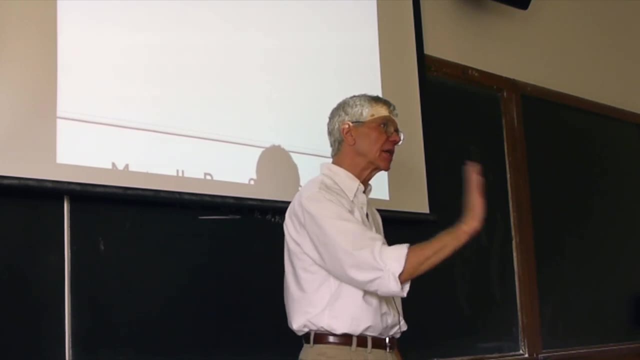 and get everybody else more involved, more excited and people in general do better. I had one class where there were two people who sat in the front row and every question I asked, the class responded with some stupid joke, And it was stupid. 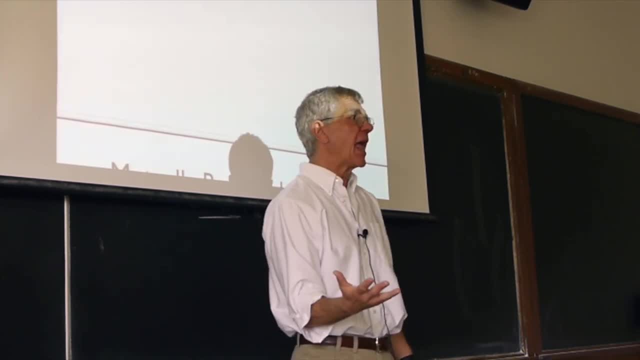 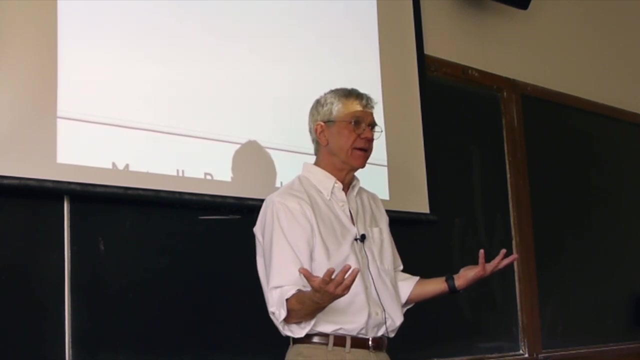 I mean it wasn't funny, but they always did it. And so you ask a question like: why were 20th century wars so destructive? And this is mental. It's meant to encourage a good discussion And if the first people to talk say something stupid. 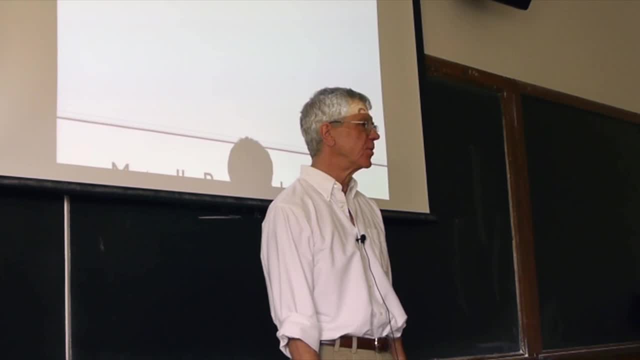 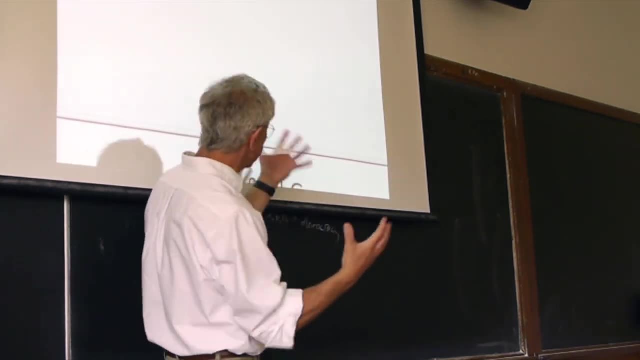 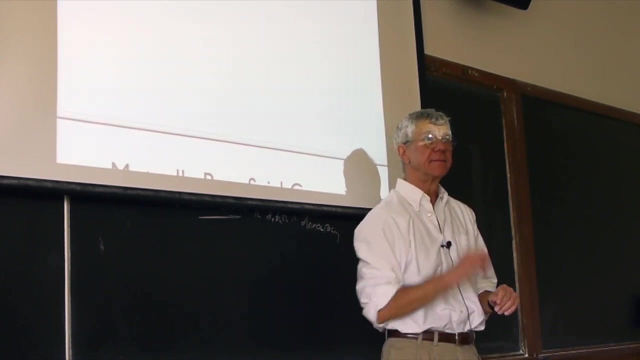 then it's kind of like: well, now the whole discussion kind of goes off the rails, So anyway, the group can act in a way that improves the group's outcomes or decreases it. Other examples: Yeah, The conformity to laws. Good conformity to laws if we all conform. 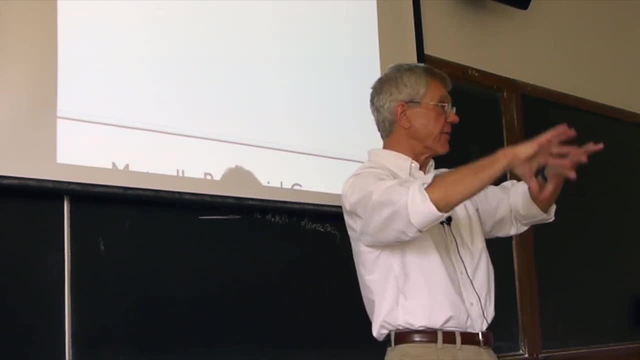 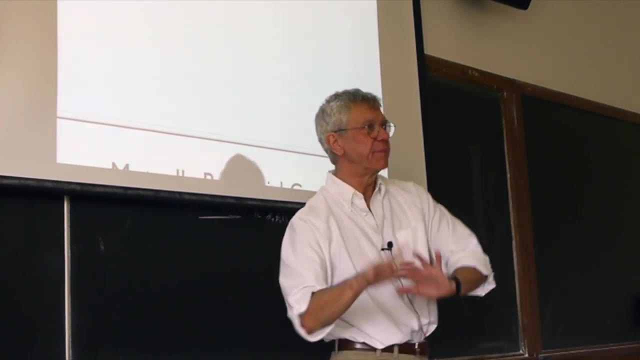 to a certain law, and it's a wise law at any rate, then it looks like everybody benefits from that. But we can also start breaking that law and that maybe makes other people more inclined to break it, and so people's behavior can make people worse off too. 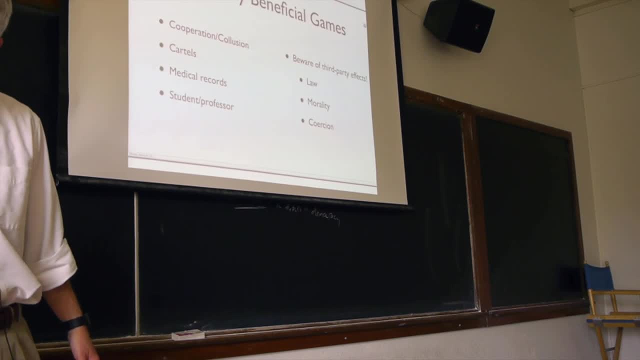 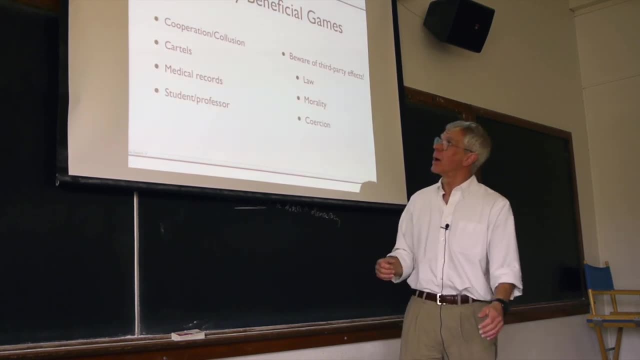 OK, well, there are lots of examples of this. It's easier than zero-sum examples. So lots of cases where people cooperate or, for that matter, collude. That's sort of a bad form of cooperation Cartels we've mentioned. 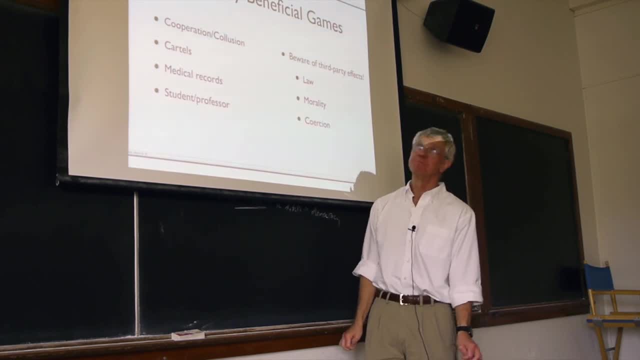 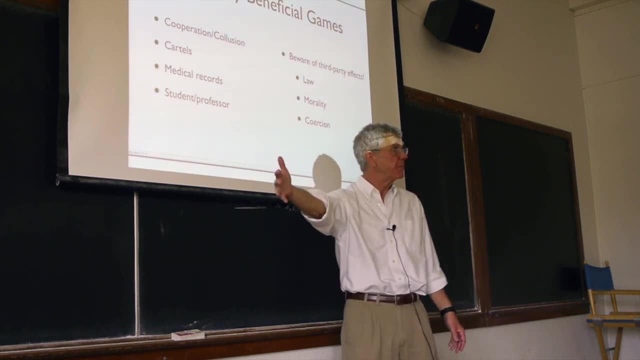 Medical records. Somebody came up with this example to this one time. It may be that if we have a system of keeping medical records, that's highly effective. it helps make people healthier because doctors have the information they need, Nurses have the information. 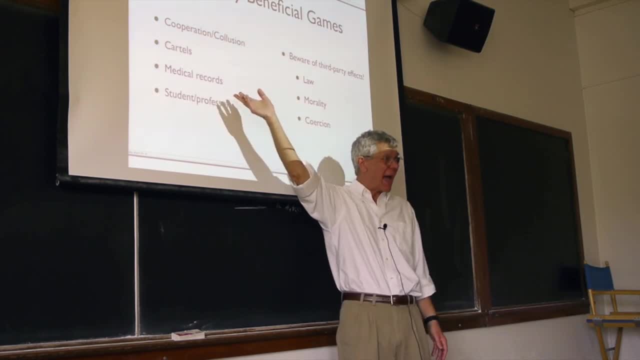 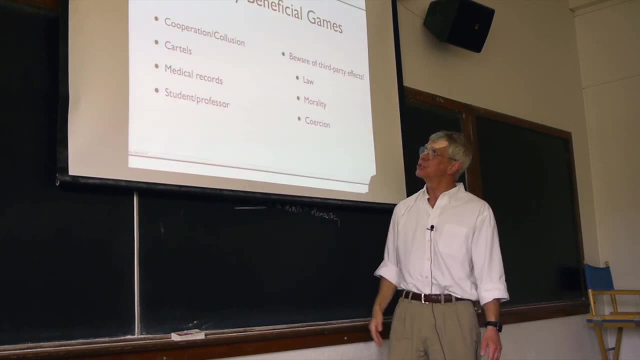 Everybody puts it in and such. On the other hand, you could have a system of doing this. that's bad, either because it's misleading or because it takes up so much of people's time that they don't have time to actually treat patients. 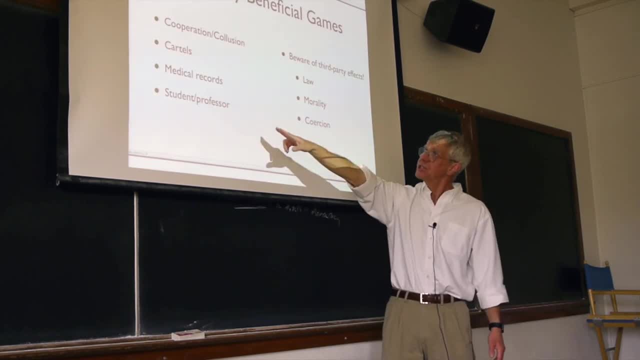 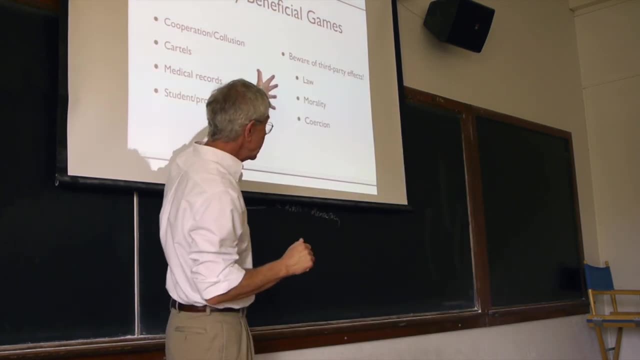 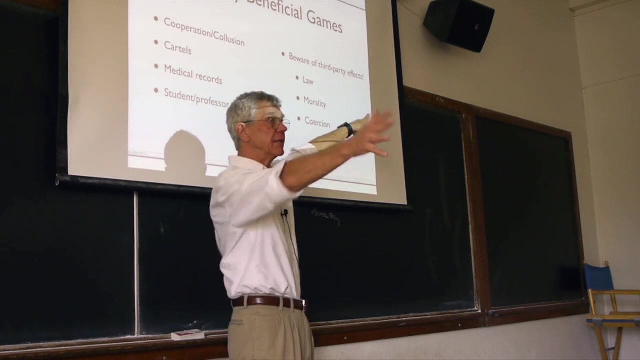 et cetera. So that can make us all better off or worse off Student-professor interactions. But do beware of third-party effects, because sometimes people can affect the behavior of others in ways that are unexpected. A lawbreaker, for example, might not only let's say: 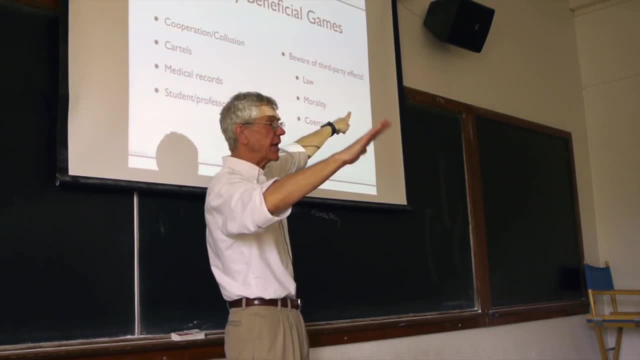 steal somebody's property and create harm in that way, but might create all sorts of other harm. All of a sudden the rest of us start getting worried. It upsets us. We think, oh, we're in some danger too. 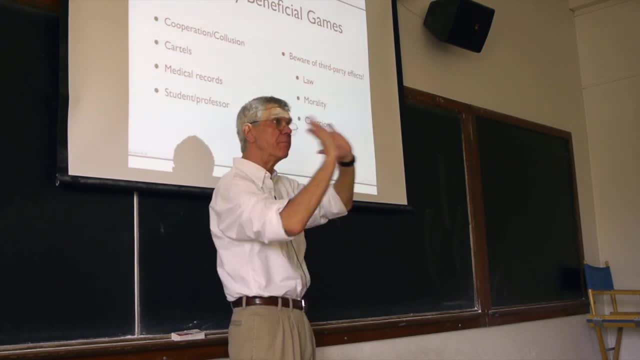 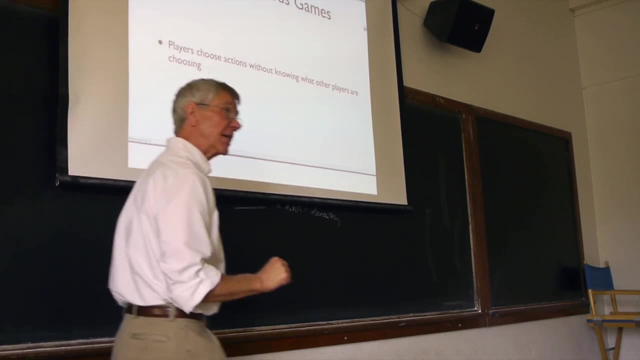 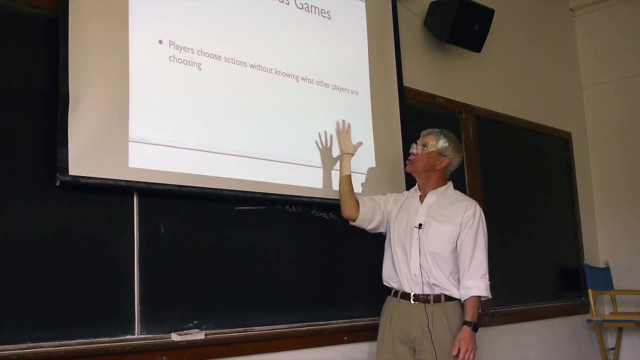 We start having to buy locks, security cameras et cetera. There can be big costs imposed on third parties. Now let's talk about that other distinction between simultaneous games and sequential games. So in a simultaneous game, players are choosing actions without knowing what the other players 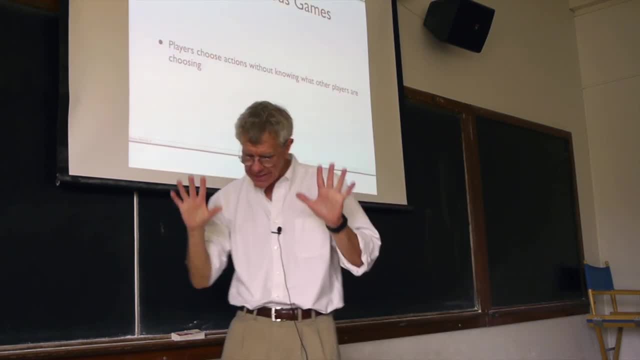 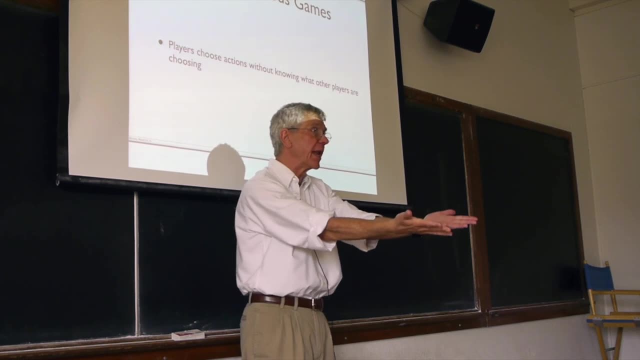 are choosing. So I have to make a decision about what I'm going to do, And I don't yet know what you're doing. We have to make our decisions at the same time, And then we see what happens when we put them together. 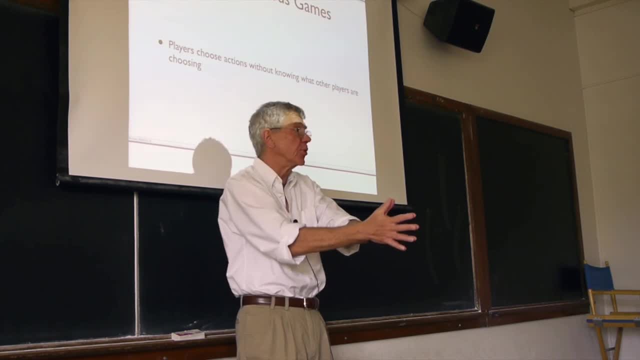 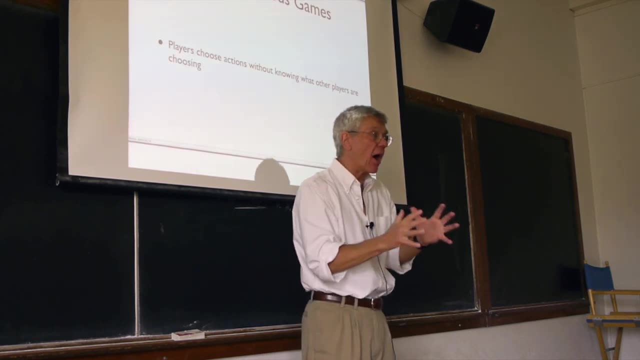 But you act in ignorance of what I'm doing. I act in ignorance of what you're doing Now. we might know the history of what we've done in the past, But in terms of the play we're making now, we have to play at the same time, as it were. 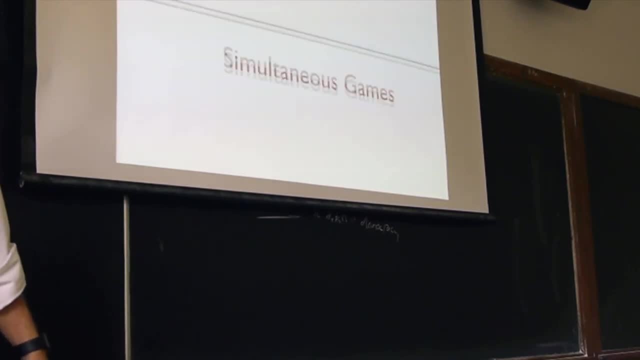 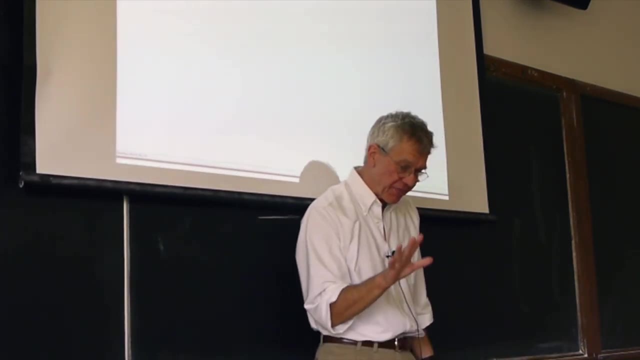 without knowing the other person's play. So what are some examples of simultaneous games? Yeah, Prisoner's dilemma. Ah, yes, a prisoner's dilemma. We're going to be talking about that a lot next time, But the idea will have to be the prisoners. 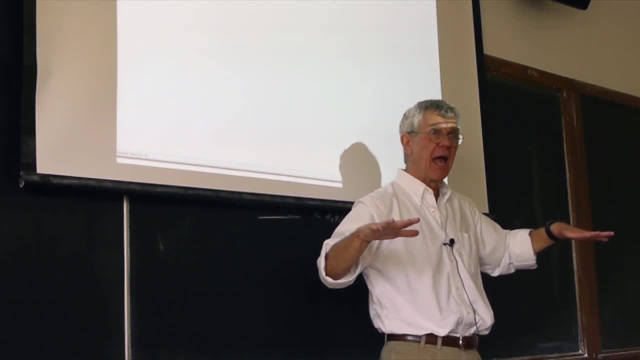 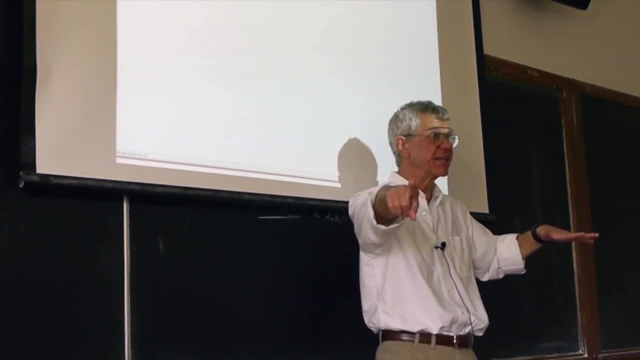 are taken into separate rooms and questioned by the police, And you have to make a decision. How much information do you reveal about things And do you, in particular, give evidence against the other person in the other room? And that is something you have to decide. 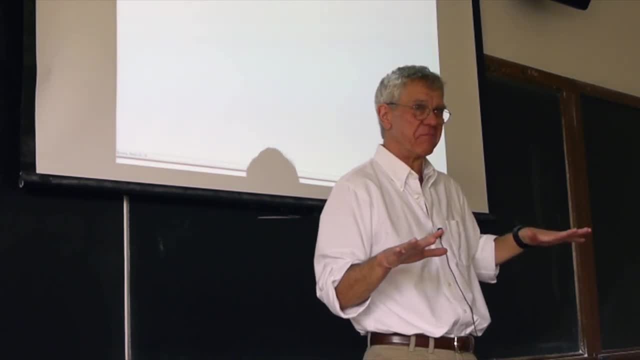 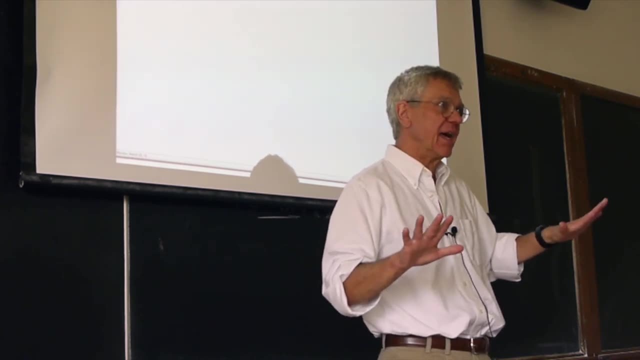 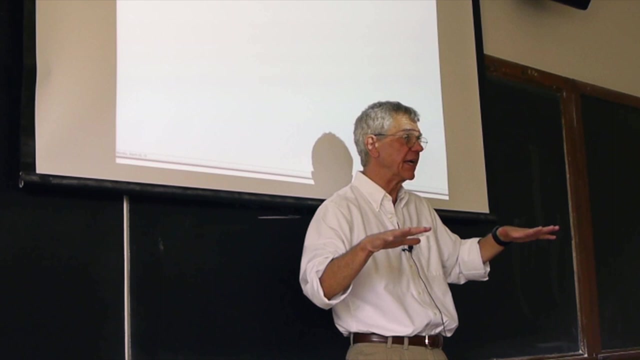 without talking to your fellow criminal in the other room. The police really do this kind of thing. They normally take people into separate rooms and question them separately, both to try to trap them in lies but also to give them increased pressure to confess and implicate. 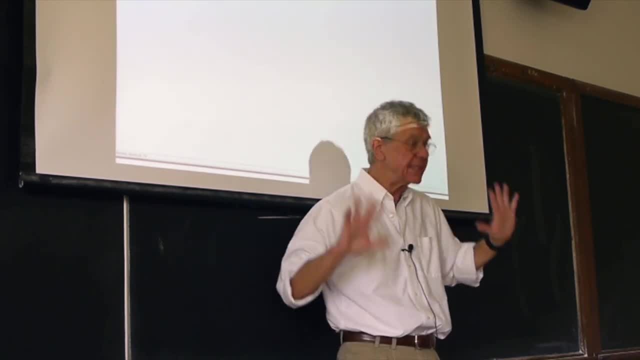 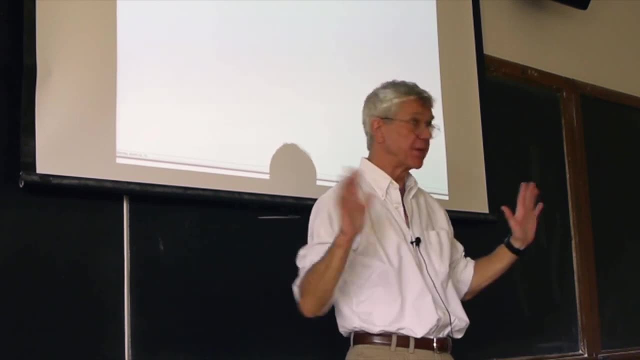 the other person And again, we'll talk about the details next time. But yeah, that's a case where you have to decide what you're doing without knowing what your fellow prisoner is doing. It'd be something totally different if you're there in the room together. 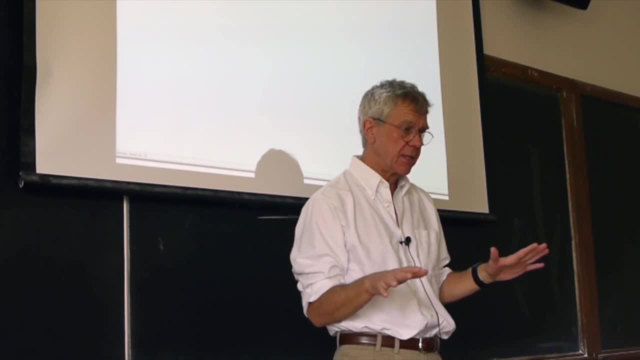 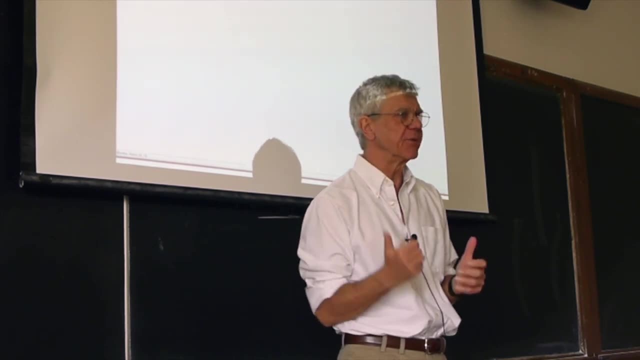 and you can kind of confer, But in this case you can't. I did have a student one time who said after class when we talked about this: I've been in trouble a lot with the law. This is exactly what they do. 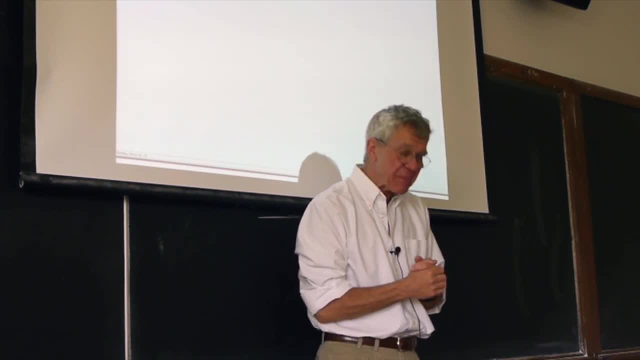 They put you in a prisoner's dilemma. That's why it's called that. Anyway, other examples of things we're going to talk about. There are things where you have to decide what to do without knowing what the other person involved is doing. 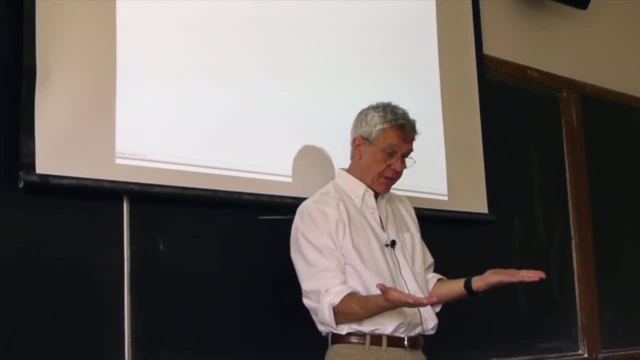 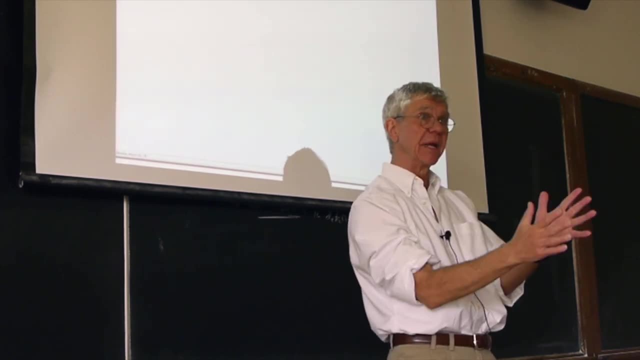 Yeah, Stock market, Good stock market. You decide whether to buy or sell the stock And you can look at the history and know what it's been doing, even in the last few minutes. But you don't know who's going to be. 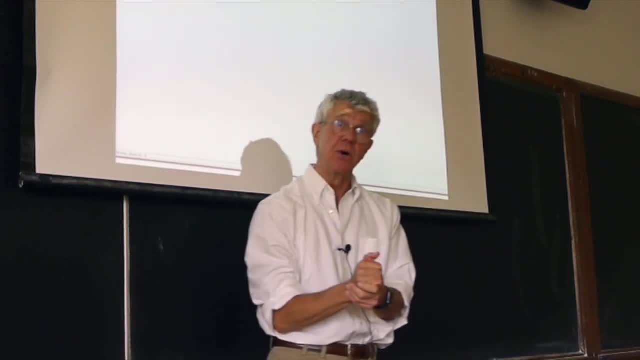 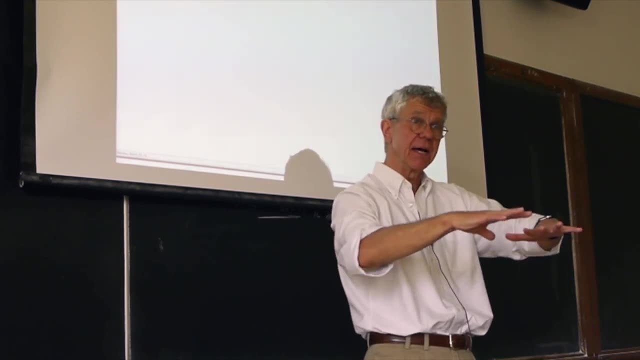 willing to buy or sell at that moment that you make the decision, And so the stock market is something that is like this: You make a decision and other people are deciding on buying and selling at the same time, And you aren't quite sure how that's going to come out. 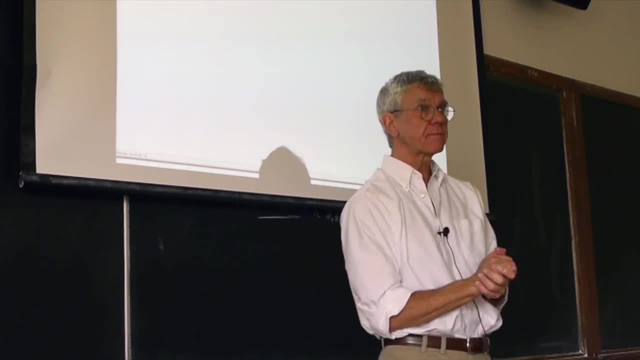 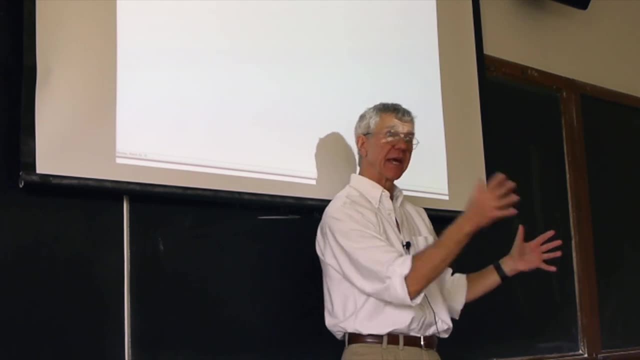 Other examples: Yeah, College applications. College applications can be like that. Yeah, it depends on the system. Now some colleges have rolling admissions And so that can be different. You can apply to a place, find out. oh, I didn't get in. 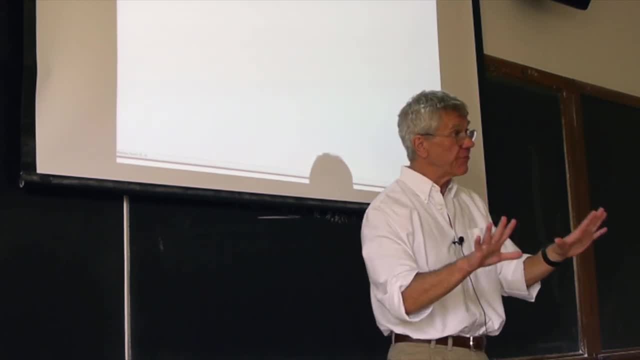 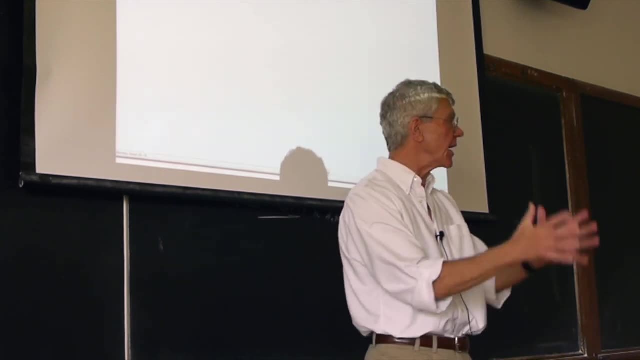 I think I'll apply to this other place. But yeah, the way it often goes, there's a certain deadline And you have to submit all the applications by more or less that deadline, And then there's a certain time you hear from them all. 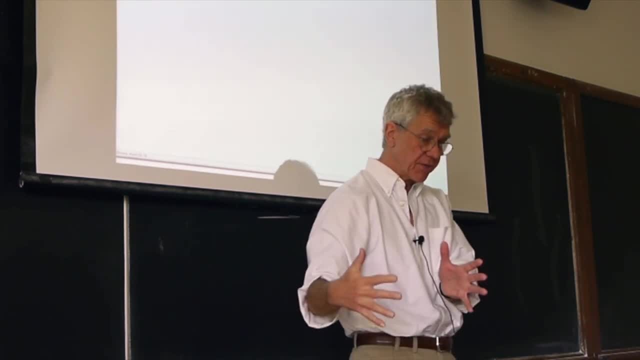 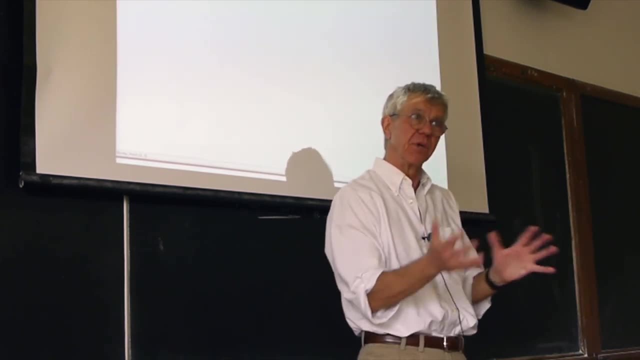 And at the time you're applying, you don't know what's happening with others. And then, when they announce their decisions, they don't know what those people are going to do. So, yeah, when it's done that way, it really looks like a simultaneous game. 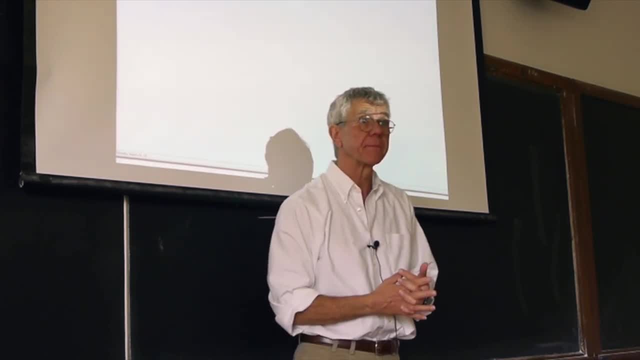 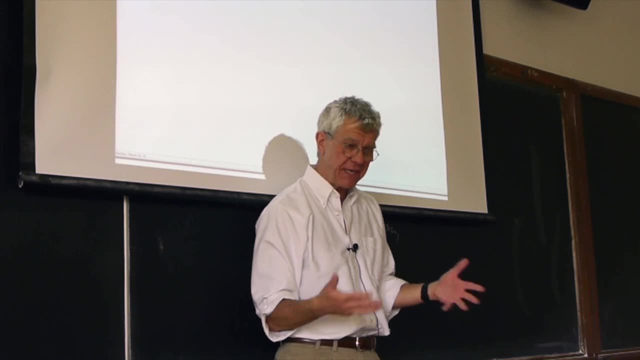 Other examples: Yeah, With reality TV, there's like game shows and stuff where people OK, good, Yeah, a lot of TV is based on this kind of thing, where you have to decide on a strategy, Somebody else is doing it. 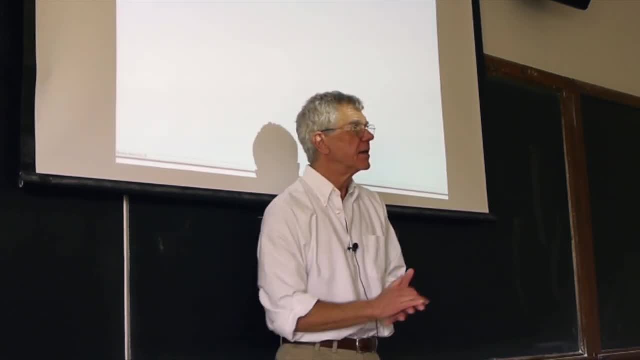 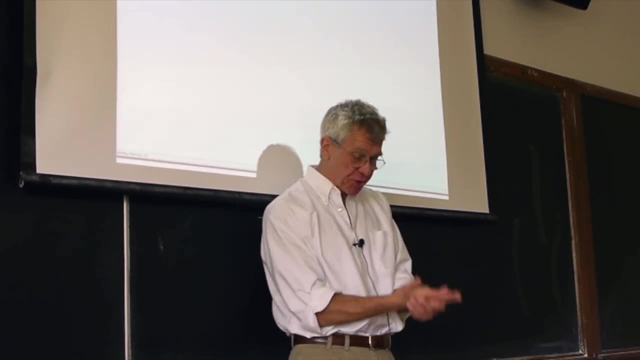 You can't see what happens until you put them together. Yeah, Good, reality TV always has collusion happening. That's something which happens in simultaneous games, That's true. yeah, I mean imagine. well, actually, if you've ever watched The Survivor Show, there's. 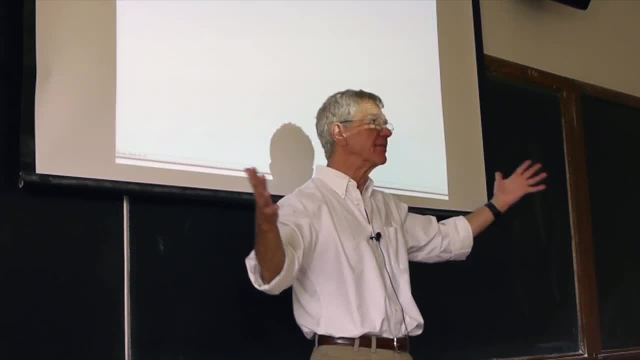 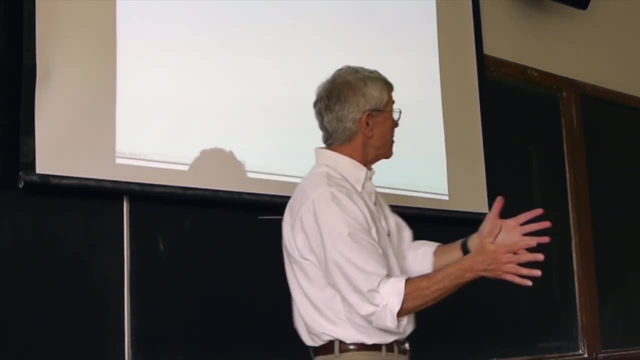 a huge amount of coalition forming and collusion going on, Until, of course, it gets down to the last two, And then it's like there's nobody else to collude with, And so then it can look more like a simultaneous game. 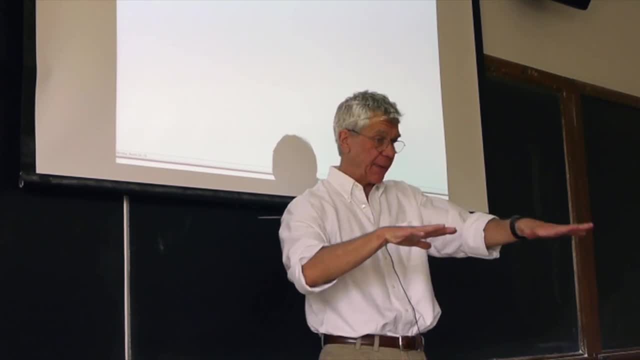 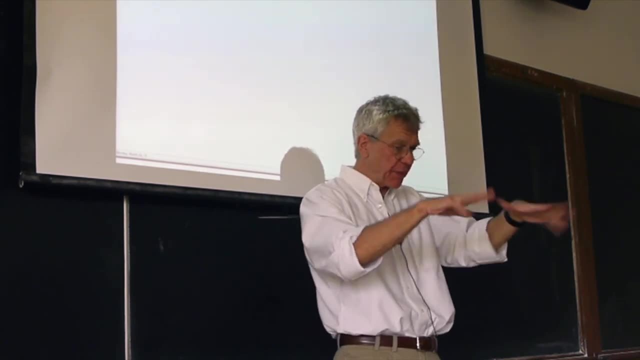 But you're right. until then, there's all this collusion happening And that is going to complicate these pictures a lot. In fact, often in game theory, what we'll do, just because we're looking at it at an introductory level. 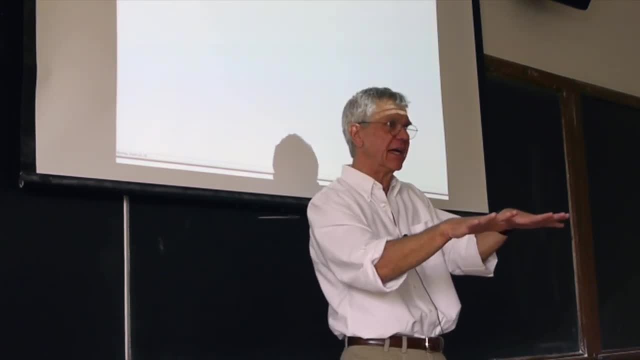 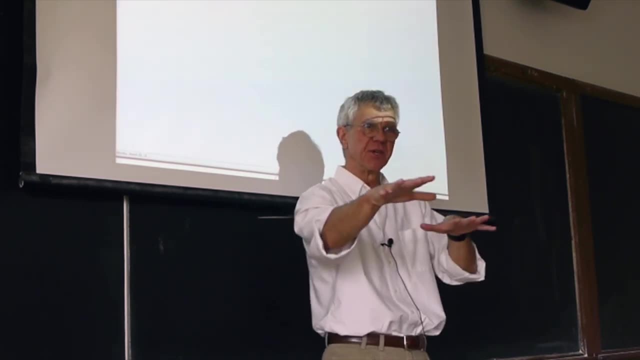 is looking at two players, So we don't have to worry about the collusion part. But you're right, in real complex situations with lots of players, they're forming coalitions with other parties and so on. Think about a European-style democracy. where actually taking control of the government isn't a question that any one party can do on its own. You have to form coalitions with other parties. That can make things a lot more complicated, And then it can be much more well. it's interesting. 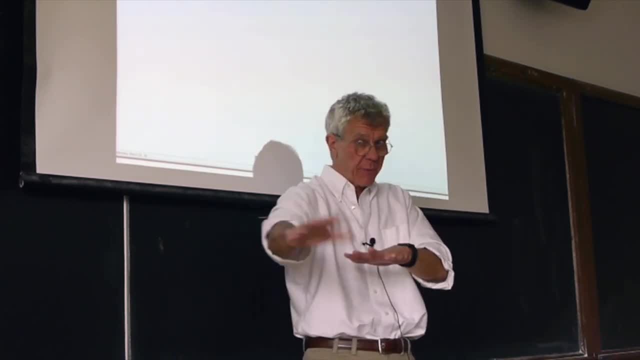 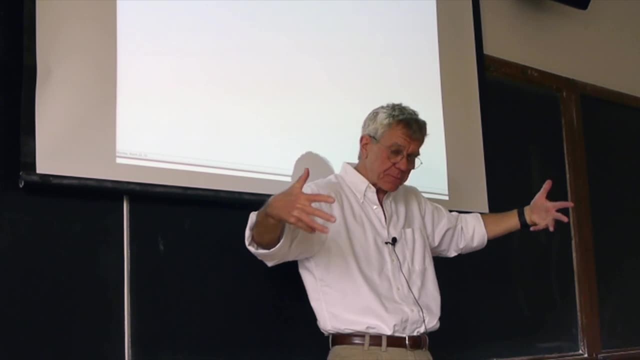 Yeah, sometimes that becomes more sequential because you form a coalition with that party and then this party scrambles to form a coalition with that one, But sometimes it can really be simultaneous. You walk into the vote and you see how the vote goes. 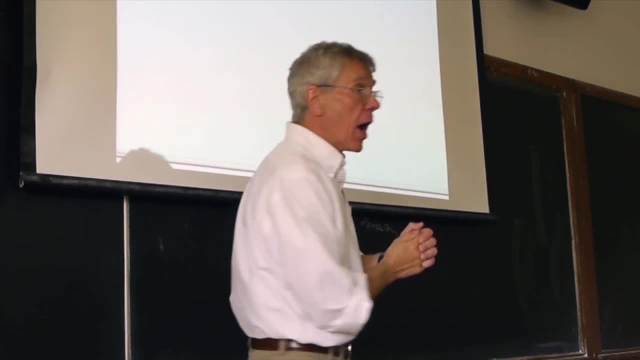 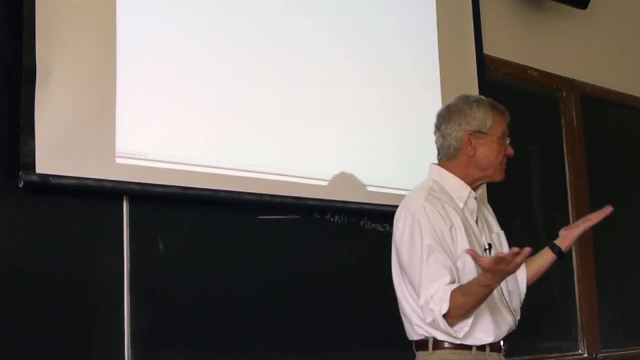 And it can all be happening at once. Other examples of this: Yeah Life, Yeah good Life is often like this: right, You don't know what other people are doing At the same time. you have to make your commitment. 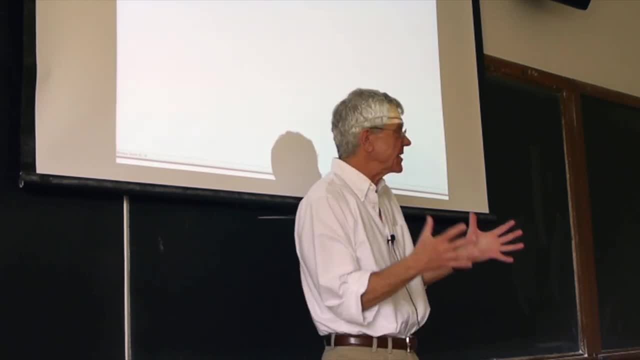 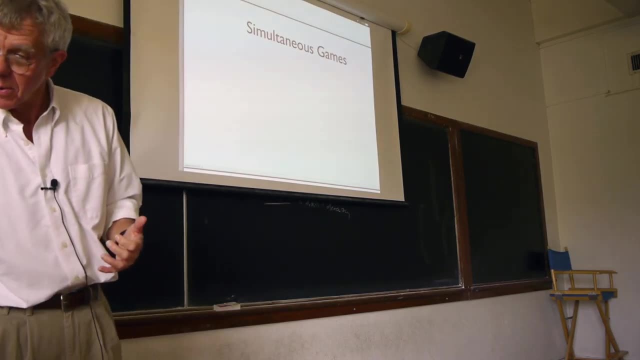 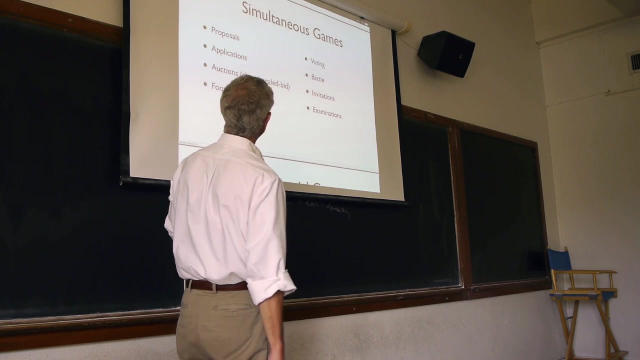 And so that's I mean in a certain sense, you face situations like this every day, And that's part of what makes life complicated: You have limited information. Here are some examples I was able to think of: Sometimes: proposals- People submit proposals. 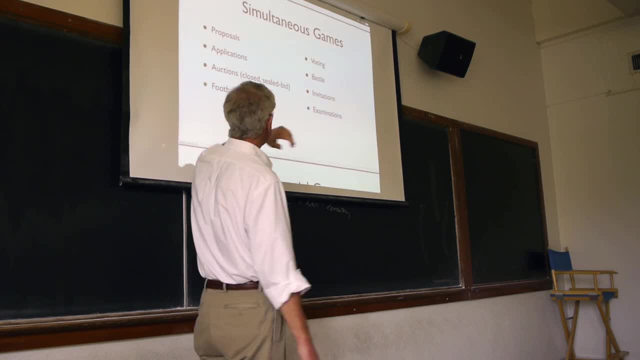 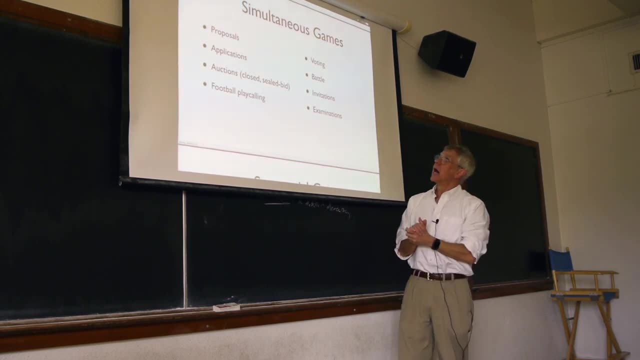 Let's say for grants or for projects or other kinds of things, And a bunch of other people are submitting proposals at the same time. You don't know what they've done. They don't know what you've done. Submitting college applications can be like that. 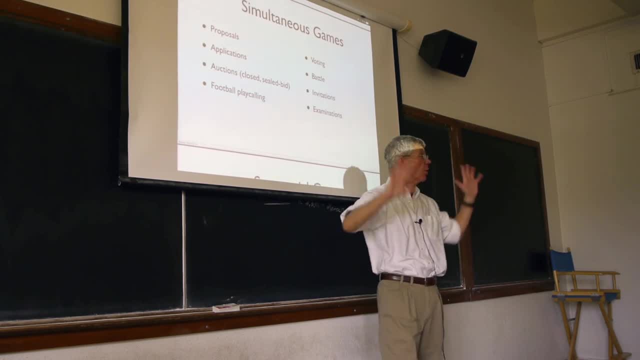 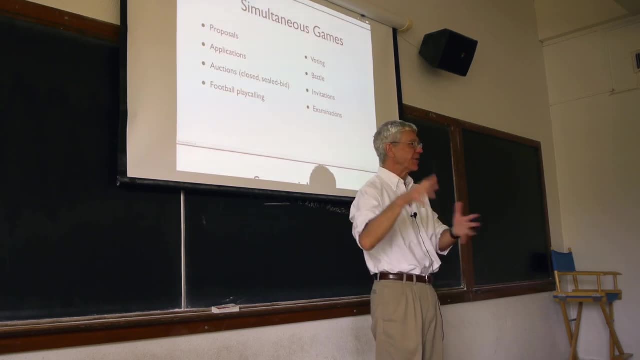 There are auctions where it has this form. Now, some auctions are open And it'll be like: ah, who will give me $50 for this small statue of Aristotle, et cetera. You bid and you know what other people are bidding, and so on. 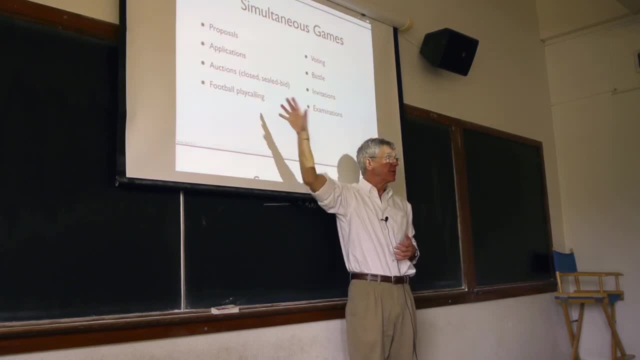 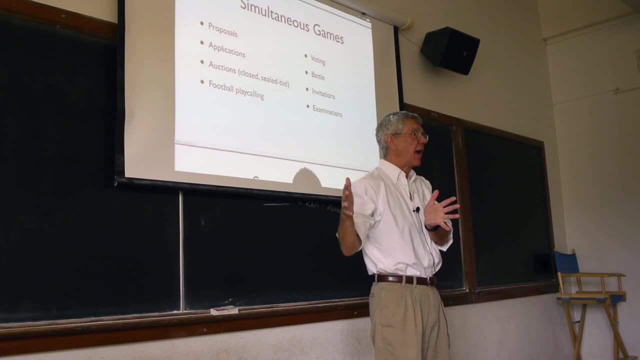 You can see their hands going up, But other auctions are closed and sealed. bid You just say, hey, here is a bid of property, Submit your bid And that's something where you don't know what the other people are bidding. Football play calling is like this. 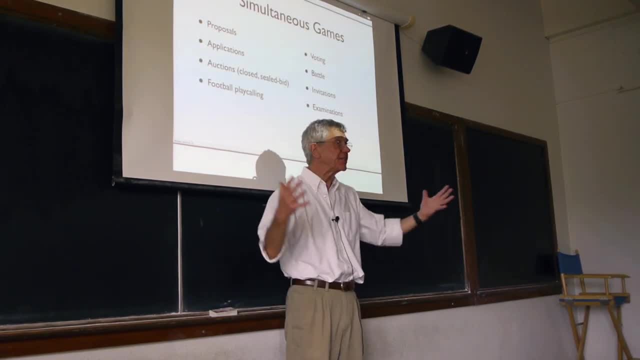 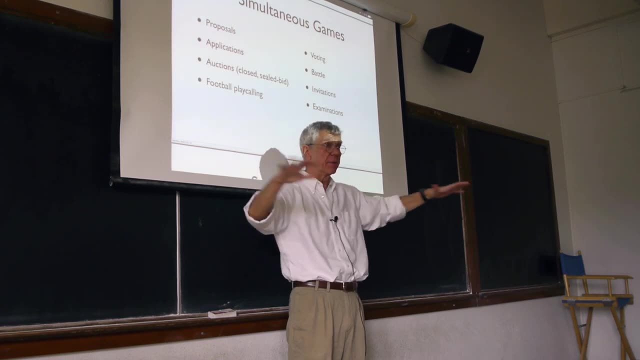 at least if you've got a decent team. The offense and the defense are there and deciding on the play. they're about to run separately And you might know the history of what people have been doing, But at the time the offense called. 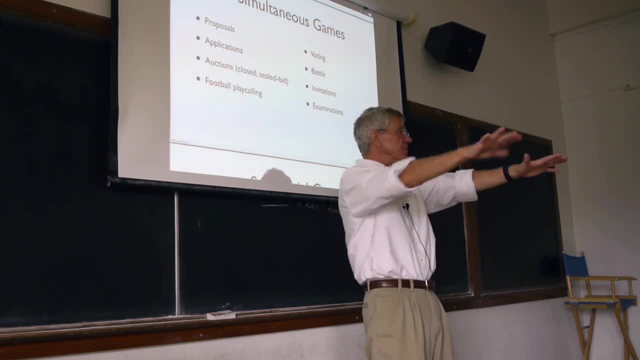 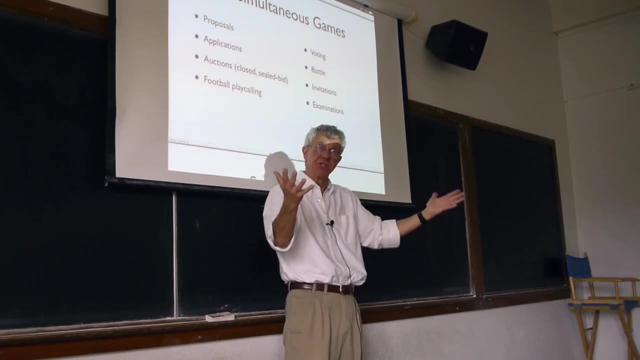 The defense calls its play in the huddle. They don't know what the defensive formation is going to be yet, And the defense doesn't know what the offense is called when they set up their formation. So you've got a situation where it's a simultaneous game. 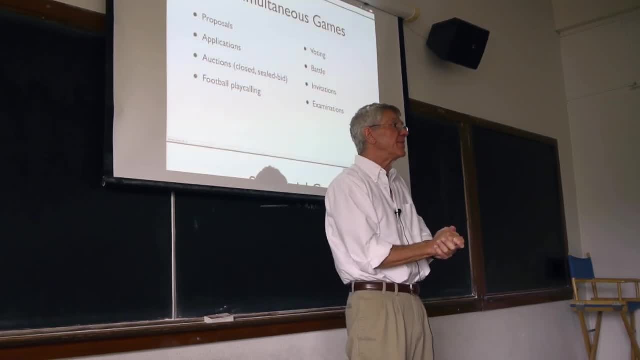 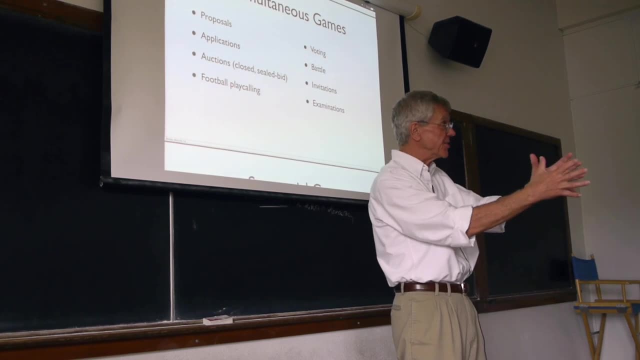 Yeah Well, the linebacker or the quarterback know what's audible, So that kind of makes it. That's true, That's sequential, That's true, They can audible. So the audible is a way of trying to turn this into a sequential game. 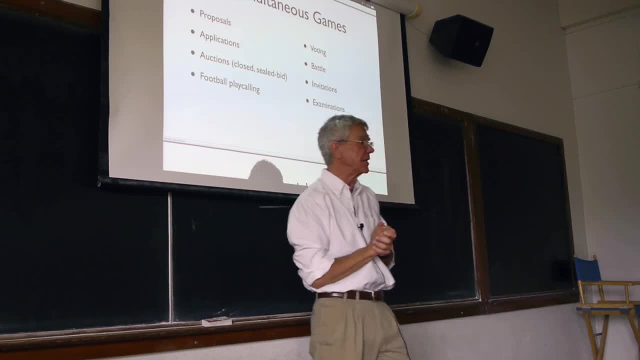 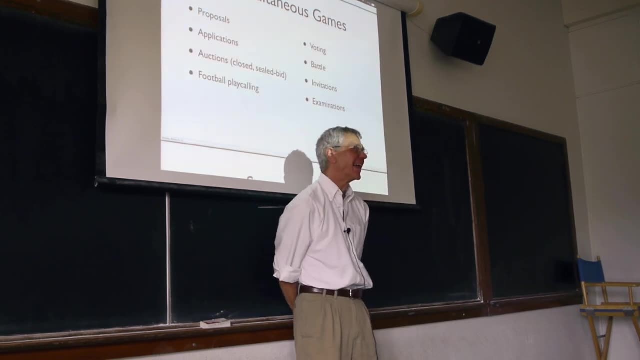 So I see where you are in the field. Now I do this Exactly, Or you could. I'm good. I'm sure some team from New England has done this at some point. You could video the other team to see what their play calls. 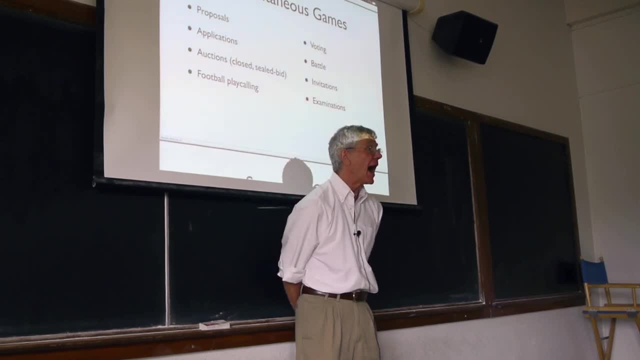 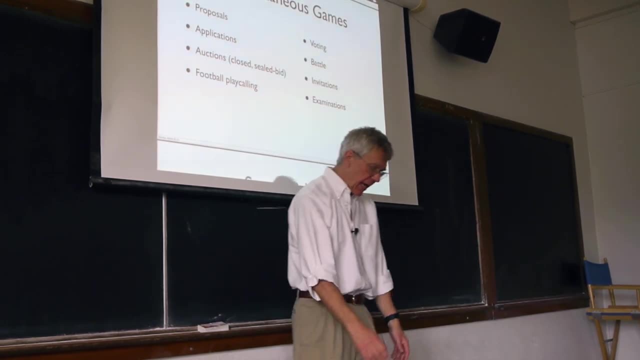 mean and then know ahead of time what they're going to do because of that. Ah, good, good, good, Yes, exactly So you should cheat. I mean normally in baseball, for example, it's a simultaneous game in the sense. 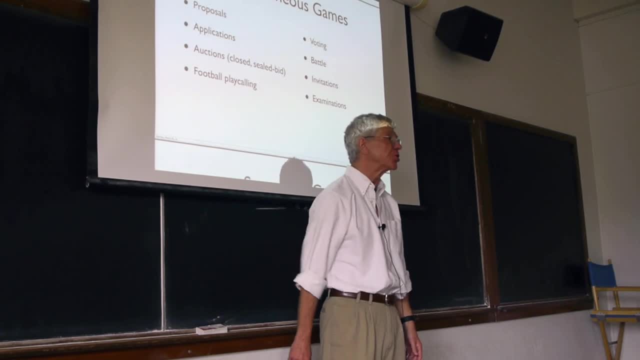 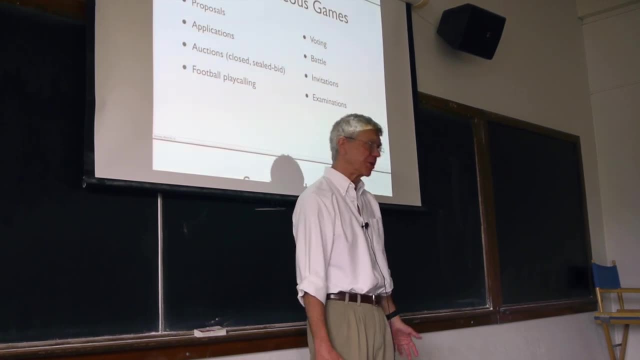 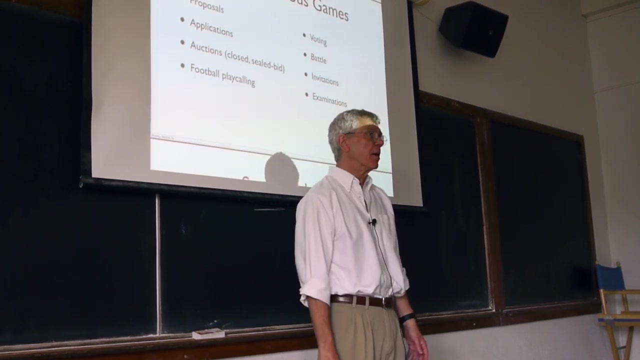 that the pitcher and catcher communicate about what pitch to throw And then the batter gets set and is expecting a certain kind of pitch. But this to a large extent has to decide on certain things before that pitch is even thrown. I mean, the batter can react to some things. 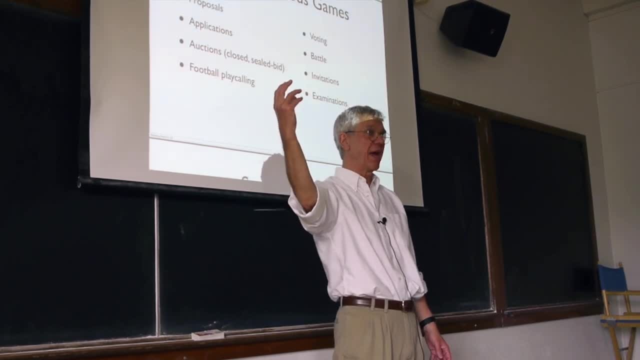 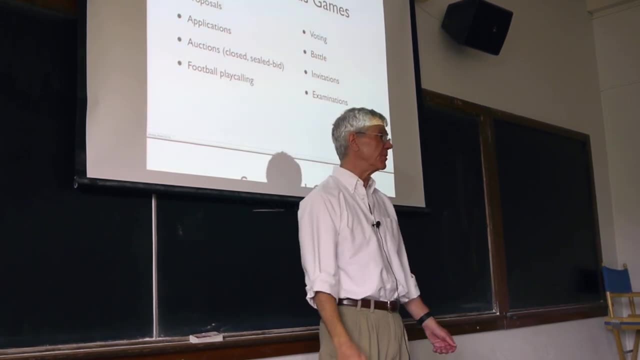 But how long is it? 60 feet 6 inches away? How quickly does that ball get to home plate? Often it's less than half a second, And so that's not much time to make a decision and move the batter around into any position. 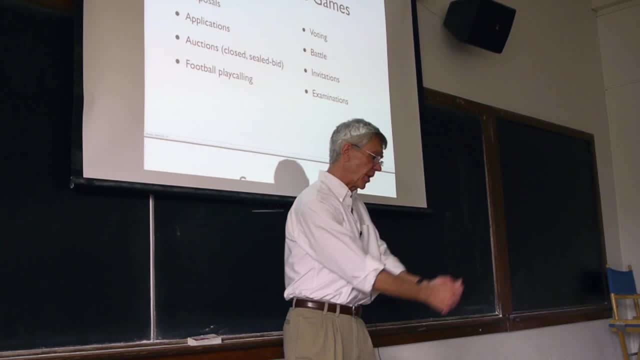 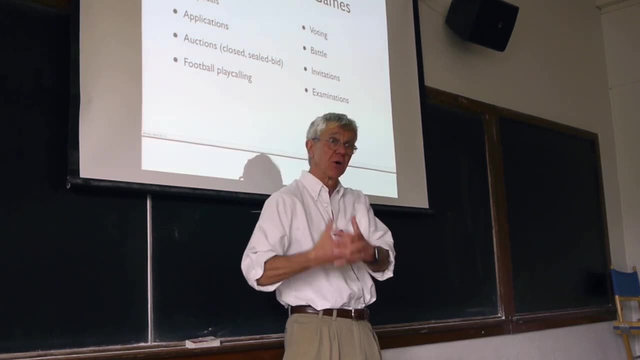 So to a large extent, the batter has to decide. am I going to try to swing at this or am I going to take this pitch Before they have any real information about whether it's a changeup, a curve, a fastball, et cetera. 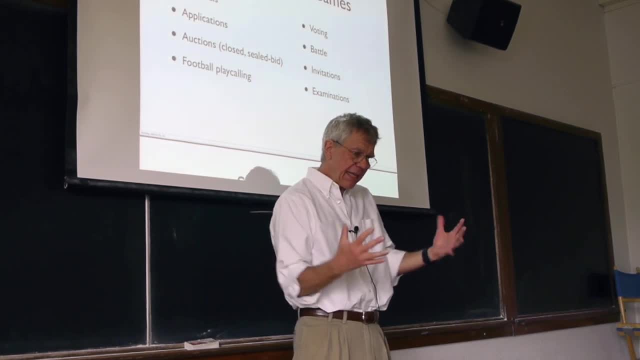 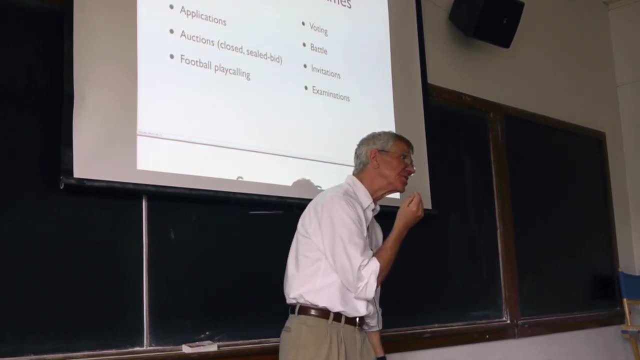 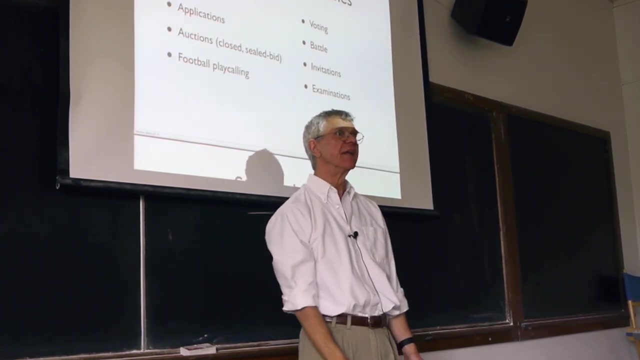 And that means it has the features of a simultaneous game. However, if you have somebody on second base and they manage to steal the catcher's sign, or let's say you have a camera back in center field and some teams have done this, then you say aha, curveball. 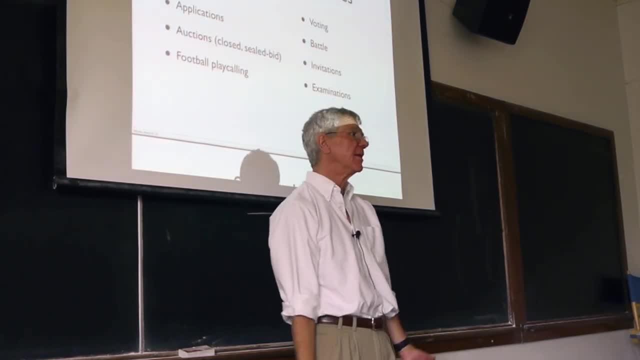 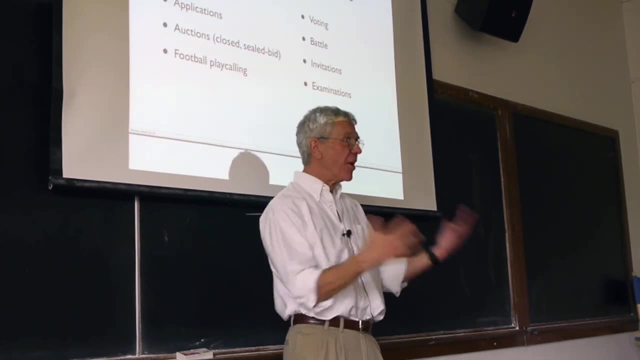 And if you have a way of signaling that to the batter, that can be a huge changeup, All right, That's a huge advantage, right? So watch those third base coaches. This sort of you know all that has a meaning. 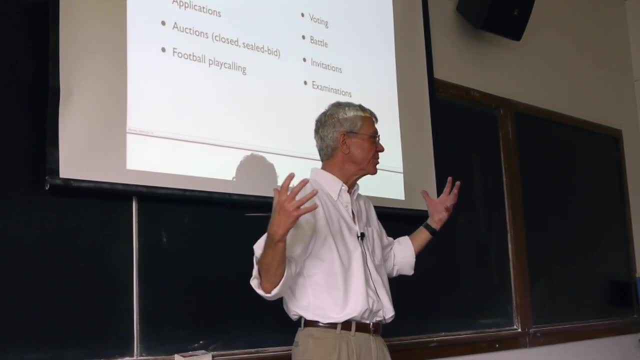 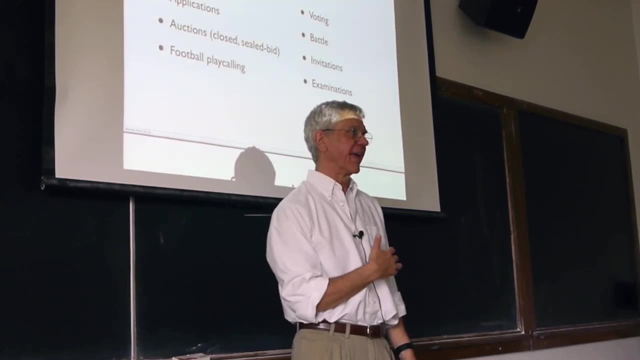 Well, some of it has a meaning. There's a lot of other garbage in there, so that you don't know what has a meaning or not. But some of that is going to be telling. the batter might be, take whatever, but it might be. 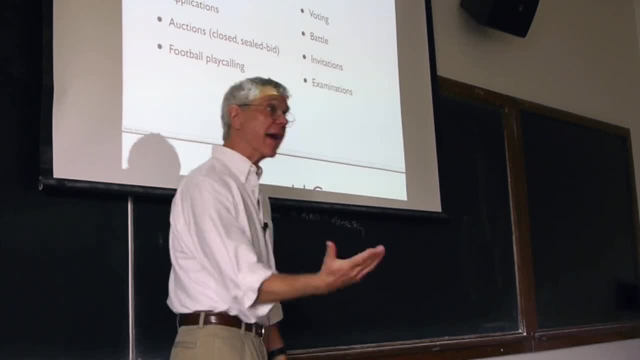 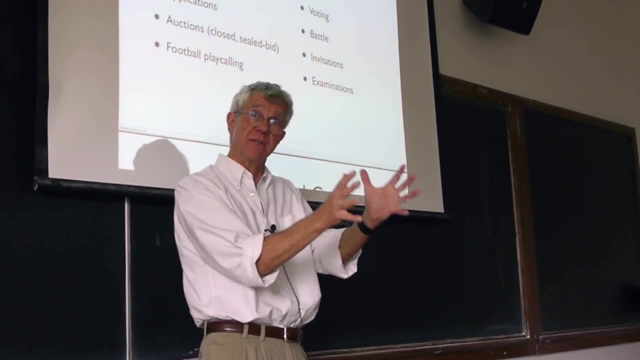 aha, curveball got me up, et cetera. So yeah, that's a way of. often it's to your advantage If you can turn the simultaneous play into a sequential one in that way by getting more information. very helpful. 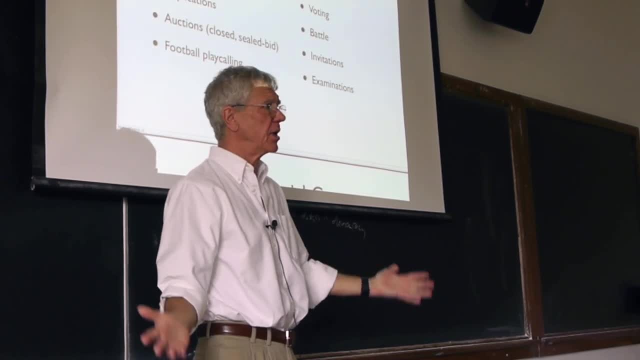 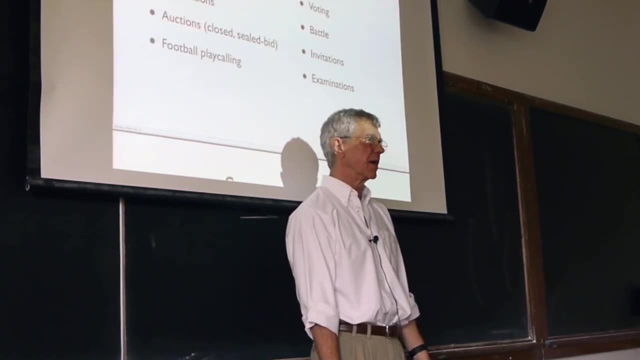 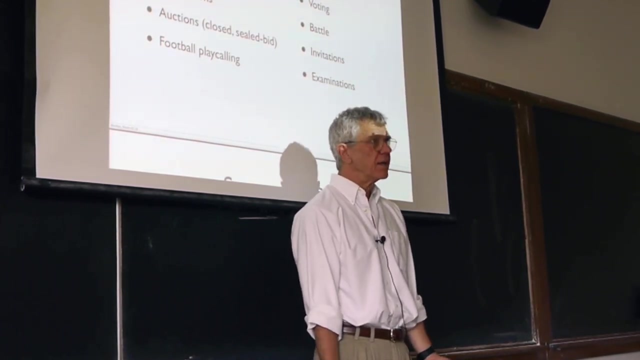 Of course. similarly, a team can give away information. There was a year- if you followed Texas football a few years ago- when it was the same thing every time: First down. oh, we're going to throw a screen pass. Second down. since that didn't work, we're going. 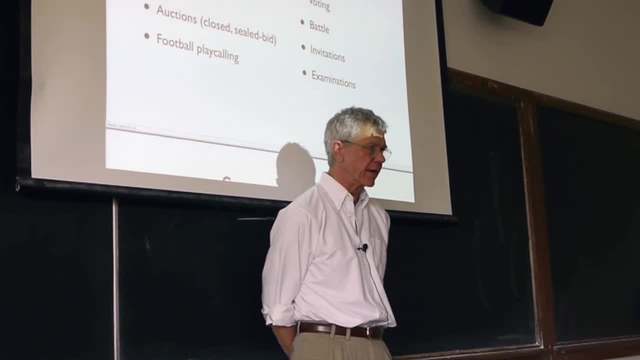 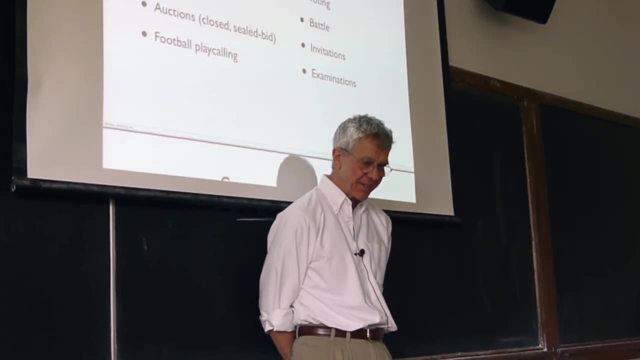 now it's second and long they expect us to pass, so we're going to run it up the middle, Then third down. well, now we've gone nowhere in two plays, So We'll just throw it randomly down the field. 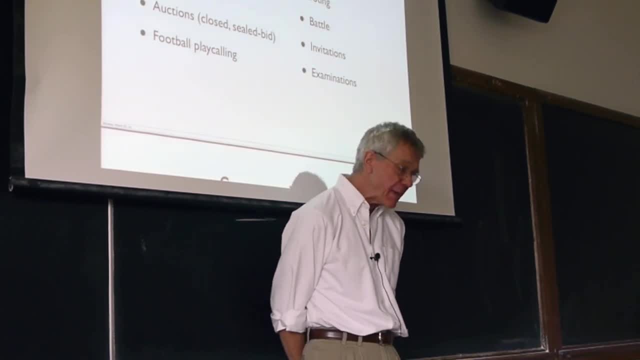 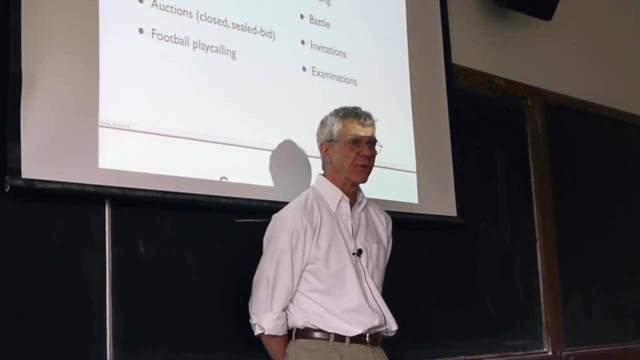 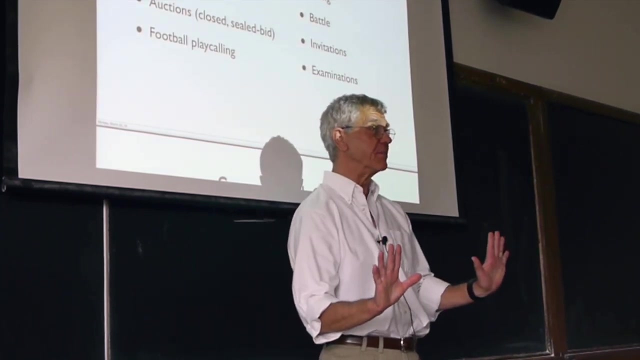 And that happened again and again and again. I mean people in the stands were calling the plays. You know it was like: ah, first and 10, OK, X screen. Yeah, that didn't work When you know the offensive coordinator's name. 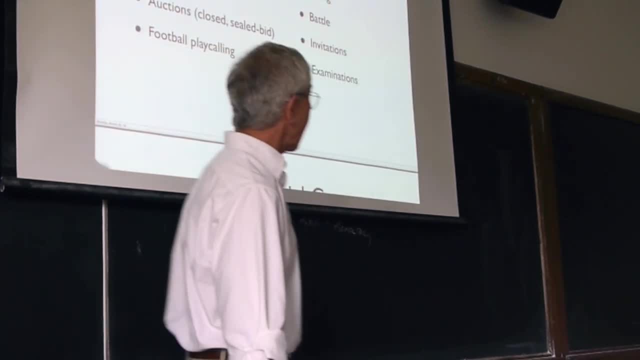 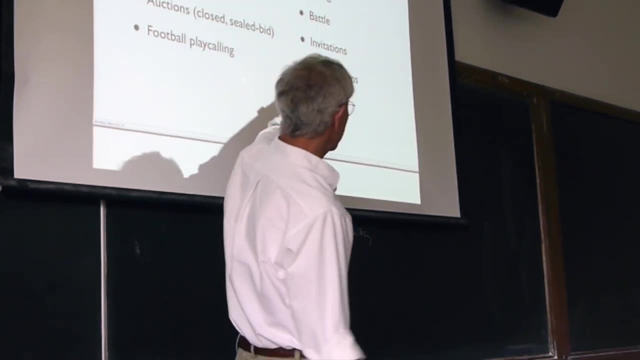 it's a bad sign. OK, People were so angry. In any event, voting is like this: You cast your vote. you don't know yet what other people are doing in the voting booth. A battle is often like this: You are formulating your battle plan in a way. 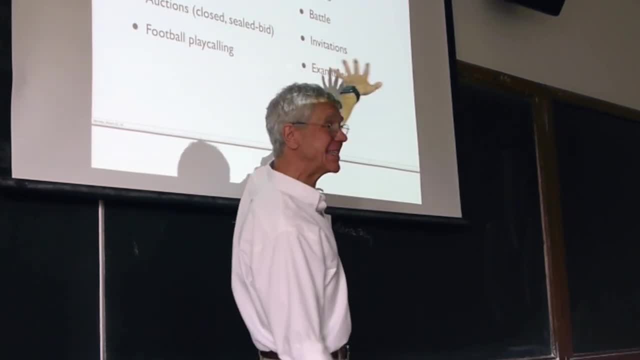 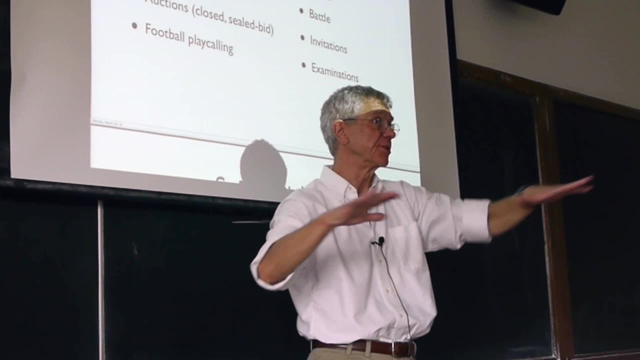 you don't know what the enemy commanders are planning. Invitations are like this: You invite people to the party at the same time and they might all have to respond to the invitations without knowing who else is accepting, and so forth. And exams, of course, are like this: 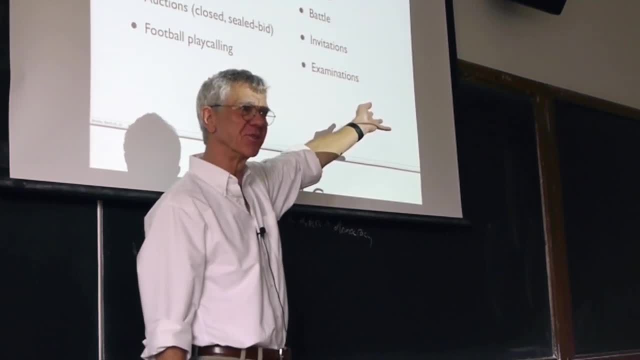 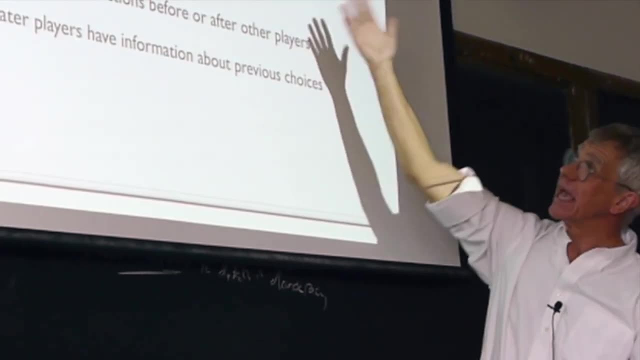 You put down your answer. You don't know- ideally you don't know- what other students are saying in response to that exam question. Of course you might, Anyway. OK, so in a sequential game you choose actions before or after the other players. 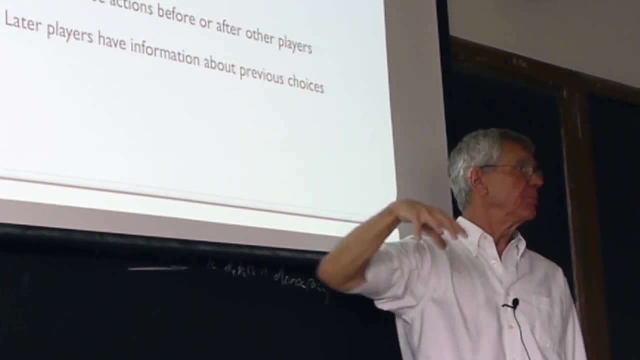 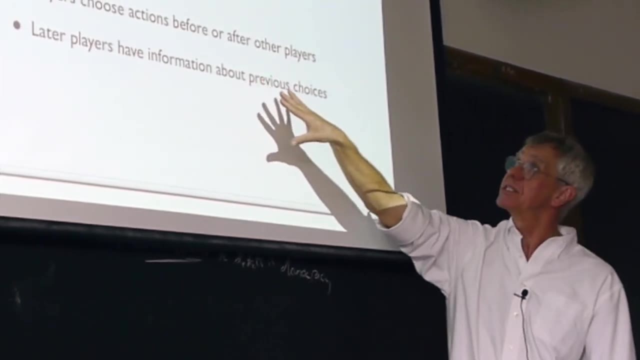 And lots of games are like this. I already mentioned chess. White moves, black sees what white has done and then responds: OK. Later players have information about previous choices And I move independently of you. You know what I've done when you respond. 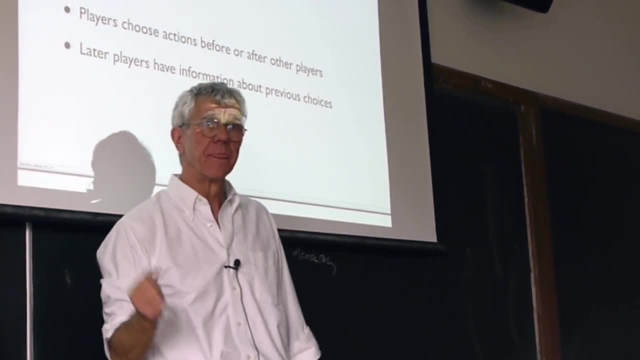 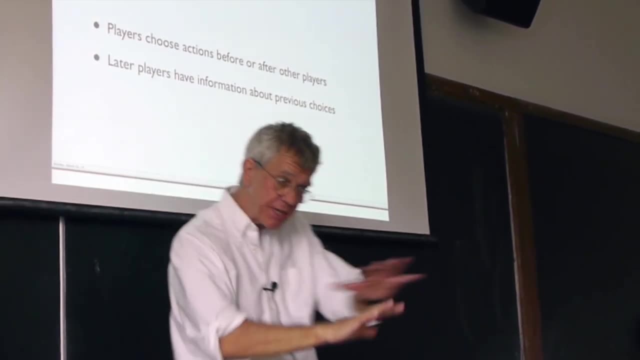 Quick examples of that in our last few seconds. Yeah, Offensive basketball. you can't see what the defense is doing anymore. That's right. In basketball, you get to see where the other players are as you're deciding where to go. It's not like you have to decide. OK, I'll do this. 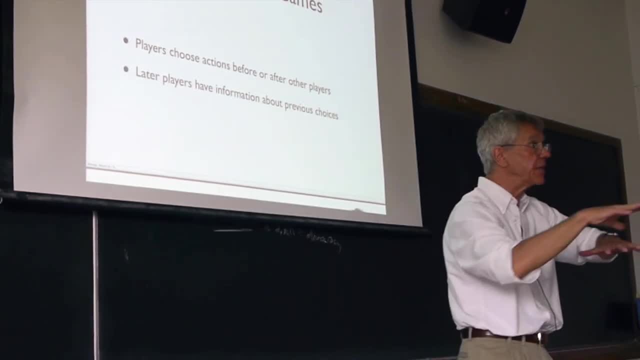 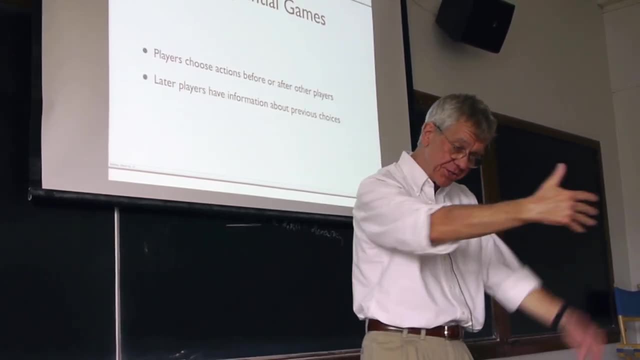 Without knowing what they're doing. you get to get constant information about what the defense is doing, Yeah, But where you can see how the other players are betting for his team, Ah good, Yes, you often can see what they've done as you go around the table. 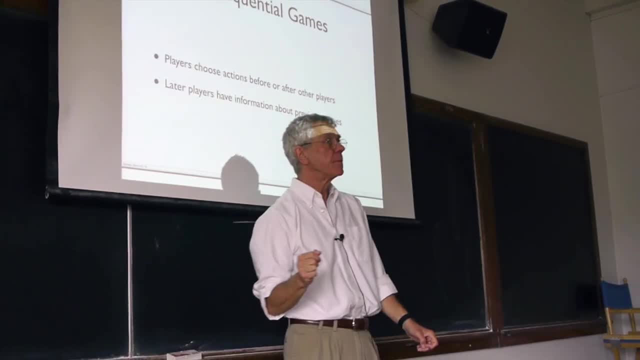 It's not like you all have to commit at the same time. Yeah, Negotiations. Negotiations can be like this: That's right, You propose something, Then you respond, et cetera, Et cetera, Et cetera. 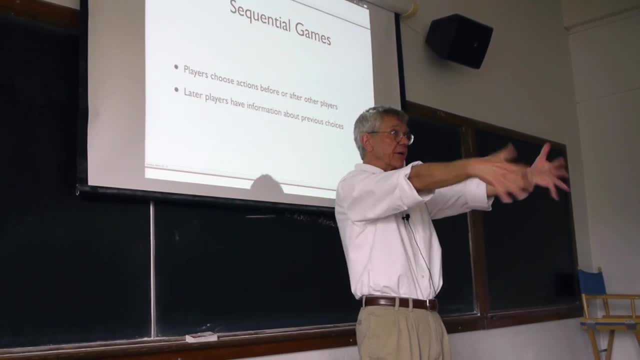 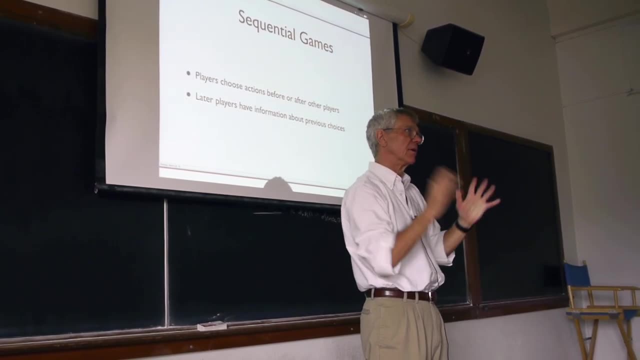 It's not like you both submit your things Now. if you're both going before an arbitrator, you may have to do it at the same time, But an ordinary negotiation isn't like that. Ah, I'll pay you $250,000 for the house.